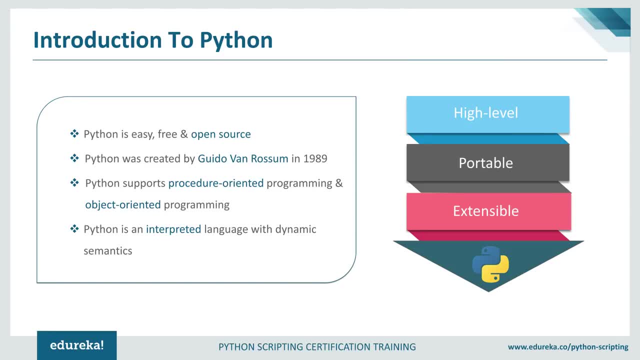 which is very famous. many big clients like Google, YouTube uses it, So it must be having some great features. So now let me just list a few of them. So, first of all, Python is easy, free and open source. The first reason lies here that it is extremely readable. 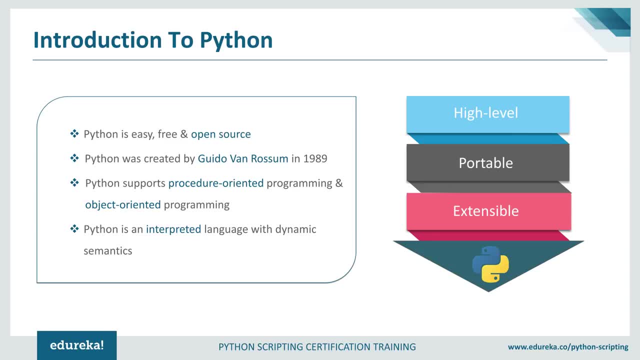 since it closely resembles your English language. Also, it was created by guru Van Ryssen in 1989 and was released first in 1991. next, it supports your procedure oriented as well object-oriented programming. I have already told you that it's an interpreted language. 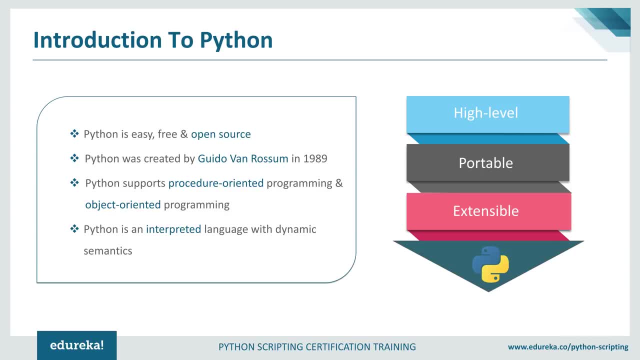 So it's also a high-level language where one does not need to bother about low-level details. You can simply write your code in English and Python will in turn convert into low-level details. Then, moving ahead, Python is portable as well as extensible. 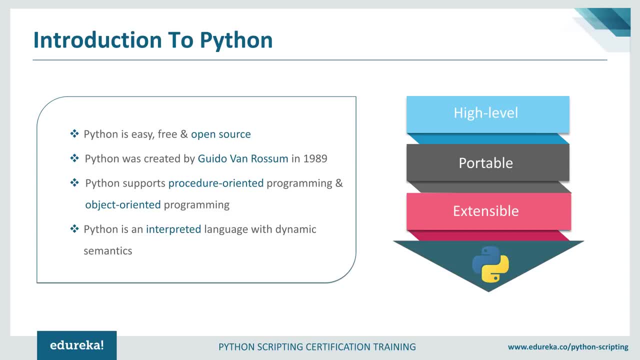 So by portability I mean it is fit for many platforms, be it Linux platform, be it Macintosh, be it Solaris or any other, then it is extensible. So by extensibility of Python I mean you can completely integrate Java as well as NET components with it. 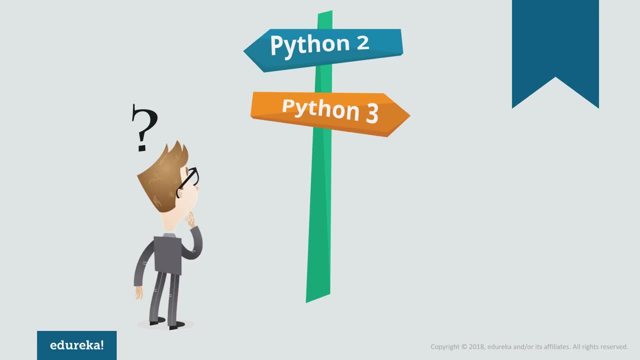 Isn't this great guys? You can do a lot of things with Python. next, Let us move ahead and talk about the popular versions of Python. So there are a lot of confusion between Python 2 and Python 3.. So let me first clear this confusion. 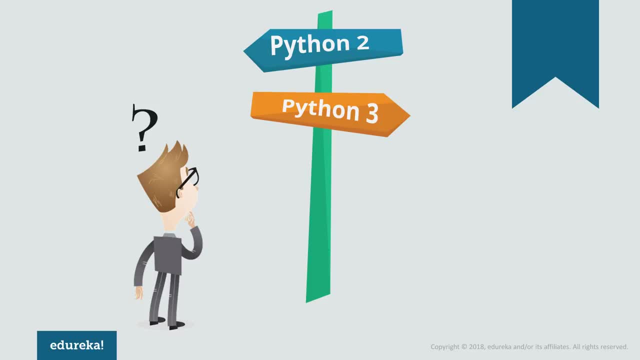 and then we'll move ahead with the practical demo. So if you're learning new, just jump into Python 3, because it has come up with some neat and clean features and also it is the present and the future of the programming language. But if you're already learning Python 2 or 2.7. 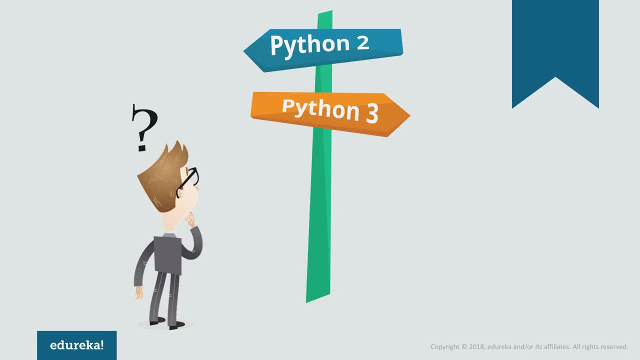 or any version of 2x family. don't worry guys, Python 2 is not so different in terms of your core language. There are just a few differences here and there, and if you learn to code in Python 2, it will hardly take your some time to learn the differences. 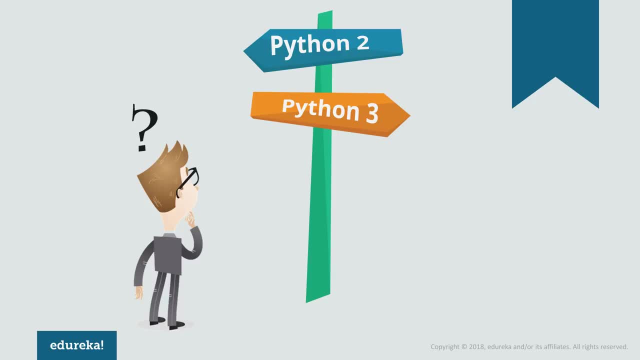 and the syntax. So we all know that Python 2 is used for many years. many organizations make use of version 2 or 2.7, which contains a large number of libraries with a wonderful support community. But again with the release of Python 3, many libraries. 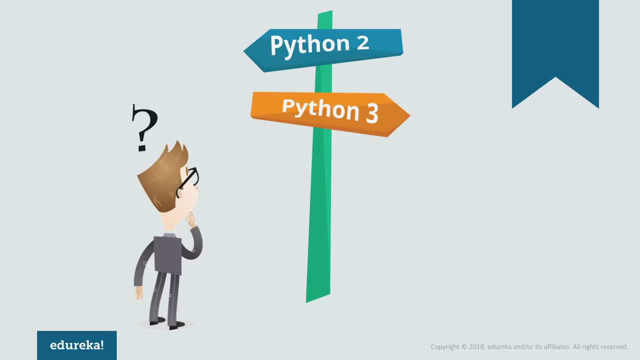 require support of the latest version. So let's say, if you are doing web development and using a lot of libraries, then you must go for Python 3.. Also, Python 3 has recently gained a lot of attention from the developers. There is a lot of additional features, such 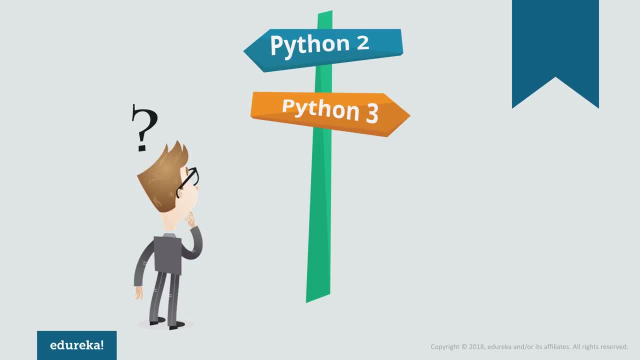 as your overall performance has been increased. Then you have a better interpreter history. Also, there are auto-completion features and you have many more like that. It has also picked some of the minor glitches from the older version and released Python 3, which is more stronger. 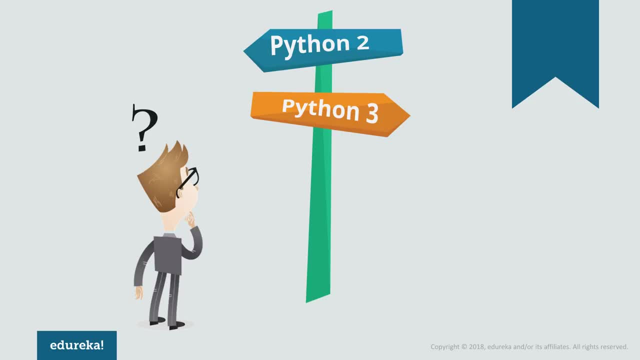 So it is faster and quite a stable version till now. So, as I already told you guys, Python 2 is a legacy, whereas Python 3 is the present and the future of the programming language. So you can learn either version of Python, which you can later tailor according to your needs. 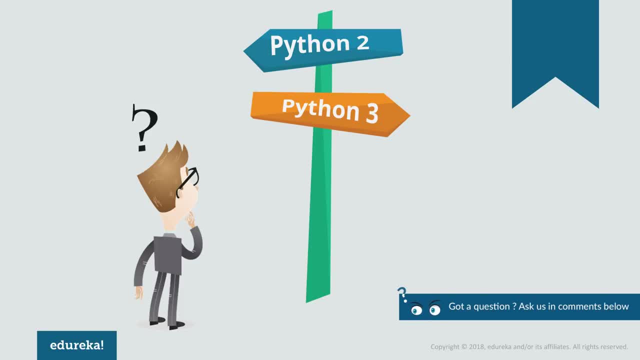 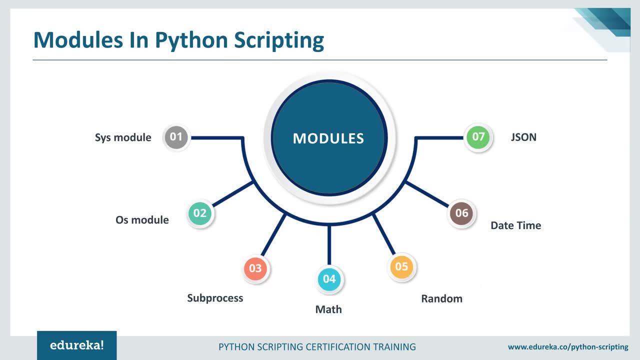 Even if you start learning from Python 2.7, it will be a no big deal to ship to the latest version as far as your focus remains to learn Python. So I guess, enough of theory part. next Let us discuss the various modules in Python. 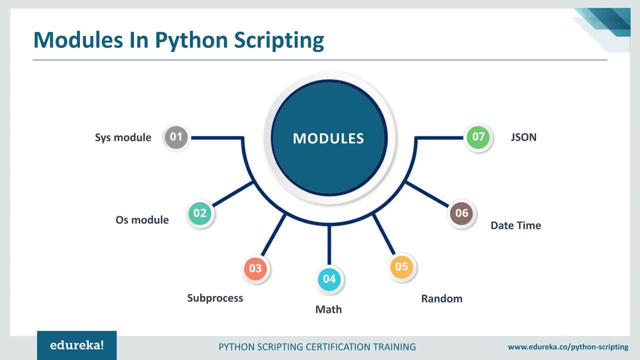 So a module in Python is basically a file which contains Python definitions and statements. Now, as you can see, here I will be talking about these modules, So it is majorly classified into sys module, then OS modules, subprocess math, random datetime module and the JSON module. 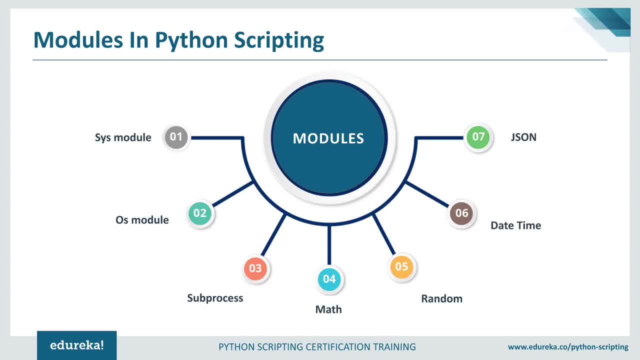 So let me begin with the very first module, that is, the sys module. So now, sys module basically provides you the information about the constants, functions and the methods of Python interpreter. So it is basically responsible for controlling and interacting with the interpreter. now, for example, 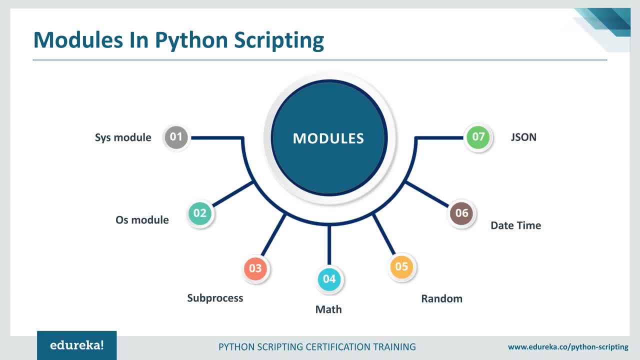 if you want to know any information on operating system or the version of Python you are using, you will be using the sys module for that. So first let us import sys using the import statement. So it means practically show you how this can be done. 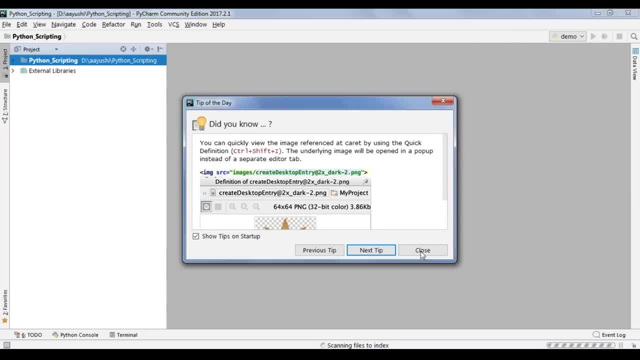 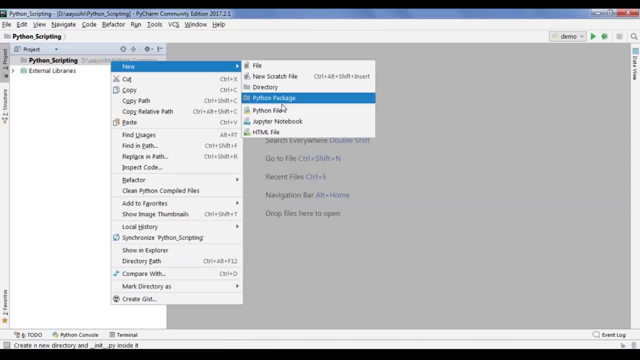 So it may just open my IDE, that is pycharm. All right, so I am in my pycharm Community Edition project named as Python scripting. So now inside this project I will be creating a Python file. Let's say I'll name this as sys module. 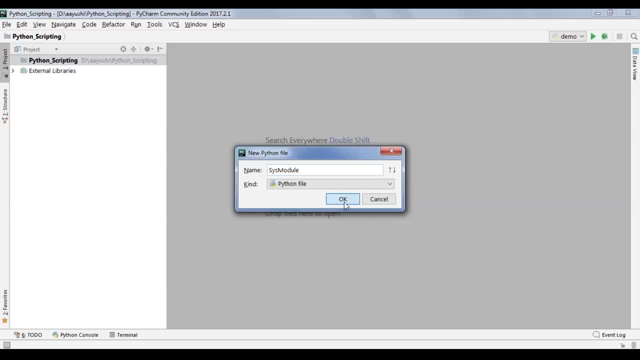 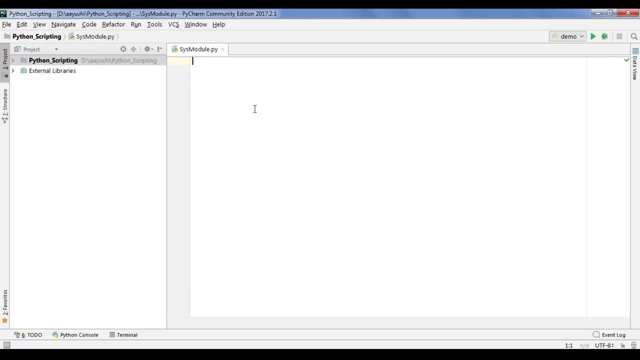 So now the first thing that I need to do is to import this module. So all you have to do is to just type in import sys. Now let's go ahead and print the version. Let's say: I want to know the current version of Python. 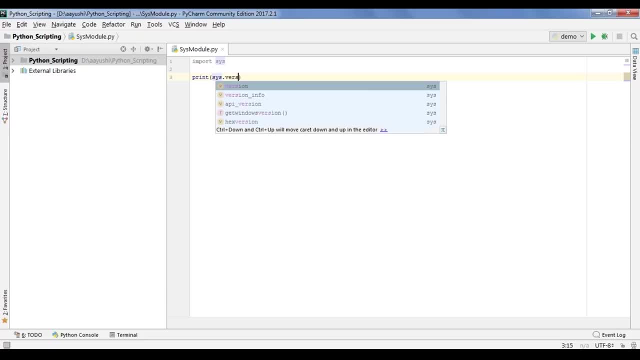 So what I'll do? I type in print sys dot version and let me just run it. So, as you can see here, the current version of Python that I am using is python 3.6.1.. So let me just zoom this a bit. 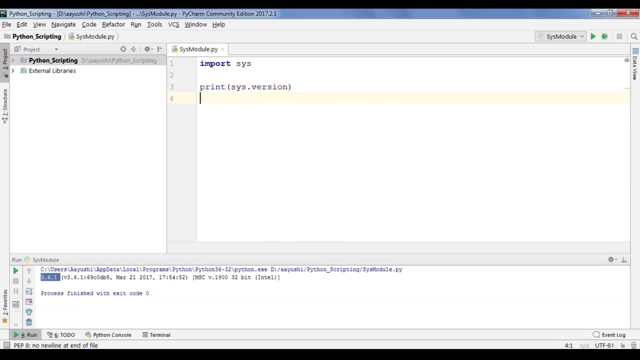 All right. next, if I have to print the command line arguments which is passed to the script. So what I can do, I can simply type in, let's say, print sys dot a RGV. So basically, a RGV is a list which contains the command line arguments passed to a script. 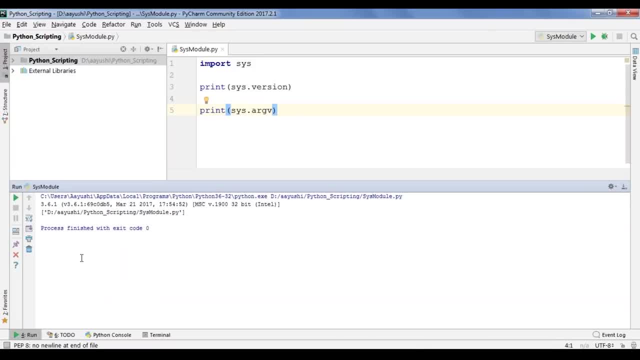 So let me just run this again. So, as you can see, here we are in this location, which is in the drive, in a Yoshi folder. Then I have a project name followed by the file That I've just created. So, as you can see, here, argument follows the script name. 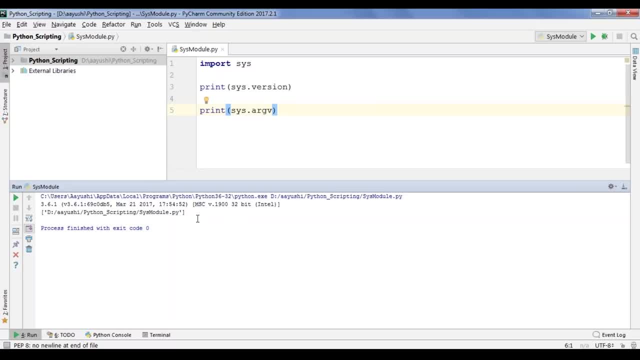 So, whatever argument we have currently, we don't have it right now, but whatever we have it, it will follow the script name. Now, similarly, we have a lot of functions. We have stderr, which basically stores your error messages. Then we have stdin, stdout, which is used to accept the input. 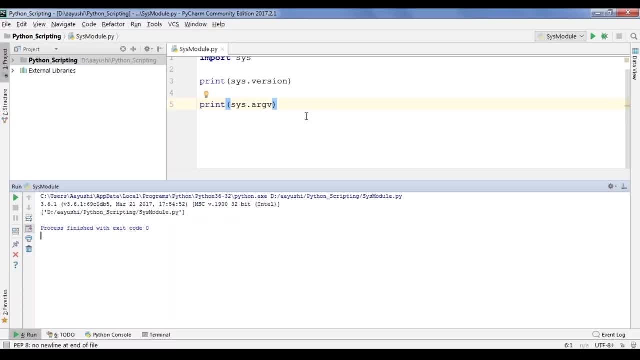 from the user, whereas your stdout method prints it to the screen. then you have an exit function which basically tells your interpreter to quit, or you can say it's a direct way to end a python script. next, Let me go back to the presentation and let's see what is my next module. 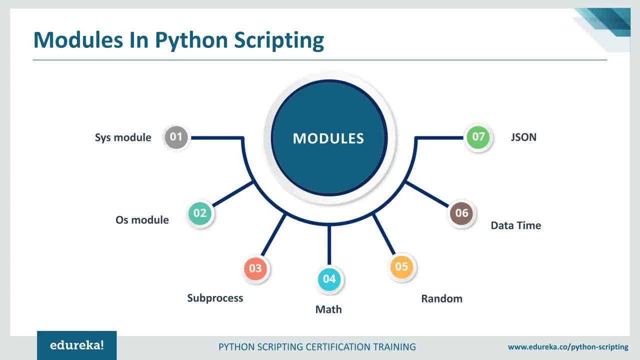 So next is my OS module, which stands for operating system. So it must be pretty clear that this module is used to interact to my operating system. Also, the primary use of this module is to create folders, remove folders, move your folders or sometimes change your working directory as well. 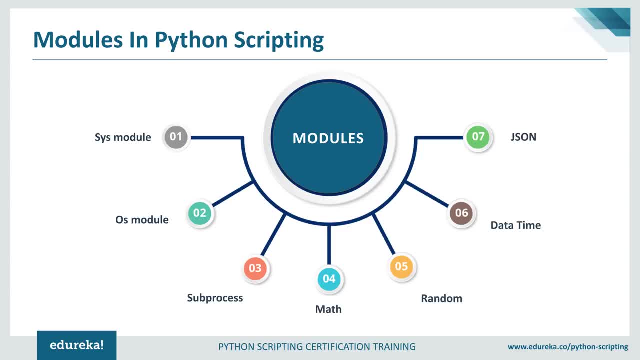 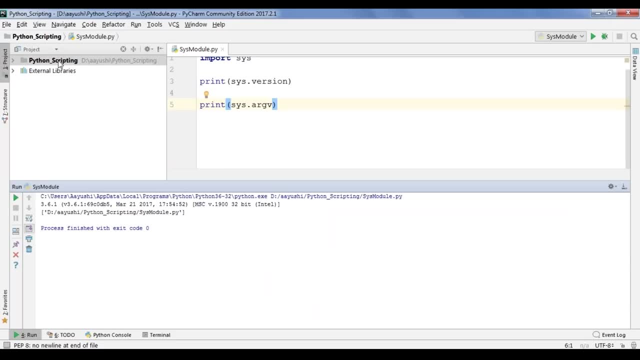 So you can also access the names of your file path by just typing in list: dir. Let me just show you some of the operations with this OS module. Go back to my pycharm. Let me create one more file here and I'll name it as OS module. 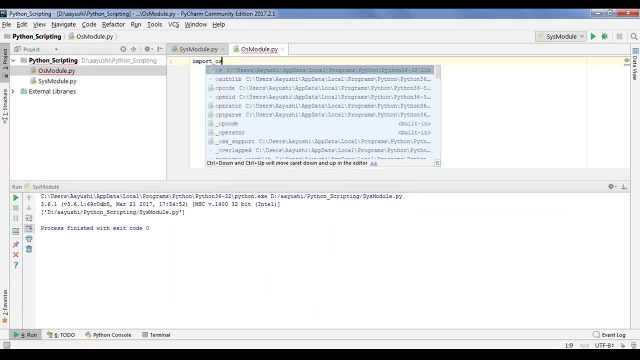 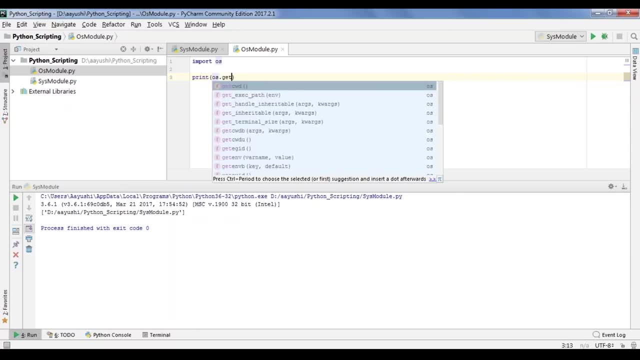 So now, first of all, I have to import the module, So I type in: import OS. now let us first print the current working directory. So I'll type in: print OS dot. get current working directory. That is CWD. and let me just run this now. as you can see here, 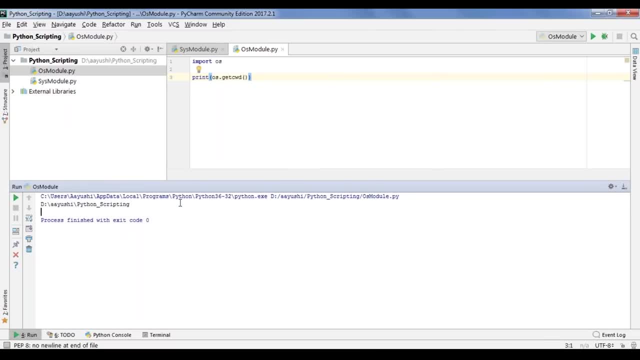 that my current working directory has been printed. now you can also change this directory. So for that, what you need to do, you just need to type in CH dir and just give the path. So let me just do that as well. So I'll type in OS dot CH dir. that is for chain directory. 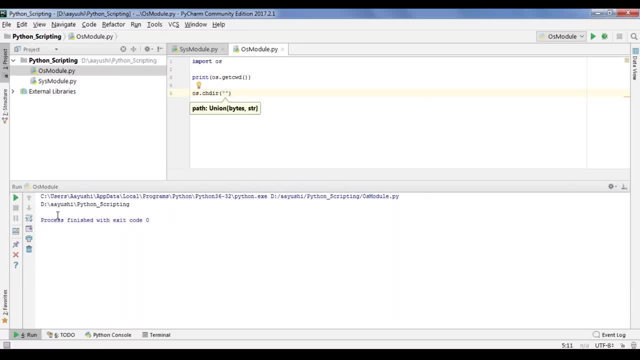 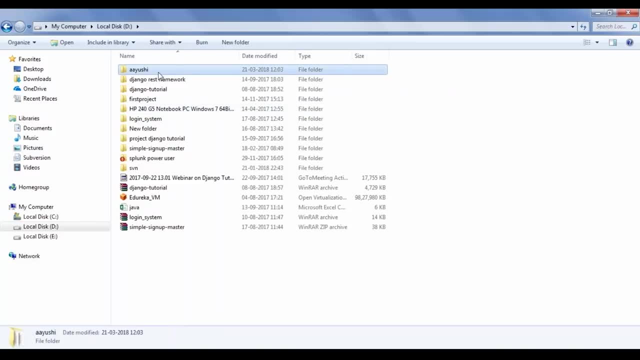 and inside this I'll be giving a path. So let's say I want to go in this type to only di. you see Python scripting, So I'll go to my files. So let's say I am in my D Drive and inside I use a folder. 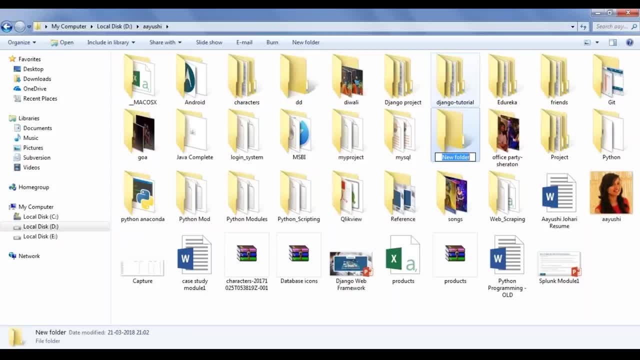 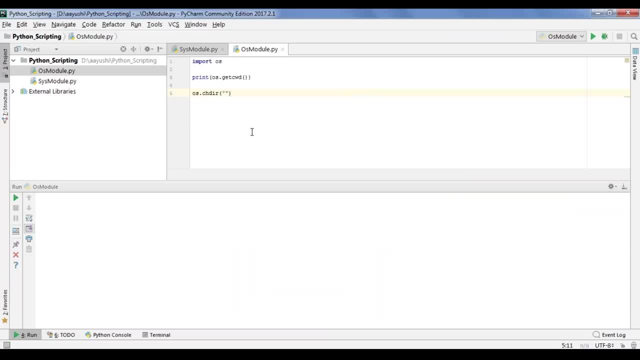 I am creating a new folder over here. Let's say you let the name be new folder only and I'll just go inside this and I'll copy the path from here. Now I'll go back to my pie charm again and then paste the path over here. 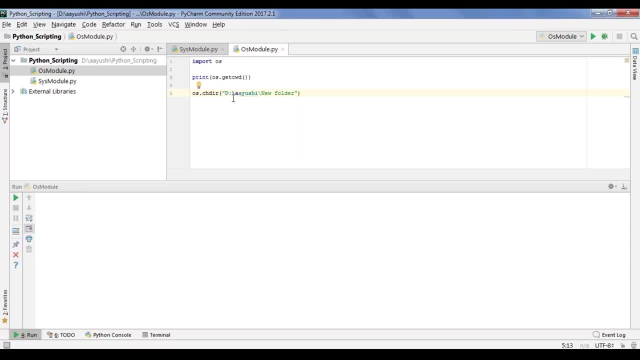 So remember, guys, whenever you copy or paste the path, you have to be careful for the slashes. You have to keep in mind that either double backslash will work or a single front slash will work. So I'll just type in here: double backslash. 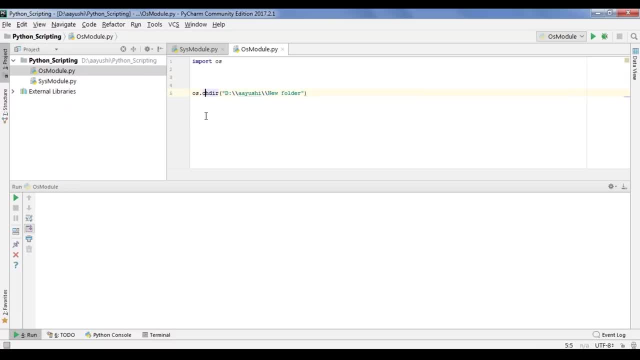 and I just print my current working directory. So I'll just cut it from here and I just paste it below that. and now let me just run this. So, as you can see, guys, my current working directory has been changed to new folder. So this new folder is we have just created. 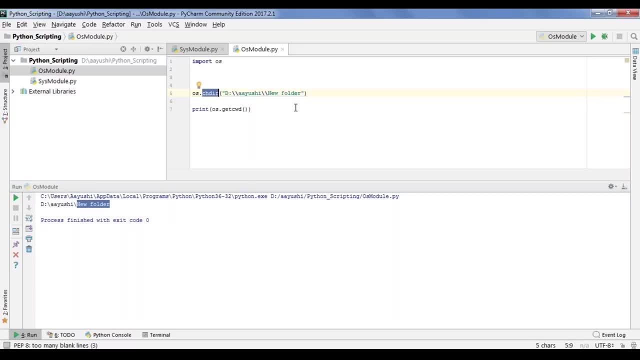 and using the command CH dir. I have just changed my path. So we have talked how to create a different directory all together. But what if you need a directory in an existing directory? So yes, you can go ahead and create a directory as well. 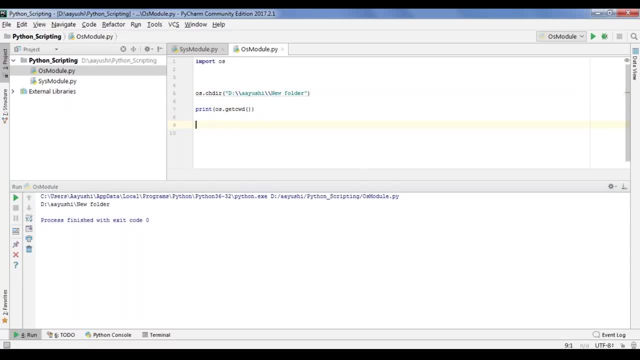 for that. What do you need to do? You just need to type in OS dot mkdir. So let me just type in OS dot mkdir, that make directory and I can write the path over here. So let me just take this path only, and in spite of new folder. 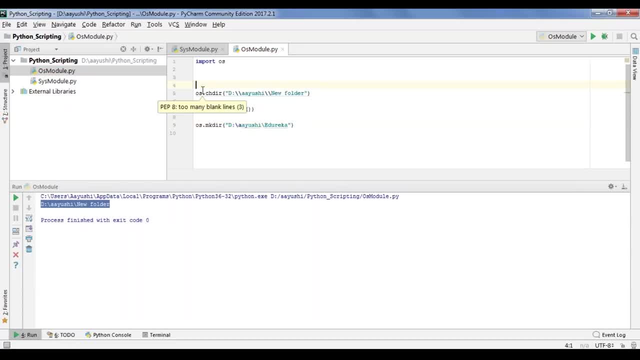 I want to folder named as edureka and let me just comment the above sections. All right, So, as you can see here, we don't have a directory named as edureka, So now let me just run this. All right, So remember, guys, a double backslash. 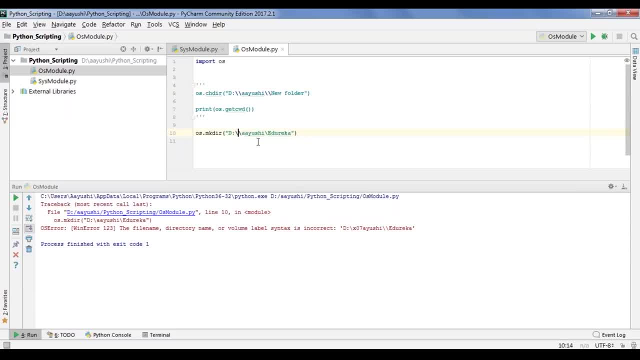 or a single front slash will only work, So I'll just change this to double backslash. and now I'll just run this. All right, So here it says that in the name already exists, So let me just type in edureka1. and now, if I just run this, 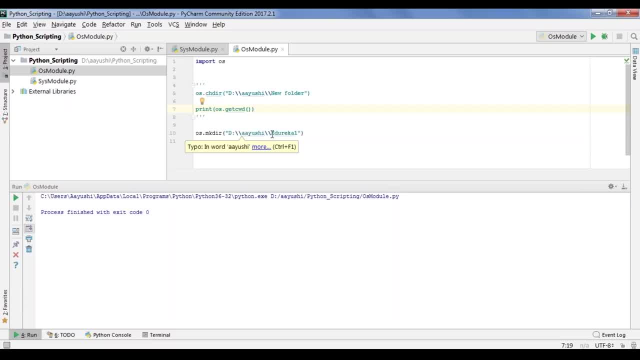 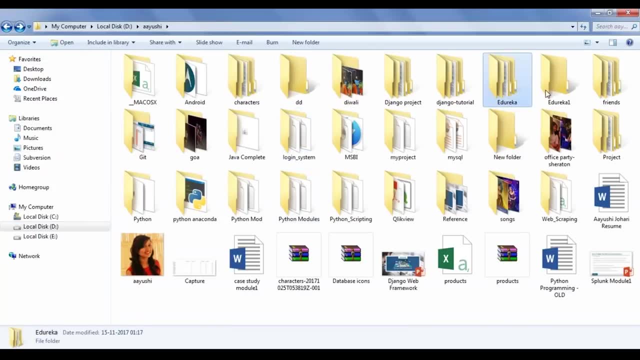 So here you can see, inside my D folder, then in I use a folder. I have one folder named as edureka1.. So let me just go to my folder and here it must be edureka1.. So, as you can see here I have a folder named as edureka1. 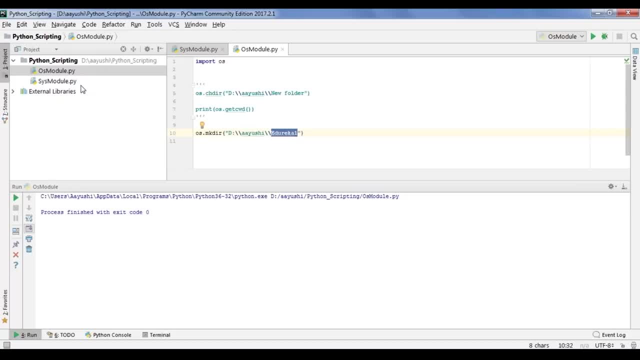 So if you don't want to do it over here, you can directly do it in your PyCharm also. So for that let me just copy this path. This is my present directory, So I'll just copy my path And over here I'll be pasting in this path. 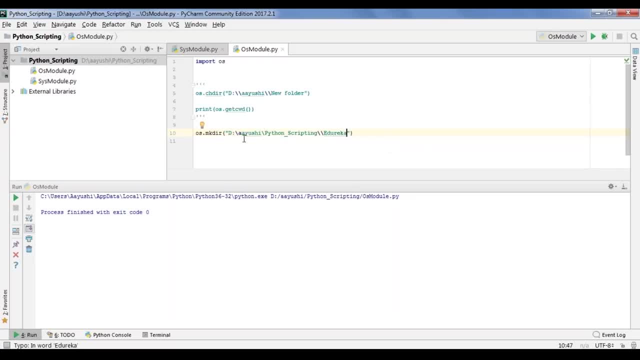 So now this folder, or you can just write edureka1 and I'll just type in double backslash and if I run this code you will see the edureka1 directory here. So now let me just run this code. So if you run this code, 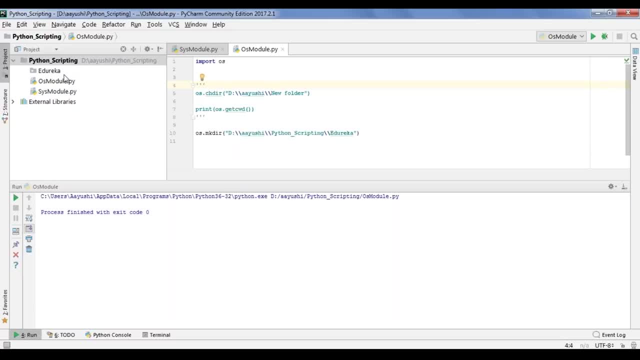 you will see that edureka1 folder, or you can see the directory has been created over here. Now you can also remove this directory by just right-clicking it and delete it, But now if you want to do it by codes, So for that what you can do. 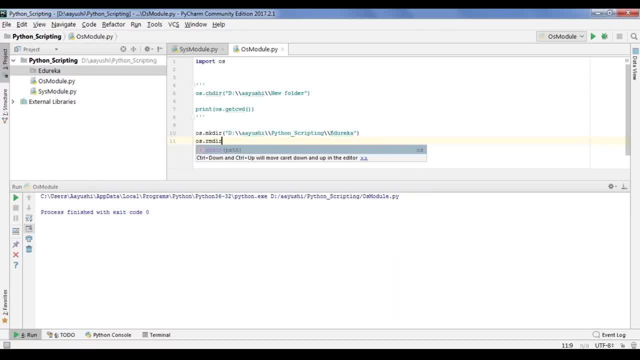 you can simply type in OS dot, remove directory, that is, RM, dir, and then you can just mention the path. So I'll just copy the path. So now I don't need this edureka1 directory over here, So I'll just paste it over here. 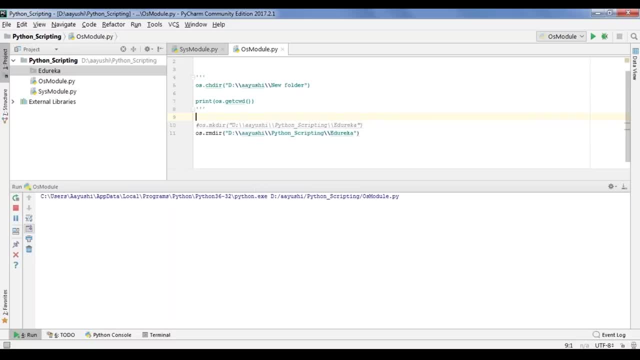 I'll just come in this line and now let me just run it. So, as you can see, edureka1 directory, which is present over here, has been deleted. next, Similarly, you can delete a file as well. So let's say, I don't want to delete a directory. 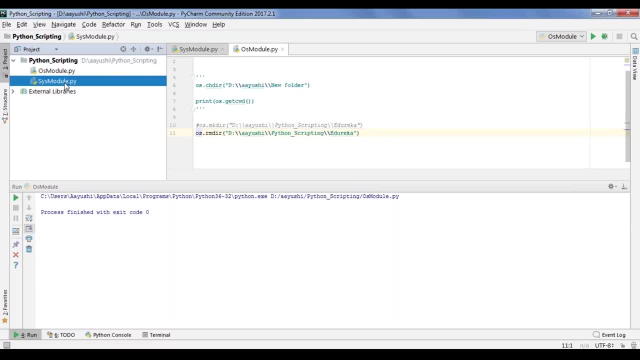 instead of that, I want to delete one file. So let me just delete this module. So let me just copy the path from here. and to remove a file, I just need to type in OS, dot remove, and I just paste the path over here. 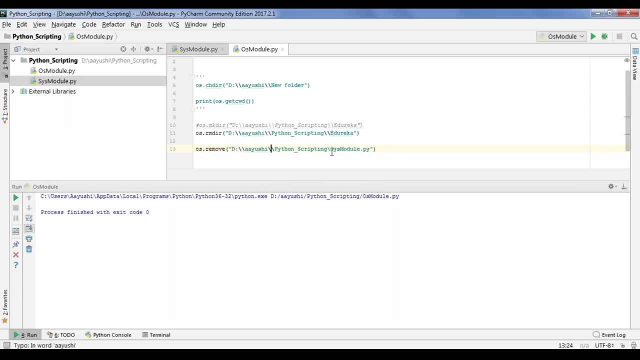 Remember, guys, to put the double backslash or a single front flash. So I just put it double backslash. I'll just comment the buff line and I'll just run this. So, as you can see, sis module, which is present over here, has been deleted. now next, 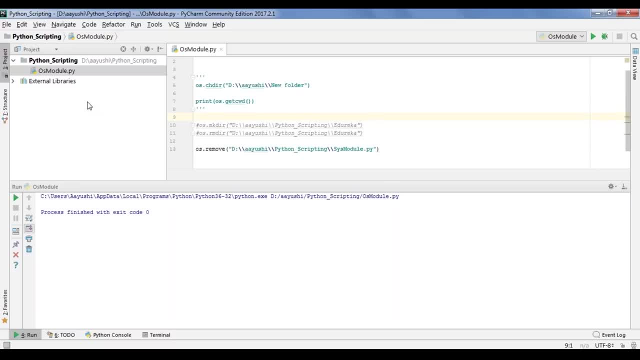 You can also learn about another sub module of OS, which is OS dot path. So it provides a range of useful methods to manipulate the files and directories. So it may implement some of the methods of this also. So first let us talk about join. 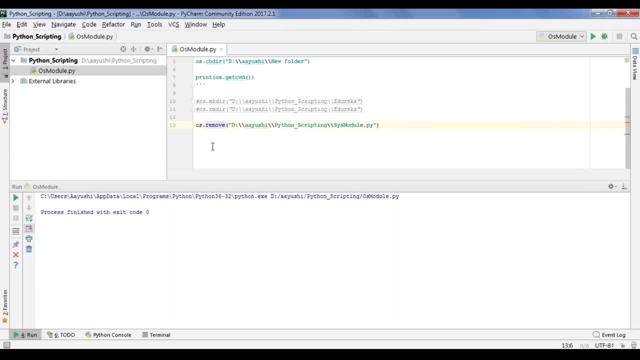 So OS dot path join is one of the important OS part tools. So it takes one or more parts and joins them by using the current OS part separator, So to join two parts. So let me just comment this. So now I need to perform the join operation. 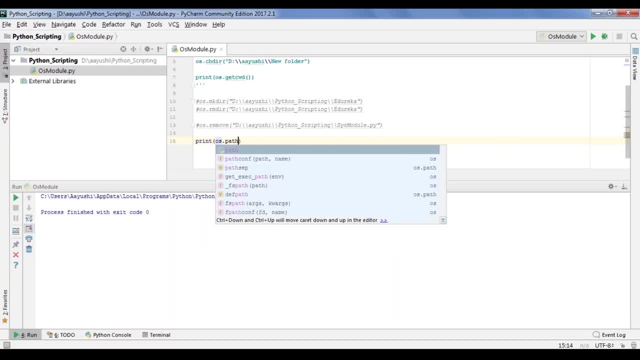 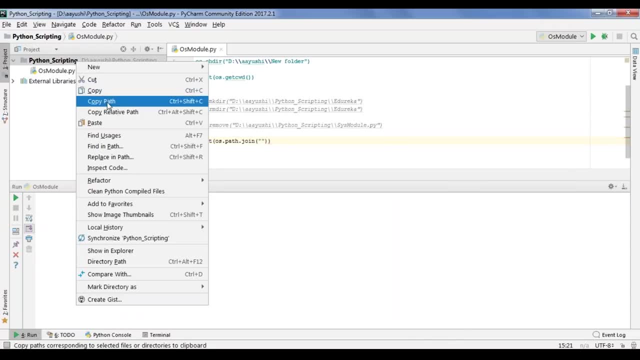 So I'll just simply type in OS, dot, path, dot join, and inside this I'll be writing two parts. So first of all, what I'll do? I'll just simply copy my directory path. So I'll take it from here, I'll paste it over here. 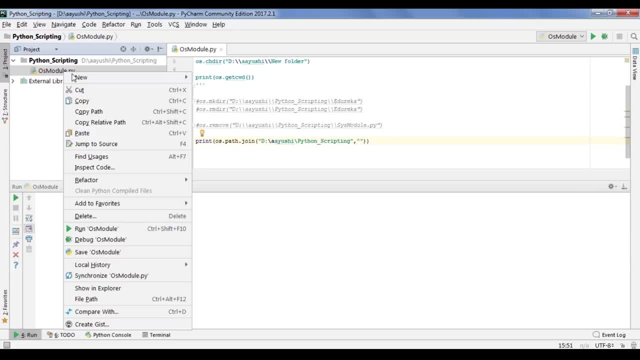 Then I'll be writing another part. Let's say I want to join the OS module, So I'll just copy the path, I'll type it over here and add the double backslash. All right, So now let me just run this. 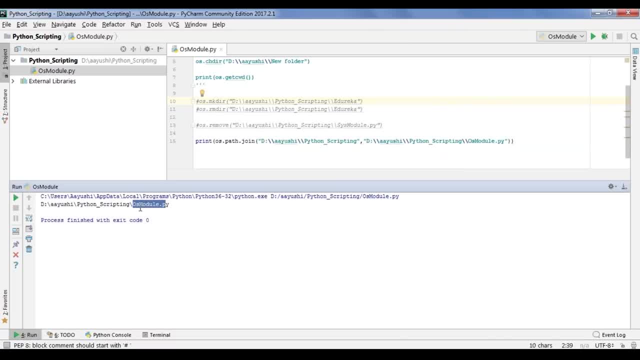 So, as you can see here, my OS module has been joined with the Python scripting. So next you can also split these parts. So basically split function. It takes a path name and returns it into the two parts, That is, the directory part and the file name. 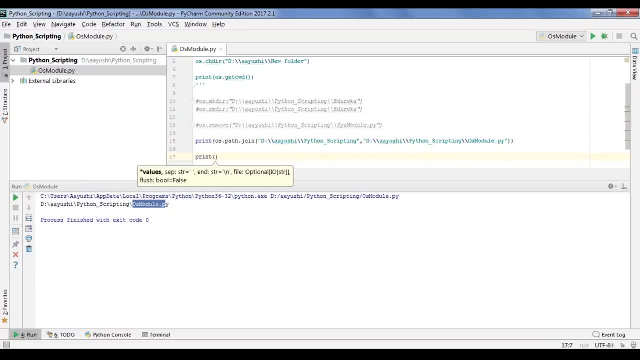 So for that, what you can do, you can type in print and say OS dot path. I'll paste the path. So let me just copy this path, All right, and I'll just comment this. Let me just now run them. So, as you can see, it has split it into two parts. first, 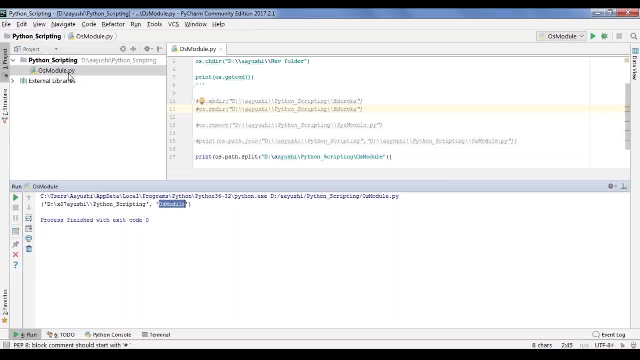 is the directory and second is the Python file that is present over here. So that is how you can use another function that is split. next, You can also use another function that is exists. So this will basically tell that whether the path exists or not, so it will return you a true or a false value. 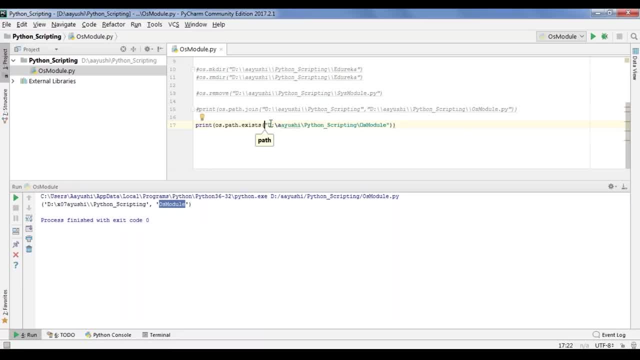 So I just type in over here: exists and I need to mention a path. So in spite of this, let's say I want the OS module path. So I'll just copy the path and paste over here, I'll add the double backslash and I'll just run this. 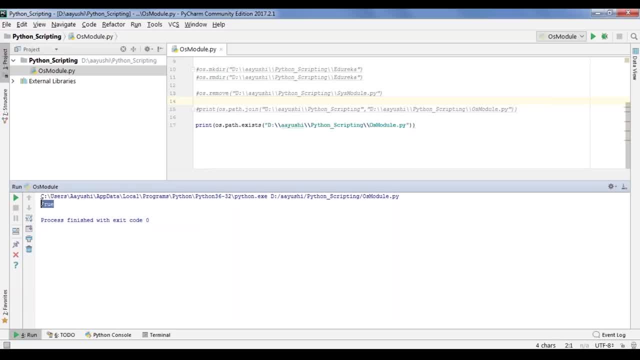 So now, as you can see, this path exists, So it is giving me the value true. Now, similarly, if the part doesn't exist, it will give you the value as false. So these are some of the methods which are used in the OS module. 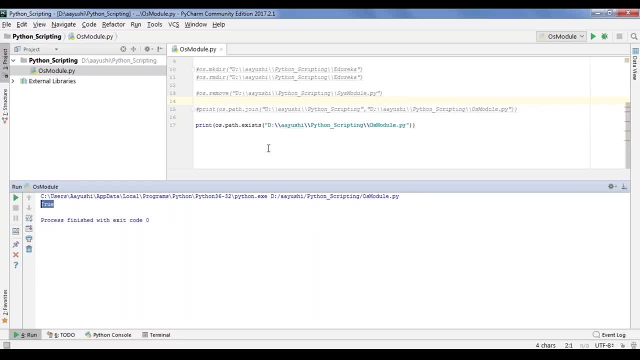 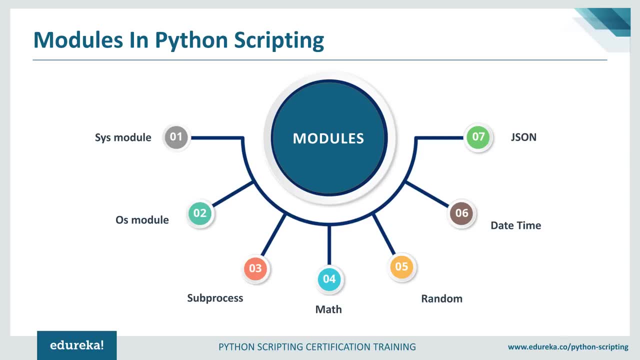 Next let me go back to my presentation and pick up the next module. So my next module is sub process. So this model basically lets you interact with operating system to create new processes, pass the information into and out of them and then get the return codes. 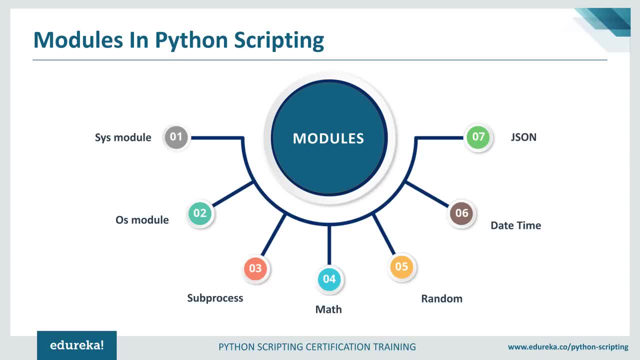 So it can be used by using the call function. So you can simply write sub, process, Call. and what will it do? it will basically run a command, wait for the commands to finish and then gives back the return code. So this is pretty much basic, guys. next, 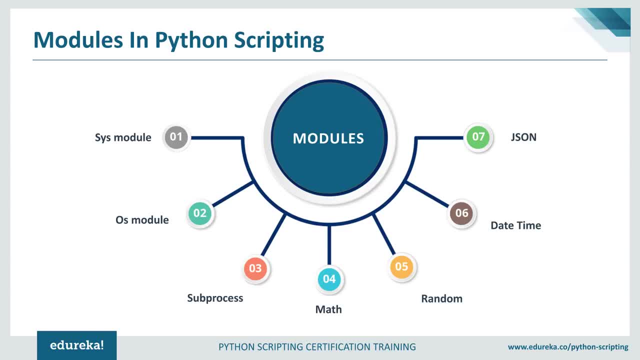 Let us talk about the next module, that is, the math module. So, as the name says, it performs various mathematical functions. Let's say, if you want to find out sine of X or let's say tan of X, you can do it very easily using this module. 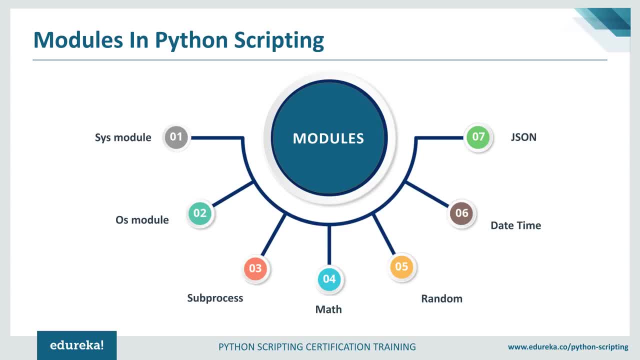 You can also convert a number from radians to degree or vice versa, or you want to calculate the natural log, or let's say, log base 10, and a lot of other things. so using this math module, you can perform angular conversions, hyperbolic functions, special functions and you can do a lot of other things. 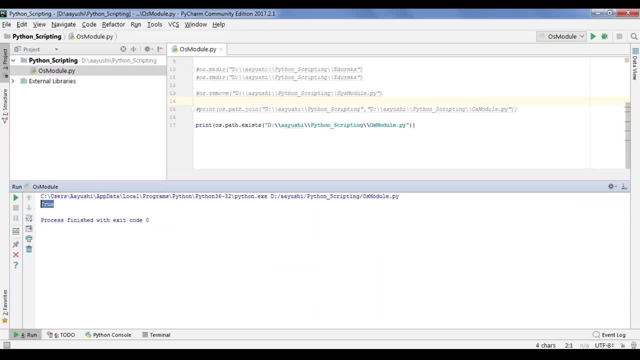 So let me just implement few of it for you. So I'll again go back to my pie charm. I'll create one more file. Let's say this is maths module. So first of all I need to import it. So I'll type in: import math. 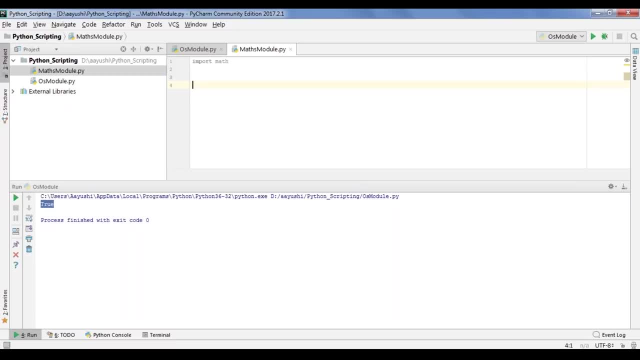 So now let me just return the value of constant. So for that, what I'll be doing, I'll be typing in math, I'll be first typing in print and inside that I will printing the value of pi. All right, so let me just run this. 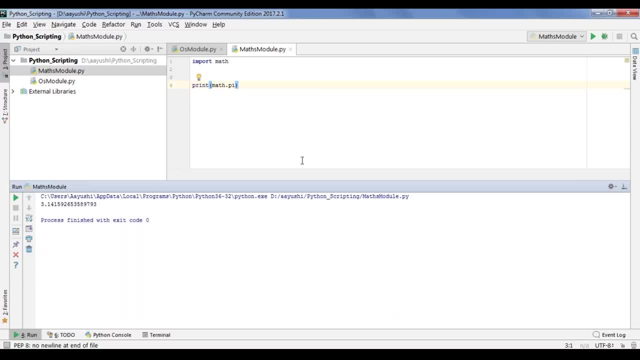 So, as you can see, the value of pi has been printed. next, what you can do, you can return the value of a constant also. Let me just type in math dot e. So this is basically returns me the value of constant e. So, as you can see here, the value of e has been printed next. 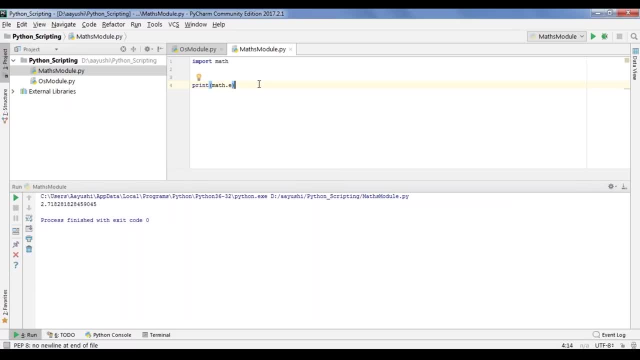 what you can do. you can also convert an angle from radians to degree. So for that, what I'll be doing, I'll be typing in print math dot degrees. inside that I'll be writing any value, Let's say 0.1, and let me just print it now. 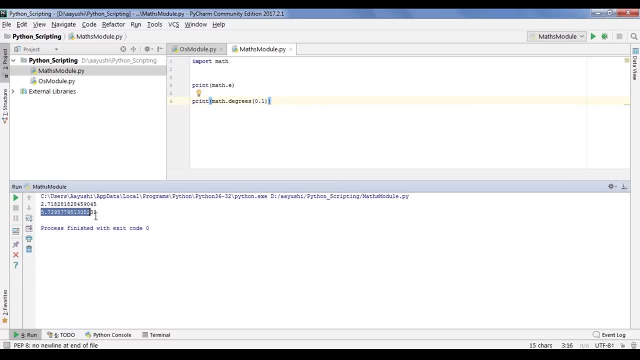 So, as you can see here, the value has been converted from a radians to degree that is 5.72.. Similarly you can find the cosine of X, or you can say any value in radians, in degrees or anything, So let me just do that as well. 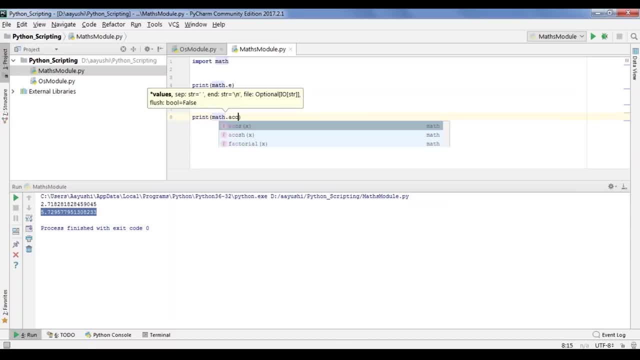 So I'll just type in print math dot a cos and inside this I'll be giving a value, Let's say 0.5, and let me just comment the above statements. And now let me just run this so that you guys will not get confused. 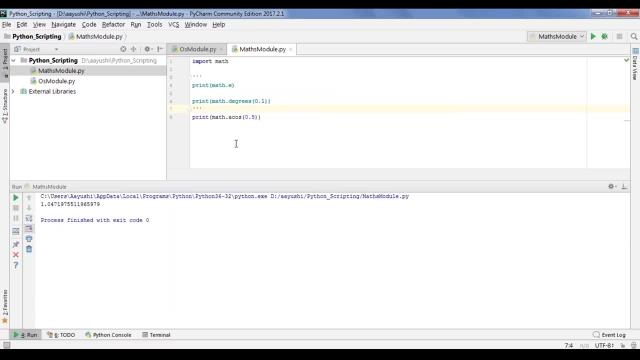 So here, as you can see, the cosine value has been printed. next, I want to do it for the sign as well, So I can simply type in a sign and let me just run this. So here the value of sine has been printed. similarly you can do for tan as well. 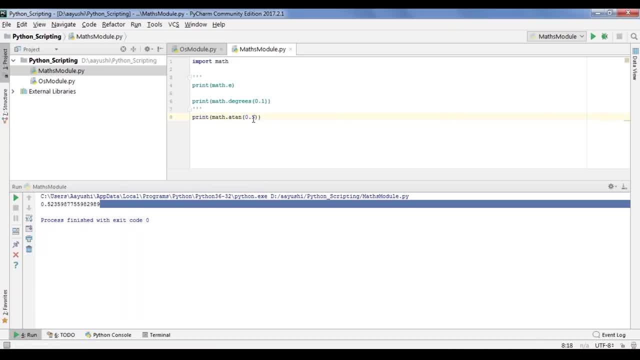 Let me just type in a tan and I'll be giving the value, Let's say 5, and let me just print it now. So, as you can see here, the value has been printed. So why we're writing a? because it will basically return. 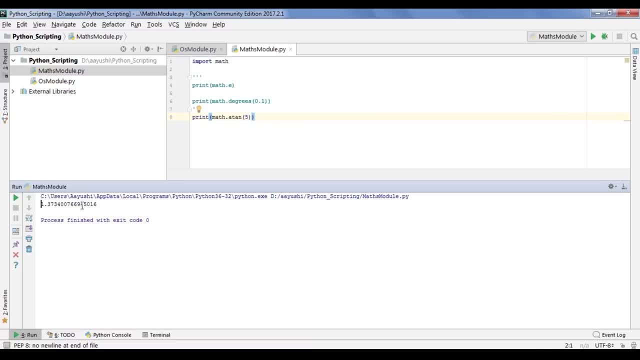 the arctangent of X in radians, which is the value present over here You can also type in: let me just copy this and let me just paste it over here. All right? So, in spite of writing a tan, you can simply type in: cos. 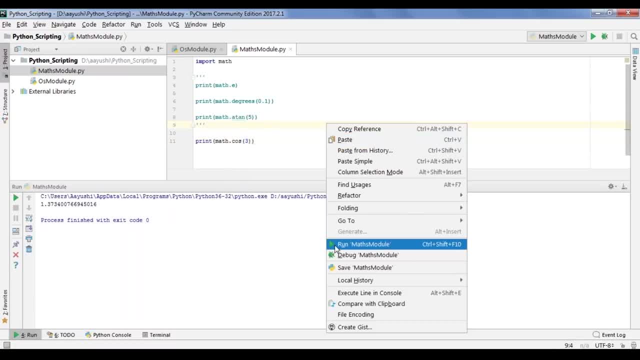 and inside that I'll be giving a value. Let's say 3, and let me just print it now. So here it turns me: the cosine of X, or you can say the cosine of 3 in radians. Now we have a lot of other functions as well. 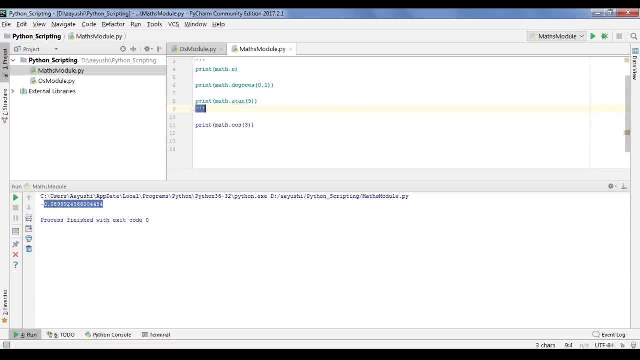 So let me just implement power and logarithmic functions. So let me just comment this till here And I'll just copy it. I'll paste it over here. So let me just implement some of the power and logarithmic functions. So I'll just type in math, dot, exp, and inside 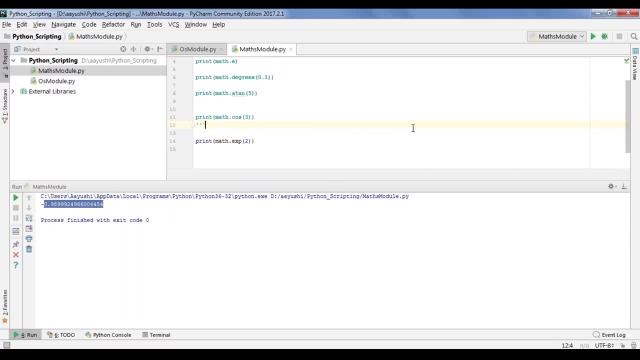 that I'll be giving a value to. so this will basically return me a raise to power 2.. So if you just run this, so, as you can see here, it returns me the value of e raised to power 2.. Next, let me implement one logarithmic function as well. 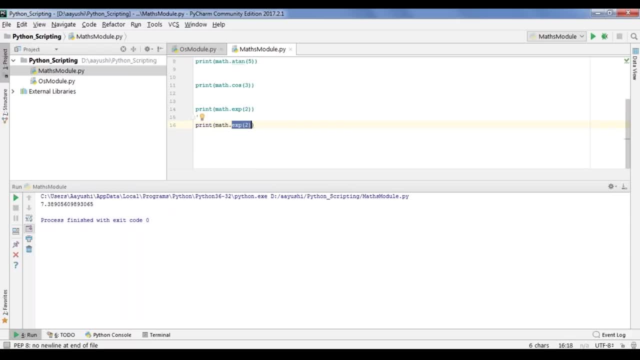 I'll just copy this first, And instead of this I'll be typing in math dot log, and here I'll be saying: X, comma, base. So here, with one argument you can return the natural logarithm of X to the base e, and with two arguments. 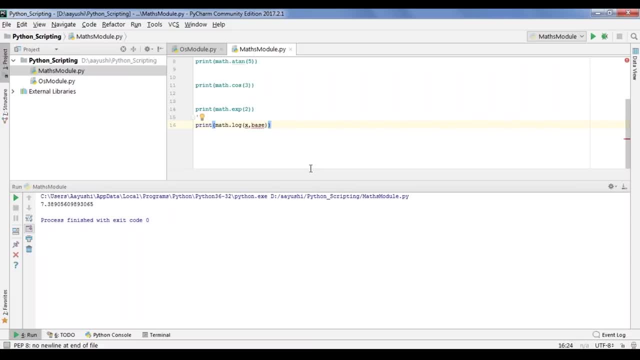 you can return the log of X to the given base. So let me just do that as well. I just typing X base 10, or you can say 10 base 10.. So if we just run this now so we know that log 10, base 10 is 1.. 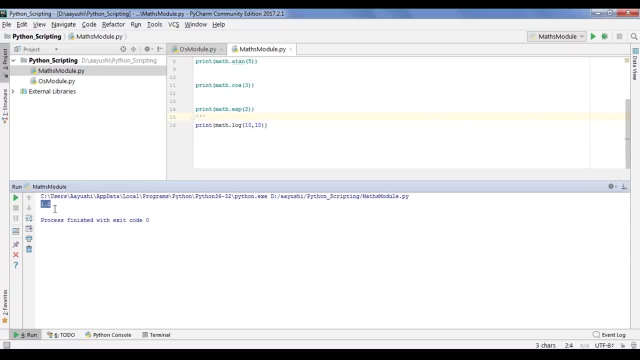 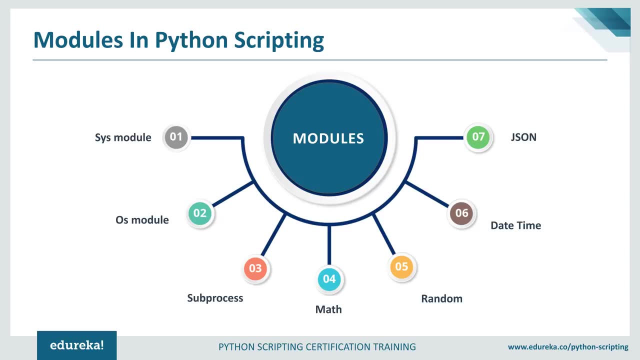 So it's giving me the value 1.. Let's let us go back to my presentation and let's see what is the next module. So next is my random module. So this module will basically helps you to generate random numbers. So it's a pseudo random number generator. 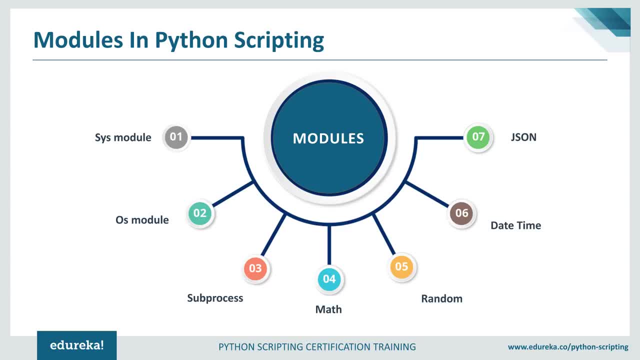 for various distribution. Let's say you don't want to type the number, So you'll ask your computer to generate some random numbers, and that is how it is used. So let me just go back to PyCharm and let us implement few of the operations of this random module. 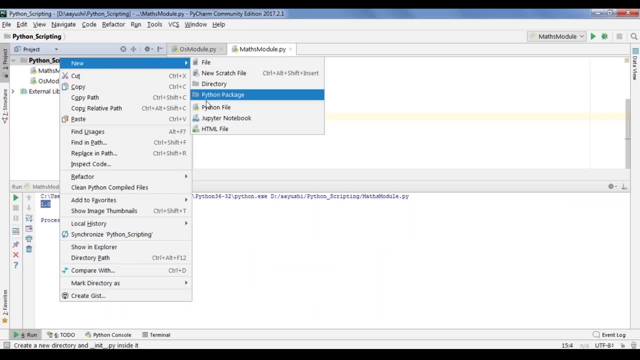 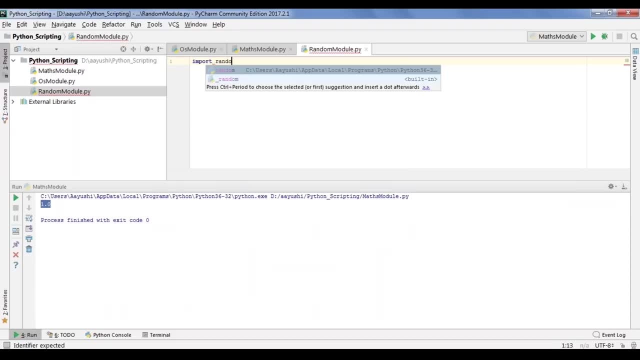 So now let me just go ahead and I'll create one more file which I'll name as random module. All right, So first of all, I need to import the module that is random. next, Let me just print some random numbers. So for that, what I'll be doing, I'll be typing in: print random. 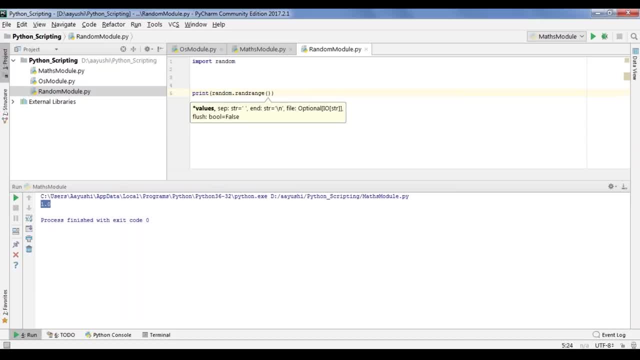 dot Rand range and I specify the range. So I'll type in 0 comma 50.. I can simply say 50 and let me just print this. So this will basically give me the number, which will never be greater than 50.. So, as you can see here, 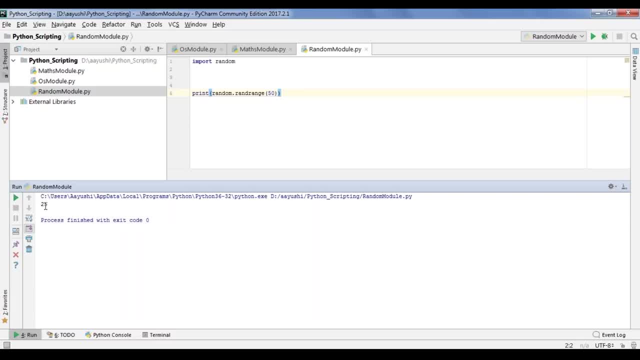 it gives me the number 2. then let me run it again. It has given me 25.. Let me run it again. It is giving 38, and so on. the numbers will be generated, but again it will not exceed the number that is 50 now. 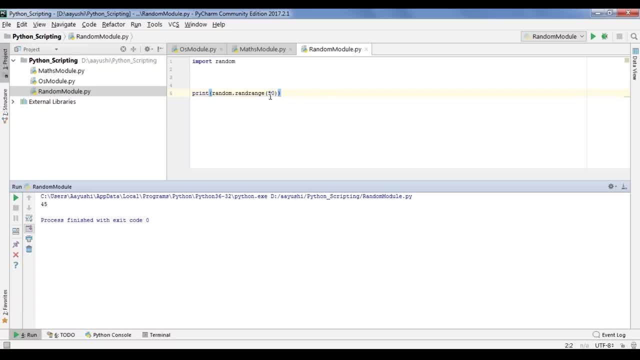 if I want to make this in a range of, let's say, I want to make it in the range of 0 to 50. So here it will just give me the numbers between 0 and 50 and also you can add some steps to it. 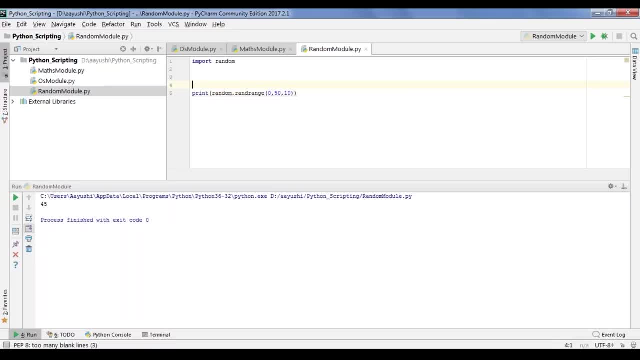 So let's say I want to step size to be 10.. So let me just print this and let us see what does this step size me? So here, if you see, it's giving me the result in step size of 10, so it's giving me 10. then is giving me 30. 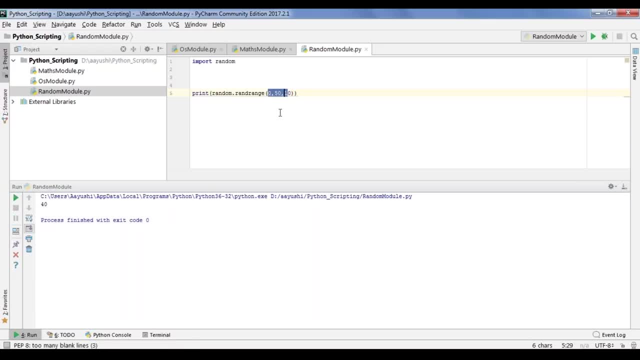 then it's giving me 10, again 20.. So basically it gives me the output between 0 to 50 and in the step size of 10 should not be less than 0 and will not be greater than 50. now You can also change the step size. 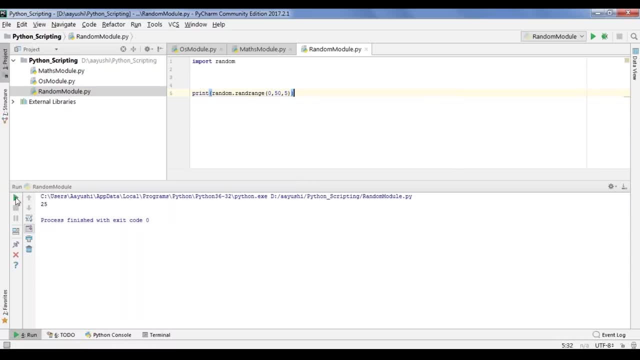 Let me just change the step size to 5, and now let me just run this. So, as you can see, here it's giving me in step size of 5.. So here it has been printed 25, that's giving me 20, then it's giving me 5. similarly, there will be numbers. 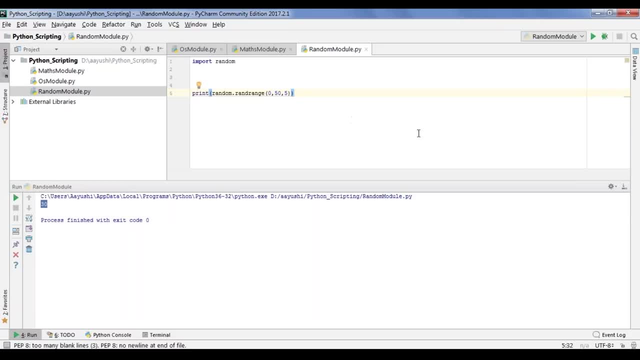 that will be generated now. next, if you want this in integers, So what you can do, you can simply type in print random, don't run in, and you can specify the range. So let's say I want the range in, let's say 0 to 20.. 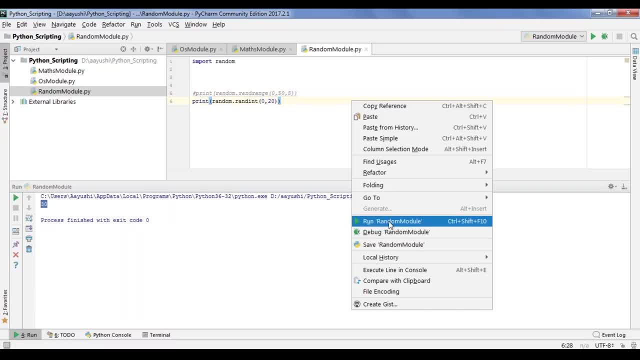 Let me just post, comment this and let me now print this. So now it will give me the random numbers, or you can see the integer numbers between the range that is 0 to 20.. So here it's giving me 9, then giving me 2, it's giving me 6. 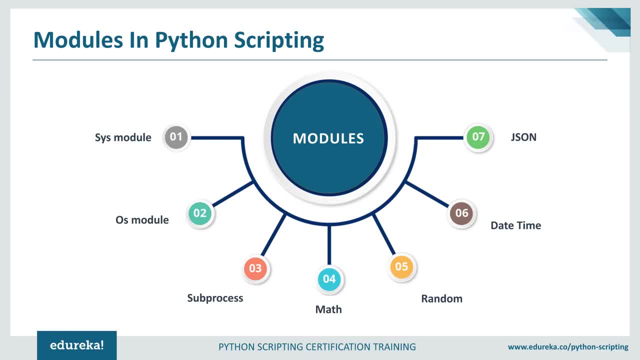 and hence the number will be generated like these. So now let me go back to a presentation and let's see what is my next module. So my next module is date time module. So this module basically includes the tools for working with dates, time and their combinations. 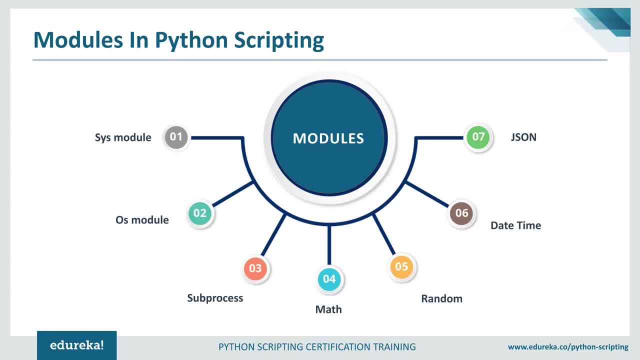 So the time module includes the tools for working with time and dates in the recent past to the near future. So it focuses mostly on manipulating time based on the computers internal representations of time. So let me go back to pie charm and let's implement some of the functions of this module. 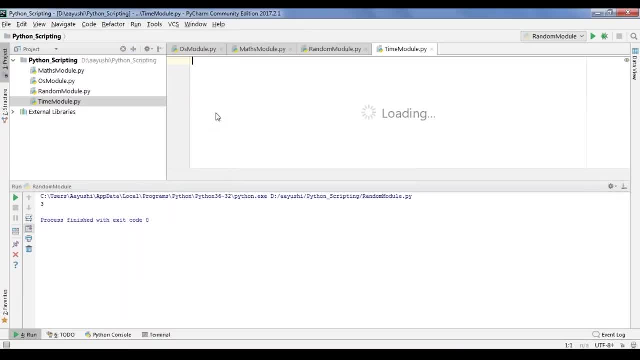 So I'll just create a new file, Let's say time module, and first of all I need to import it. So I'll just type in import date, time. Next was, let's Prince, today's day, So for that what I'll be doing. 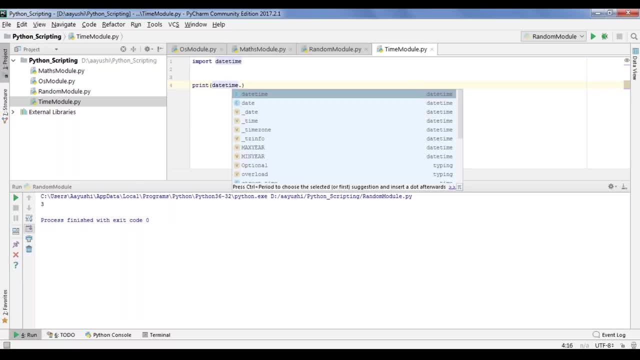 I'll be typing in print: date time dot. date Dot, today. So now let me just run this. So, as you can see here, the current date has been printed, So today it's 21st March 2018.. So now you can also perform some arithmetic function on this. 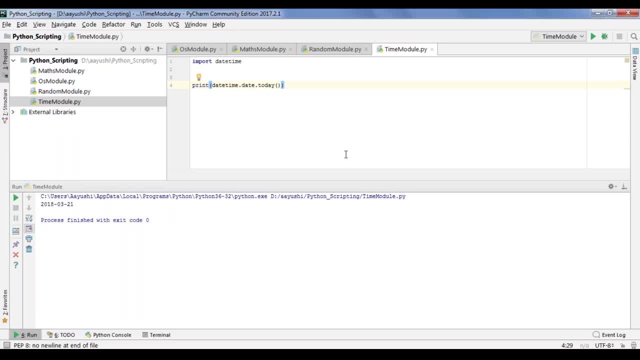 For example, when you perform an arithmetic function on date time object, you will get the result in a time Delta object. So basically the attributes are days, seconds and microseconds. 12 create a new object. Let's say now and say date time, dot date time. 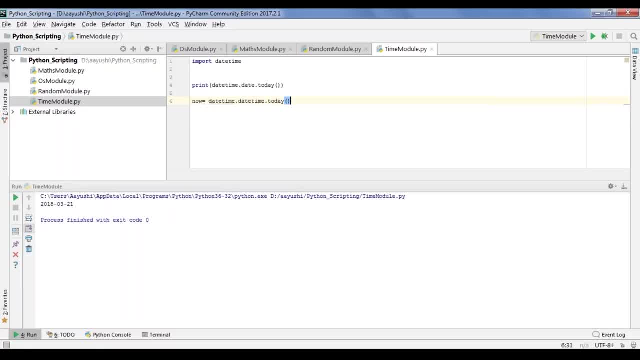 Dot today. So now, what I'll do? I'll print the difference between the two dates. So what I will do, I'm applying some arithmetic operations to them, where you will get the result in a time: Delta object. Let me create one more object. 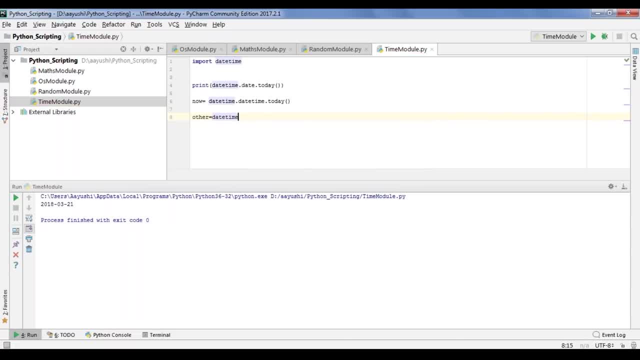 Let's say other, and I'll say other. dot date equals to date time, dot date time, and I'll mention a date, Let's say 1994.. And now let me just print the difference between these two objects. will I say: print now Minus other? so now let me just comment the above print statement. 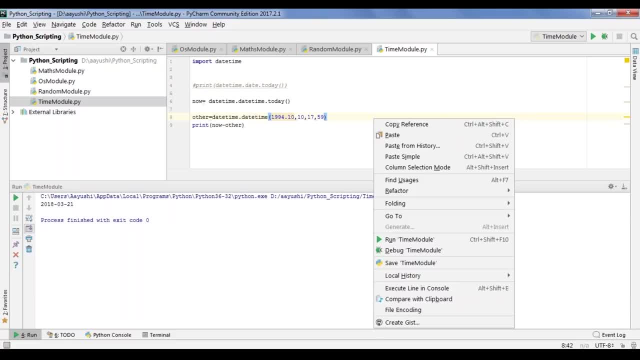 so that you guys do not get confused. and now let me just run this All right. So here I have not specified a comma, So now let me just run this All right. So as you can see, here, difference between these two dates has been printed. 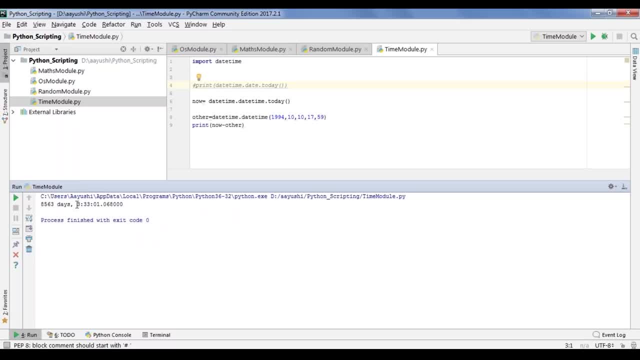 So I have already told you that the attributes for these are days, seconds and microseconds. So here it is telling me that 8563 days are there, And then we have the other detailing as well. Next, let us see the last module, that is, my Jason module. 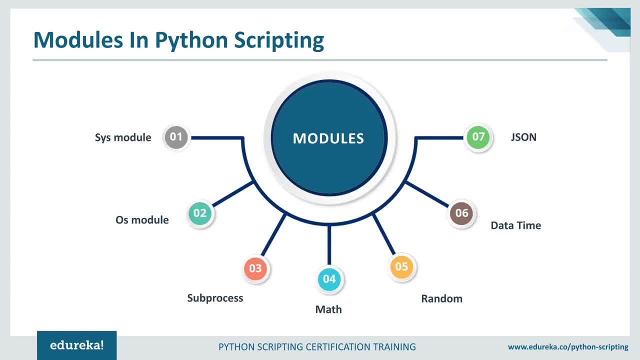 So Jason is popular communicating between the web servers and the clients. So in Python the Jason module provides an API similar to convert in memory Python objects to a serialized representation that is known as Jason, or you can say JavaScript object notation and vice-versa. So Jason has the benefit of having implementations. 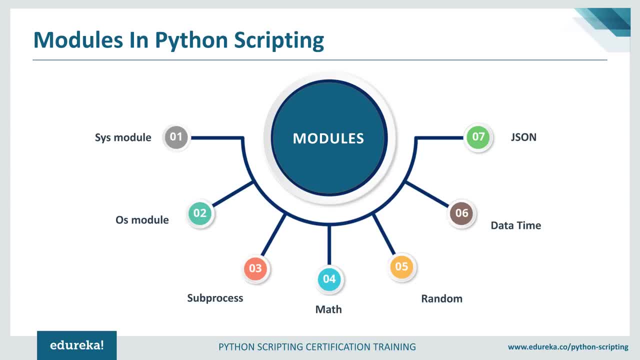 in many languages, and especially JavaScript, making it suitable for your inter-application communication. So this Jason module provides an easy way to encode and decode data in Jason. So now let me just go back to my pie charm, and I just implement this as well, So I'll create one more file. 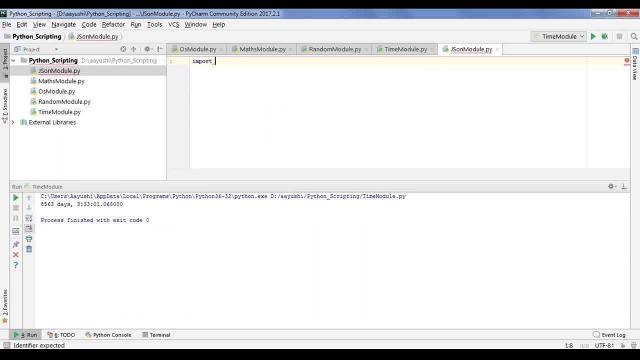 Jason module. first of all I need to import it, So I'll just type in import Jason. So now what I'll be doing, I'll be first typing in some data in Jason. So let's say I have an employee data, So I'll say employee data. 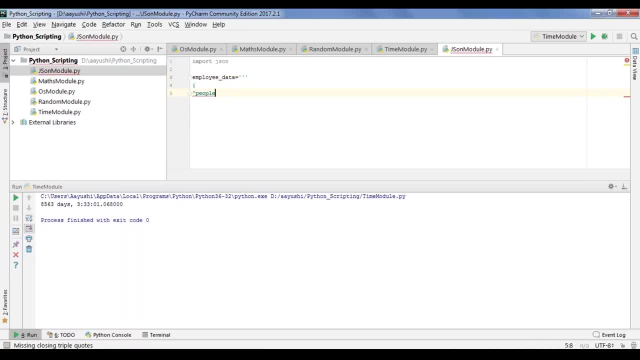 Equal to. let's say, I have some people, Let me just give some attributes to them. So I'll say the name. Let's say the name is Ayushi. Then I specify an email, So I'll type in email and then I'll just type in. let's say: 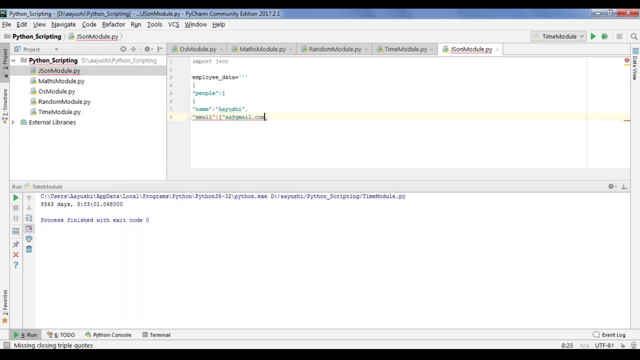 a at the rich gmailcom. and then let me just give one more email ID, Let's say had the rich email again. Then I'll give one more attribute, Let's say married, or you can say the marital status. So I'll say false and just close this similarly, 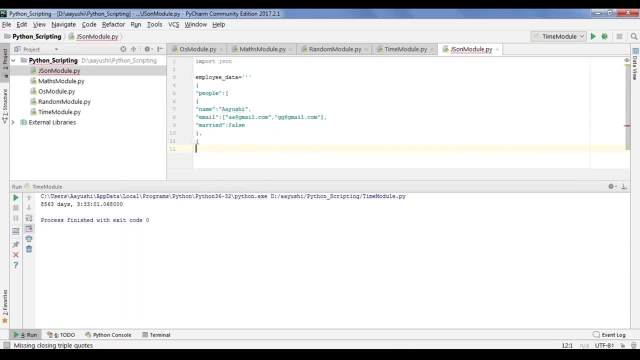 I'll take one more, So I'll just copy it from here, I'll just paste it, I'll just change the name. So let's say this time It's a Namika. I'll change some email ID as well, And now let me just print it. 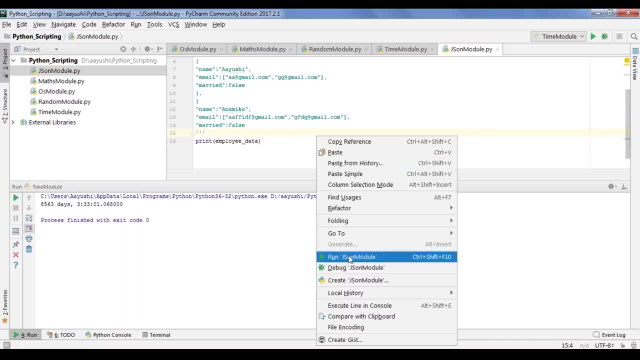 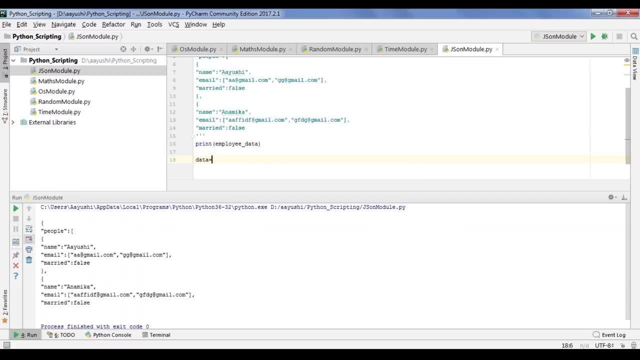 So I'll just print this employee data. So, as you can see here, my Jason has been printed. now let me do it in Python as well. So I'll just take a variable- It's a data- and I'll just load this Jason. 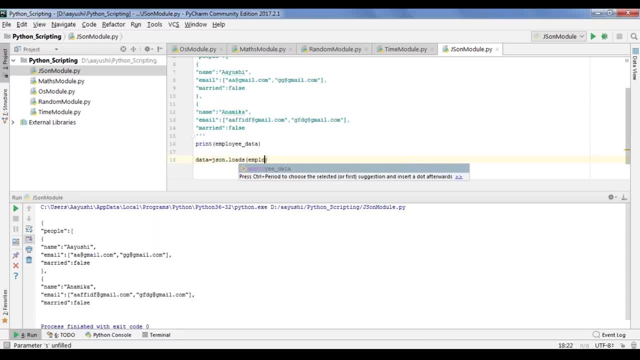 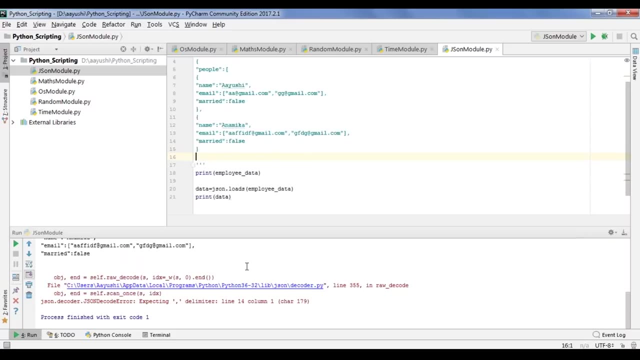 So I'll say: Jason dot loads inside this. I'll be just passing my Jason, that is my employee data and I'll just print it. Let me just run this now. All right, just giving me some error. All right, so I haven't closed this. 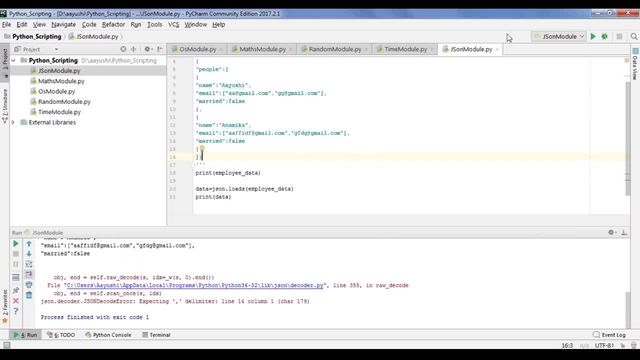 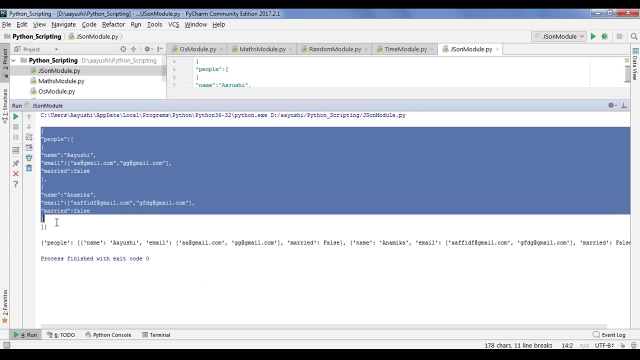 So I'll just close this, All right. So I guess it will work now. So let me just run this now. Yes, So as you can see here my Jason, which is being printed over here, and that is how I just load the data in Python. 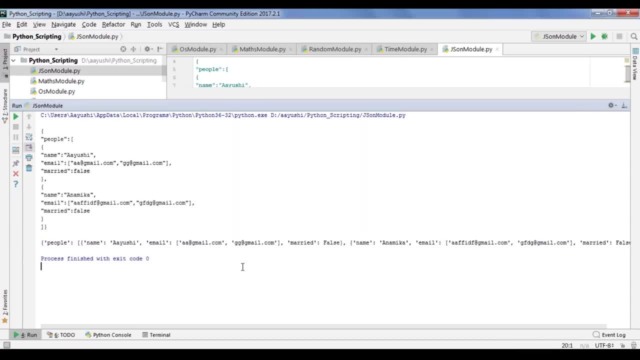 It gives me this result. So basically, it has converted your Jason to a dictionary. So whenever you load Jason into Python, it uses some conversions, such as your Jason object hasn't converted to dictionary. So, as you can see here, your data has been in key value pairs. 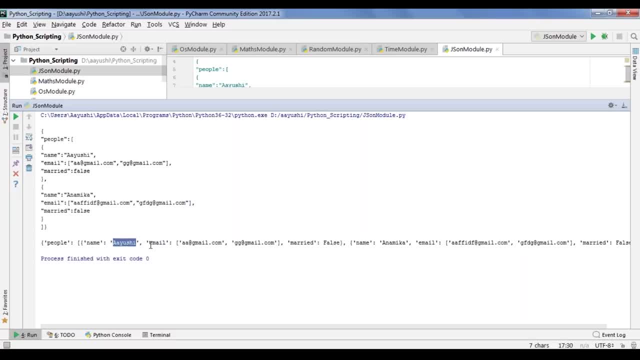 Also, this is my key and this is the value to the key. Similarly, I have another key, which is email, and this is the value to it. So, basically, whenever you load the data in Python, it has the object or you can see the JSON object is converted. 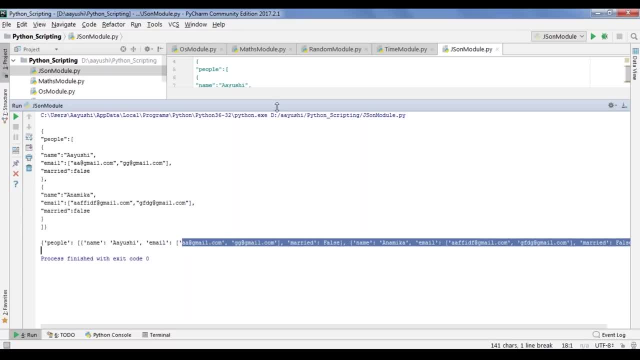 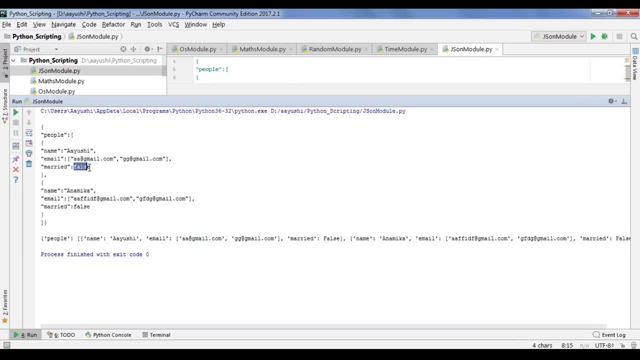 to a dictionary. Now there are also few more changes which has been done. So if you see here, such as your array has been converted to list, then if you see here you have a JSON which says that marriage falls, and if you see here it has been converted. 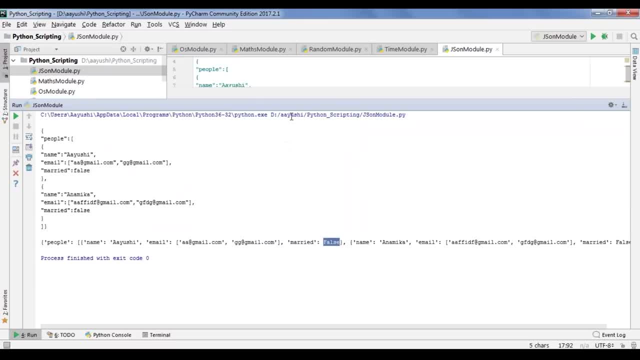 to the uppercase falls. So these are some of the conversions which Python do. this one more conversion where you have a value which is null and then, if you see it over here, it will be changed to none status. How, whenever you load a JSON into Python. 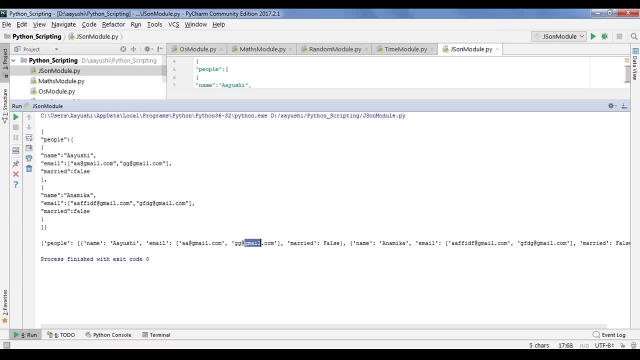 it uses some conversions also. this JSON module provides an easy way to encode and decode in JSON. So there are basically two main functions, which are Jason dot dumps and Jason dot loads. So I've already told you about Jason dot loads. So here you have a function which says Jason dot load. 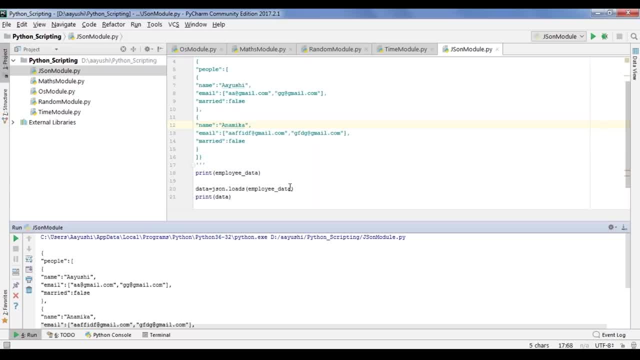 and inside that you can just load a file. Similarly you have Jason dot loads. So basically this does a difference of S. So whenever you want to load a string, so for that what you can do, you can just type in Jason dot loads and inside the brackets you can pass on the string value. 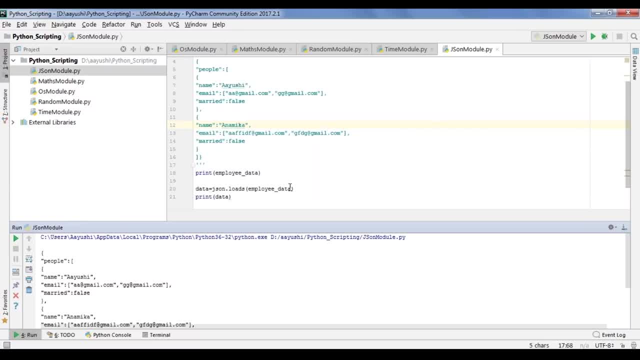 Now you have another function which is called a Jason dot dump. So using this function you can just load the JSON object to a file and again, if you type in Jason dot dumps, you will be having an output- Jason object as a string. So that is how Jason object plays a major role. 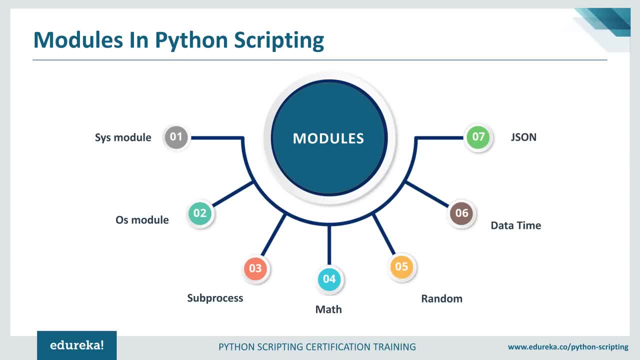 in the modules in Python. So now let's move on to our next topic, that is, AWS scripting. So here we will be talking about the boto module, which is an AWS SDK for Python. So in AWS will be performing two tasks First of all. 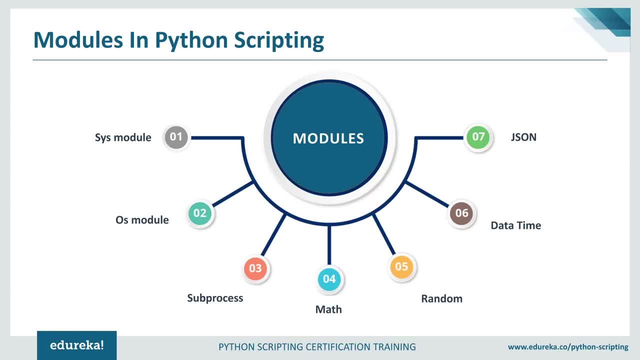 we'll be creating an EC2 instance and then we'll create a S3 bucket. Now let us see how you can configure this boto module. So, first of all, to import boto, you just need to type in pip, install boto3 and once the installation has been done, 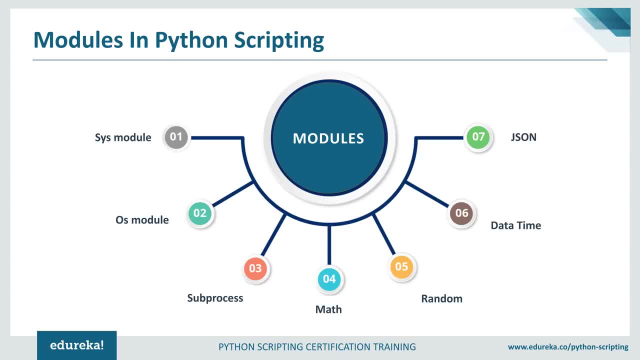 you also need to install the AWS command line. So for that you just need to type in pip, install AWS CLI. many times There are some problems regarding pip. So what you can do, you can go to Google and you can just download the MSI file for AWS CLI. 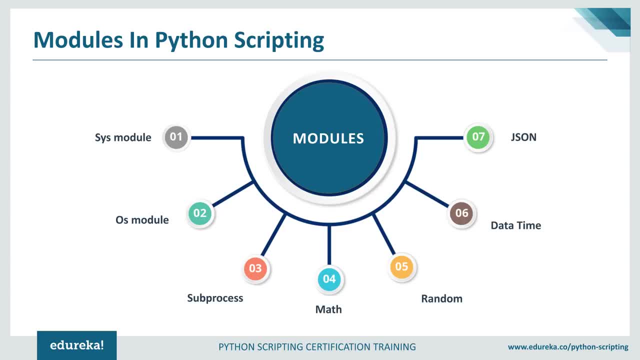 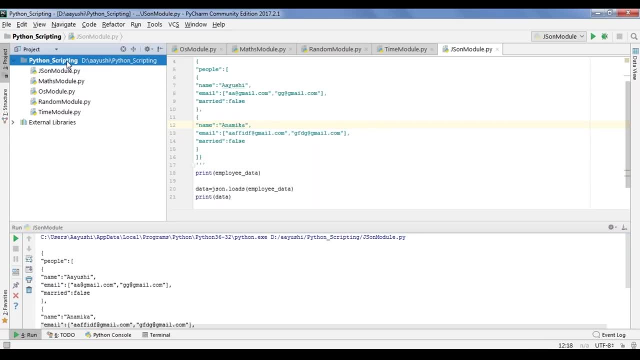 Then, once this is done, you can just type in AWS configure and then they'll be asking you for the access key. So now let us just go to my pie chart and let us implement how we can do that. So I'll just create one more file. 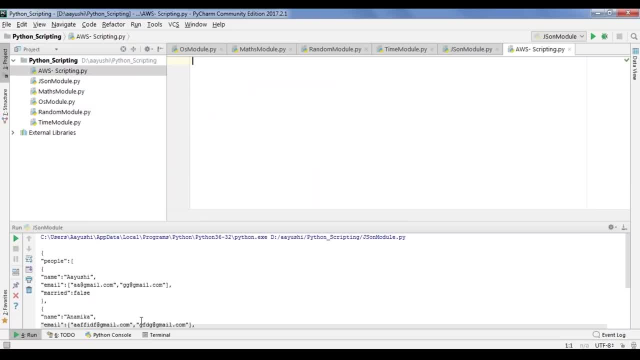 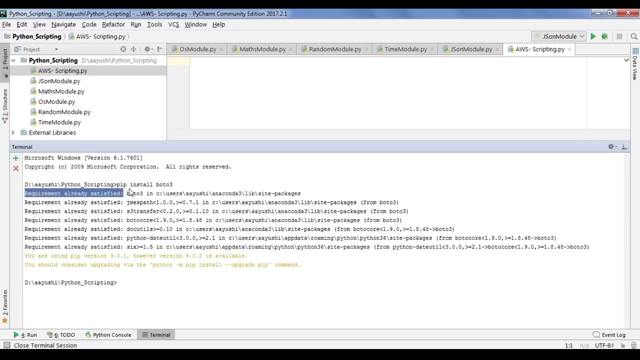 Let's say AWS scripting. So first of all I'll just go to my terminal, So I'll just type in: pip, install boto3.. So now this will take some time. So now it tells me that the requirement is already satisfied. So I already have my boto3 installed. 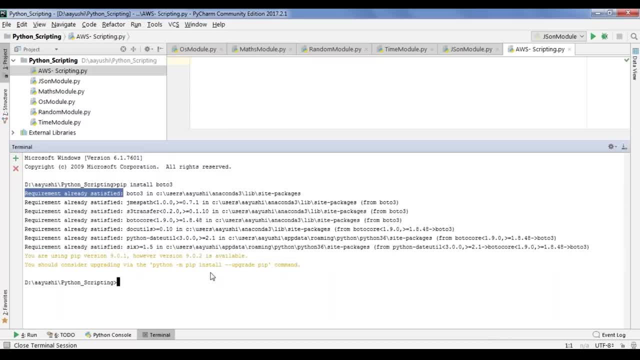 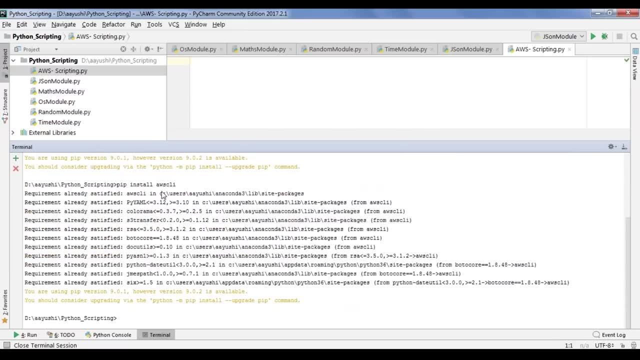 So next what you need to do? you need to install the AWS CLI. So I'll just type in pip, install AWS CLI and hit enter. So again, I have already installed my AWS CLI. So again it's giving me this statement that the requirement already satisfied. next step: 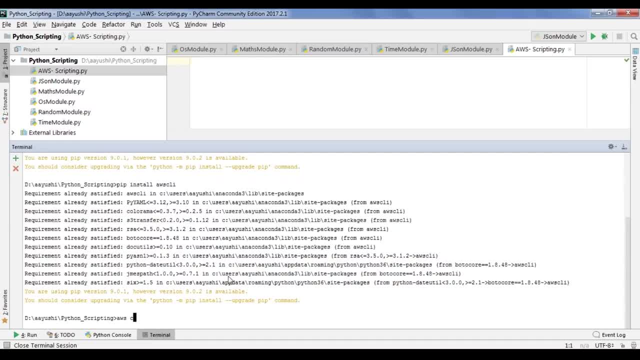 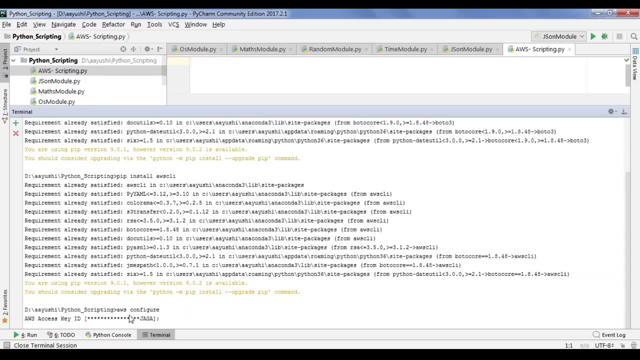 You need to type in AWS configure. so I'll just type in AWS configure. So now, as you can see it asking me for the AWS access key ID, So what I will be doing, I'll be going to the AWS management console and be generating a user which has an access key to it. 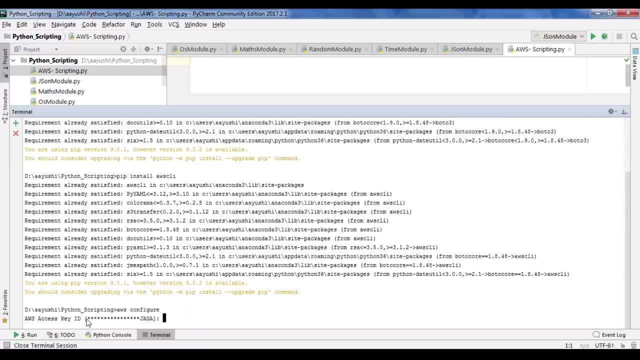 So once you configure your AWS, it will ask you for the AWS access key. So now, to find that access key, what you need to do? You need to go to your AWS management console and there you have to create a user which will be having an access key to it. 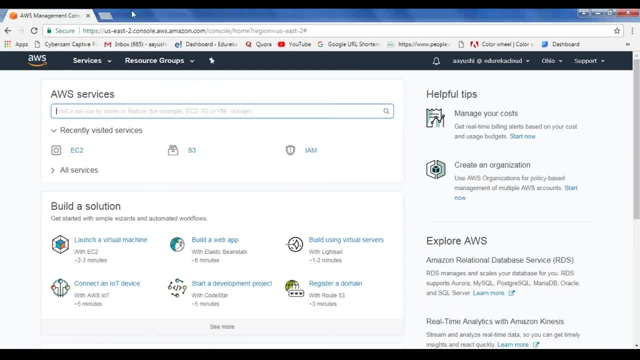 So let me just go to my AWS management console. All right, So this is my AWS management console. So over here I'll be just typing in: I am, which basically stands for your identity and access management. So over here you just need to go to users. 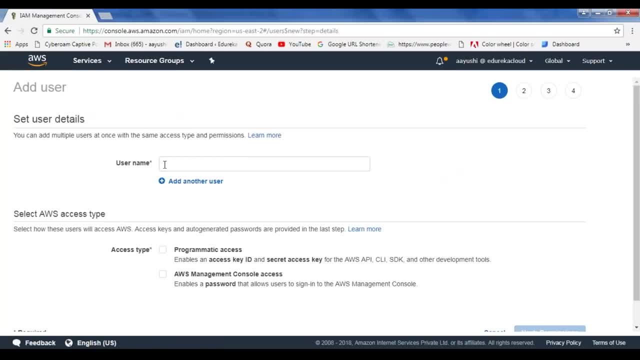 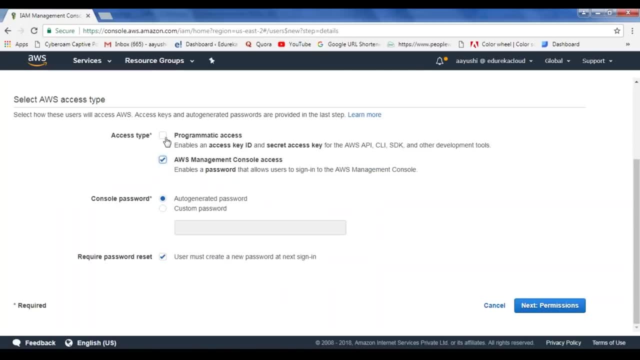 and just add a user over here. So I'll just create one user over here. So I'll say user. I'll give a name to it. So let's say user one. Let me just give the permissions to it. Just click on next. 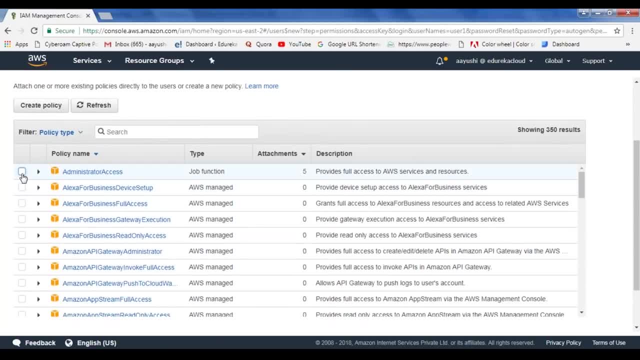 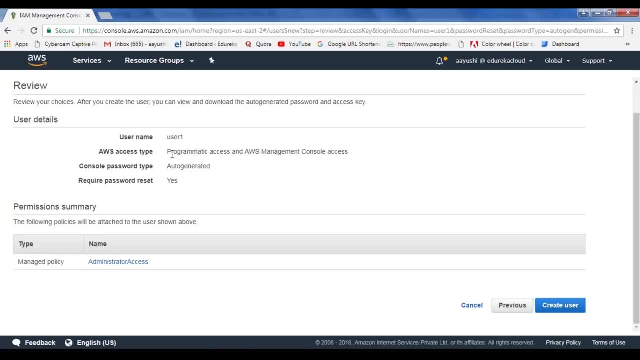 So I'll add some policies. Let me add some administrator access and then just quickly go and click on next. So here, as you can see, I have a user name, I have access type and you have all the required information. then you just need to create a user. 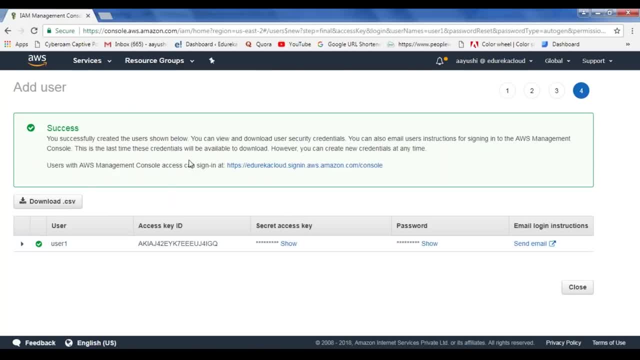 So I just click on create user. It will just take some time. So, as you can see, here I have the user which is named as user one, Then I have the access key ID and I have the secret access key along with the password. 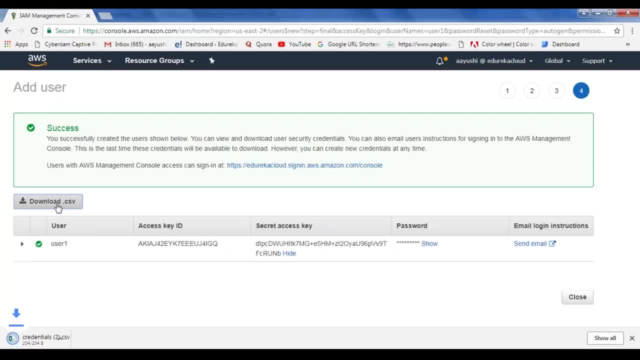 So here, what you need to do, you can simply download. It's a CSV. So I'm just downloading the CSV from here. Now, why I'm telling you to download it? because later, if you face any problem with the AWS authentication, you will not be able to access these keys. 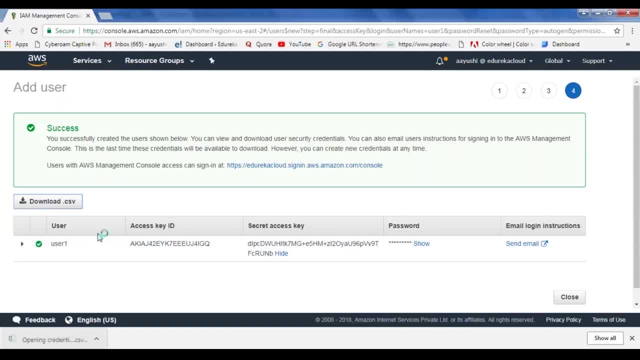 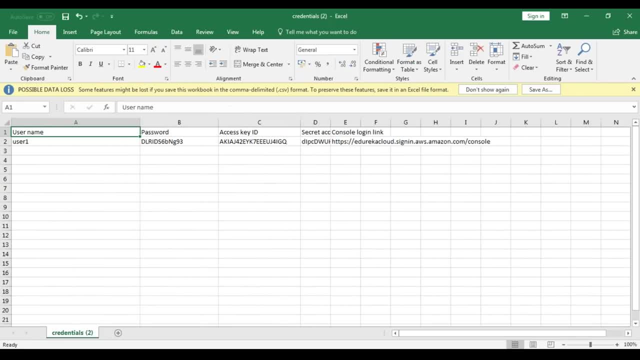 So the better way is to just download the CSV. So I just open the CSV and let me show you what all is present over there. So, as you can see, here, I have the user name, I have the password, I have the access key ID. 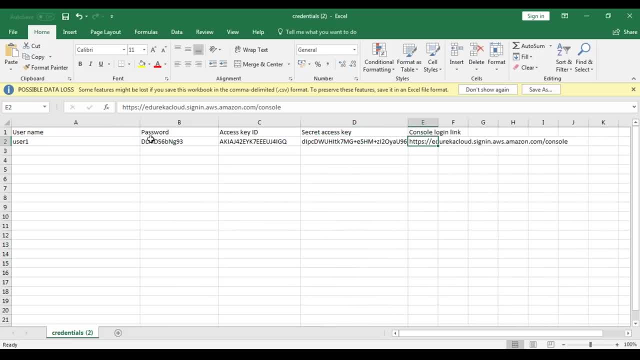 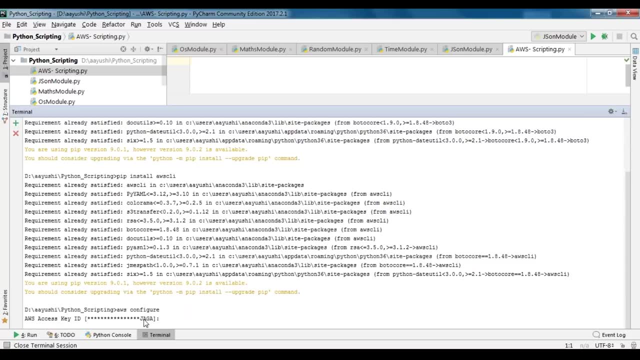 and I have the secret access key and this is the console link. So what I'll be doing, I'll be just copying this access key ID. I'll paste it to my pie chart. So it's asking me the AWS access key. So I'll just paste it over here. then ask me. 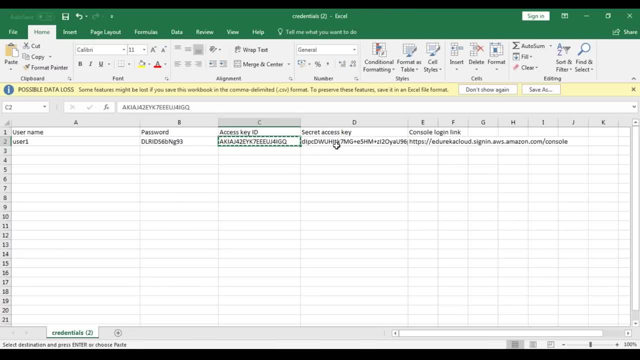 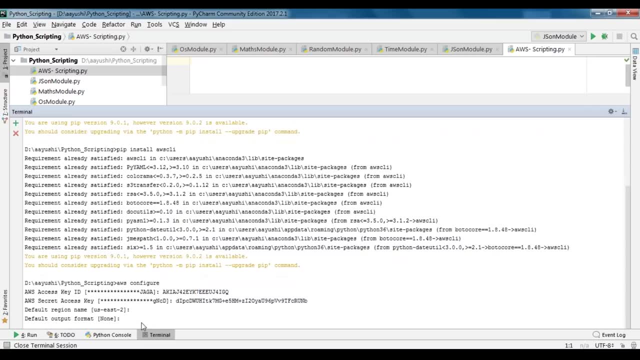 for the AWS secret access key. So I'll again go to that CSV and I'll copy this and paste it over here. then tells me the default region, which is the US East 2.. Okay, and I'll just click on enter. So here my AWS has been configured. 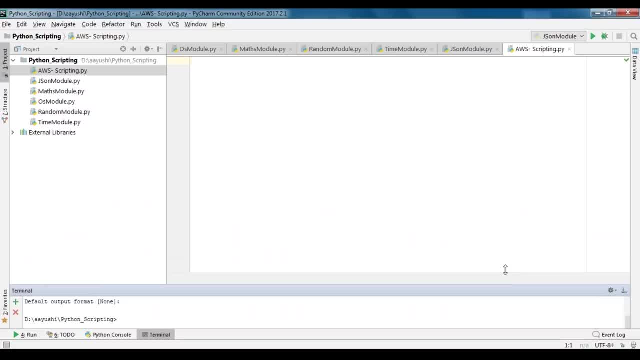 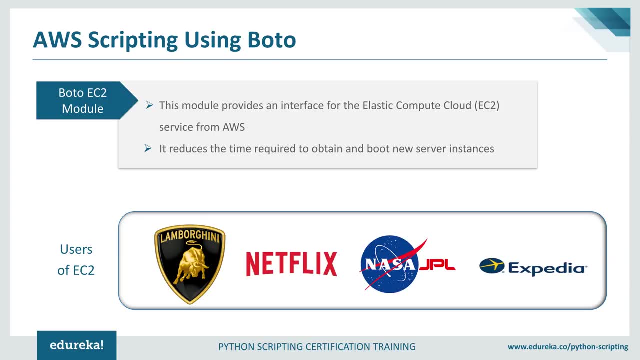 and the default region is the US East 2.. So now let me just go to my coding part and let us just write the script for it, But first let's understand what exactly they are So easy to basically stands for your elastic cloud computing. 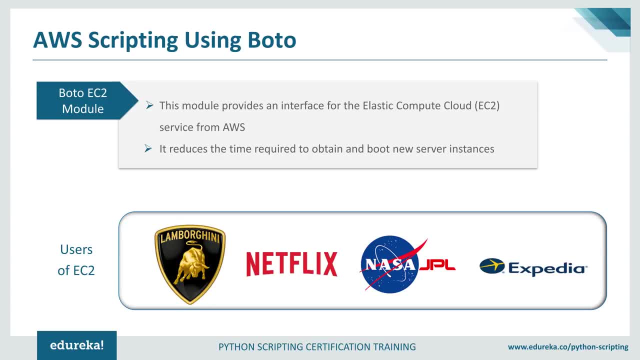 which is a web service which provides resizable compute capacity in the cloud. So it is basically designed to make the web skill computing easier for developers. So it allows the users to rent virtual computers on which to run their own computer application. So there are many big companies who use a ec2. 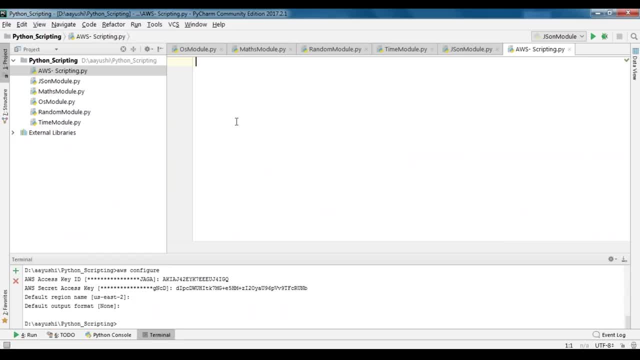 like Lamborghini, Netflix, NASA and many more like that. So now let me just go to my coding part and let us just write the script for it. So first of all, I'll just go ahead and import boto3. next, what I'll be doing: 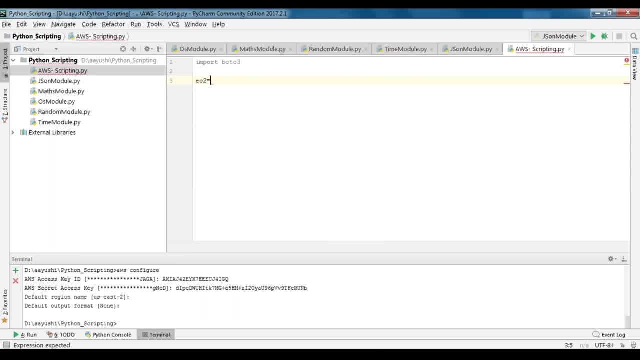 I'll be creating an ec2 instance. So for that, what I'll be doing, I'll be creating an object, Let's say ec2, then I'll say ec2 equals to boto3 dot resource And inside this I'll be passing ec2.. 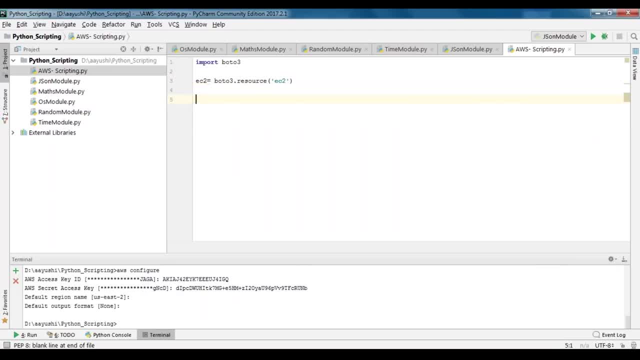 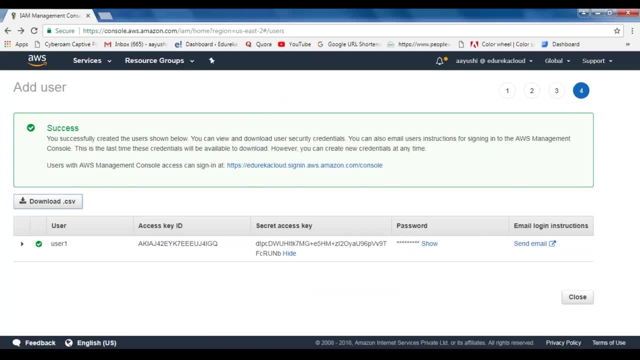 So here I'll be writing a script So to launch an ec2 instance without manually going to the AWS console and adding the instance over there, so I can show you that as well. So let me just go to AWS console. So here, as you can see, the first compute service is ec2.. 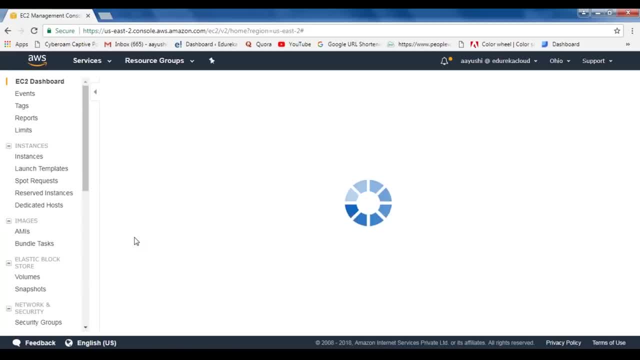 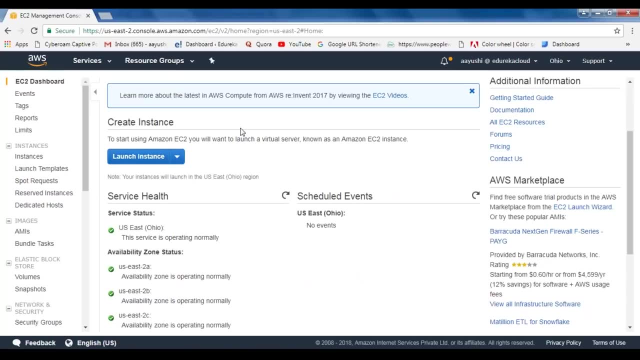 So I just click on it. So what you can do, you can come to this AWS management console and launch the instance from here. but in spite of this, what I'll be doing, I'll be writing a script so that an ec2 instance can be launched automatically. 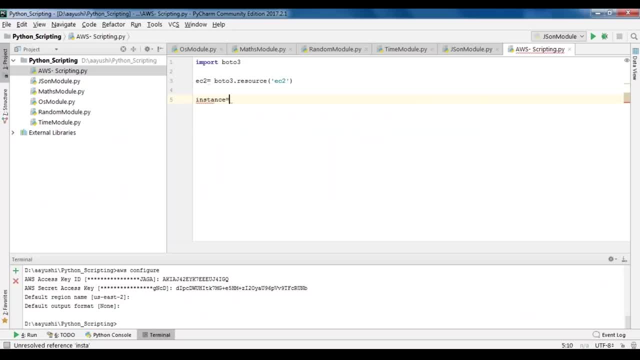 So next, what I have to do, I have to type in instance is equals to ec2 dot. create instance And inside that I'll be giving some specifications to it. So first of all, I've been giving the image ID, or you can say the AMI. 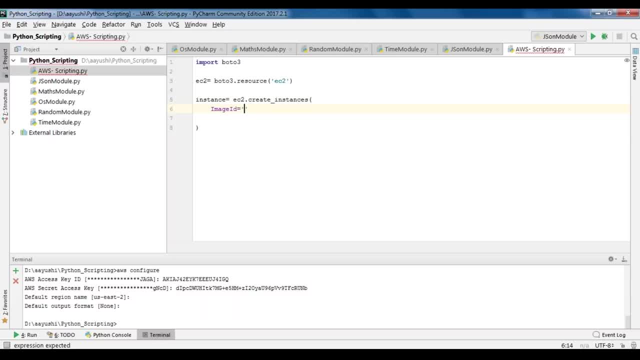 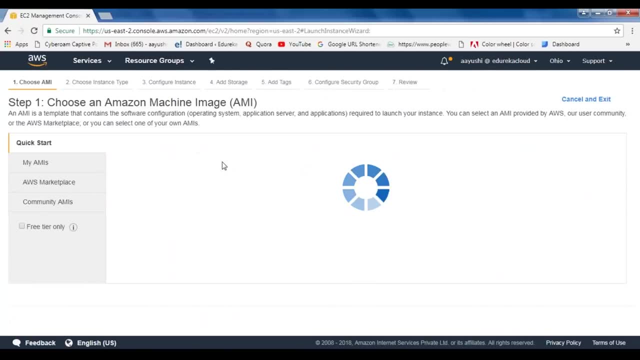 which stands for Amazon machine image. So here I'll be giving that. so from where I can find this image? So again, I'll go back to my Amazon console and I'll click over launch instance. So here, as you can see, I have my AMI. 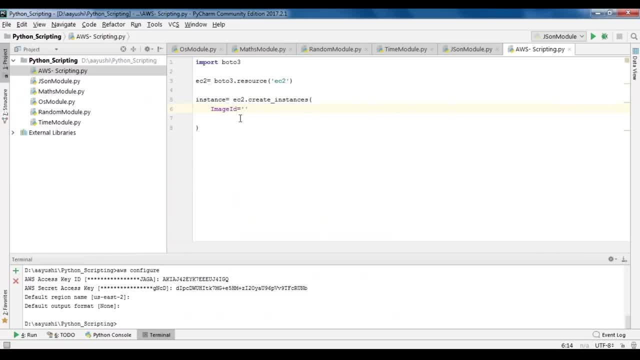 or you can say the image ID. So I'll just copy this image ID and paste it over here. next I just need to give the min count and max count. Next I'll be specifying the type of instance. So I have t2.micro. 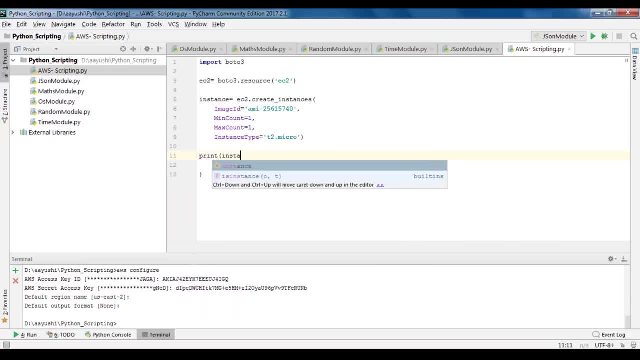 And finally, I'll be printing the ID of the instance that has been created or that has been launched. So I'll say instance 0 and I just type in ID. I'll just remove the extra phrase. All right? So here, as you can see, I have just created ec2 instance. 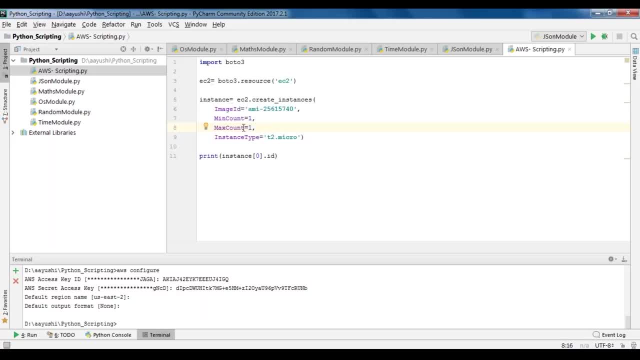 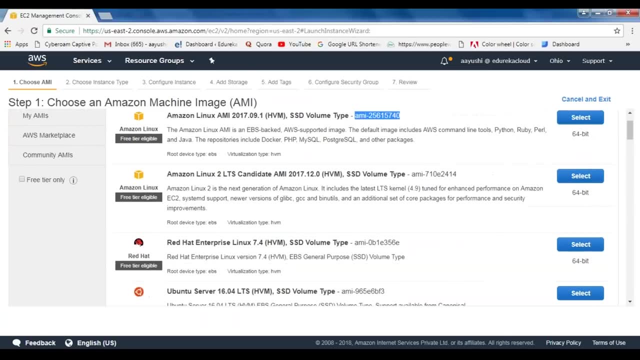 wherein I have just given the image ID and specify the min max and the instance type. So now let me just run this, or before that, I'll just go to my console and show you that there are no such ec2 instance running. So I'll go to an instances. 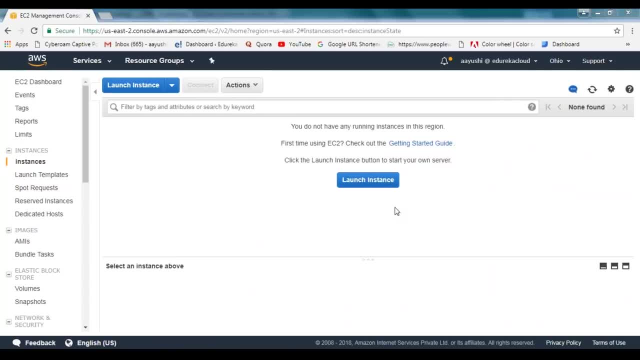 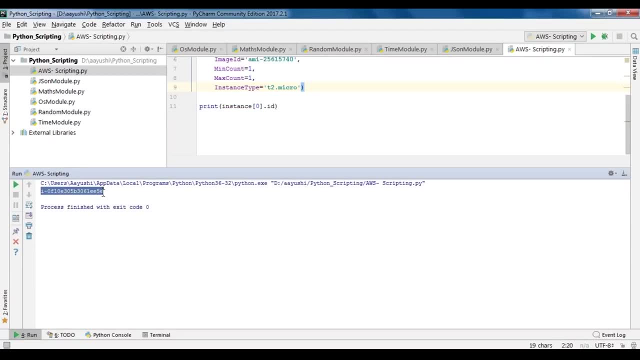 So, as you can see here, I don't have any instance. Let me go back to code and let me just run this code now. So, as you can see here, it has printed me the ID of the instance. So now let me go back to my console. 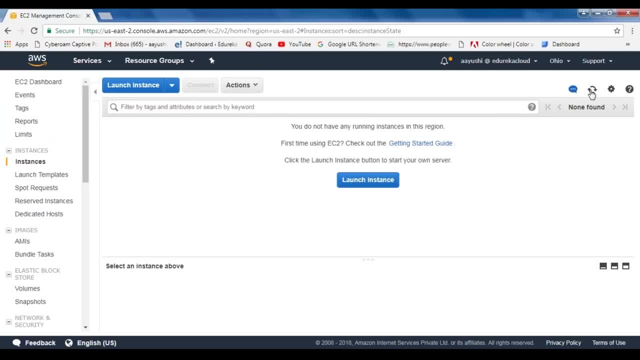 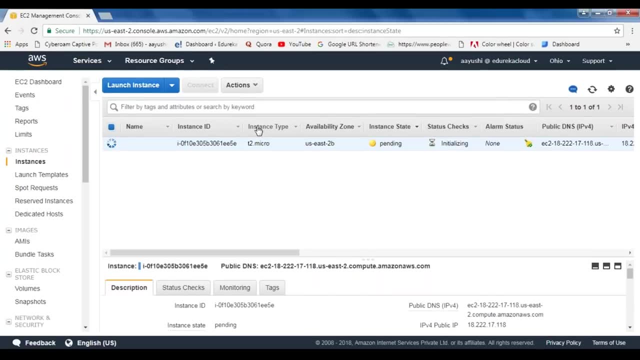 and let's see whether the instance has been launched here or not. So now let me just refresh this. So yes, it has been launched. It has the same instance ID which is given over here and the instance type is t2 micro and the instance state is pending right now. 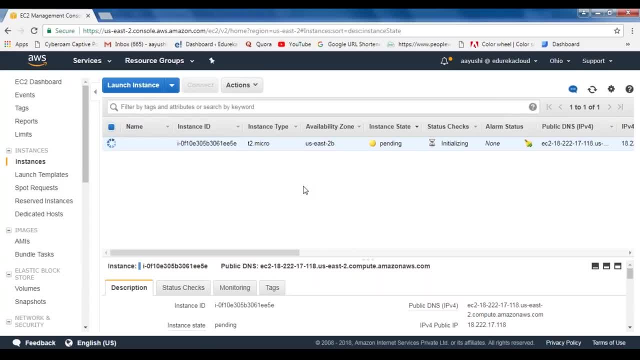 but it will be launched in just a few seconds, So let us just wait for some time. So, as you can see here, my instance is up and running now. Now you can also delete this instance, So you can also go here. you can click on actions. 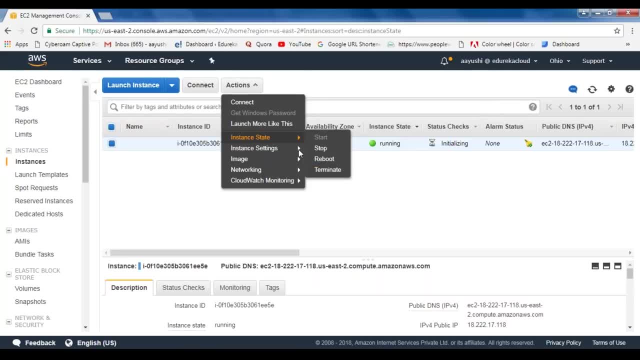 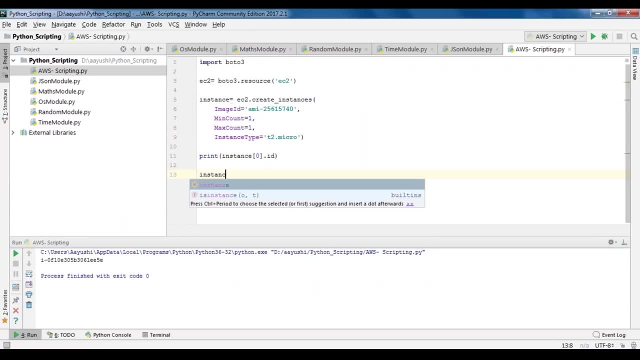 and you can just go to instance state and terminate it. But again, if you have to do it, to Python script, so what you can do, you can go to a pycharm again and you'll just type in instance ID. So I'll specify my ID, which is this: 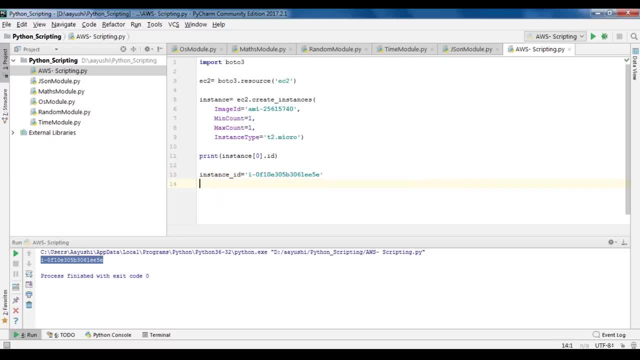 So I'll just copy it from here. Then what I'll be doing? I'll be just saying: instance is equals to EC2.. I'll give the instance ID to it. Then I'll be having response where in I will terminate this EC2 instance. 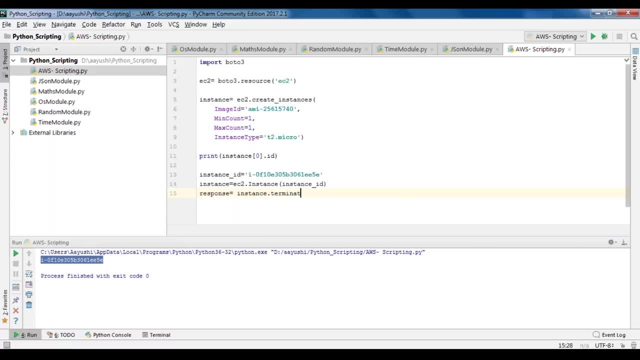 So I'll just type in instance dot terminate and I'll just print the response. So first of all, let me just comment this part so that the new instance is not being generated. All right, so this is the code for deleting the instance. 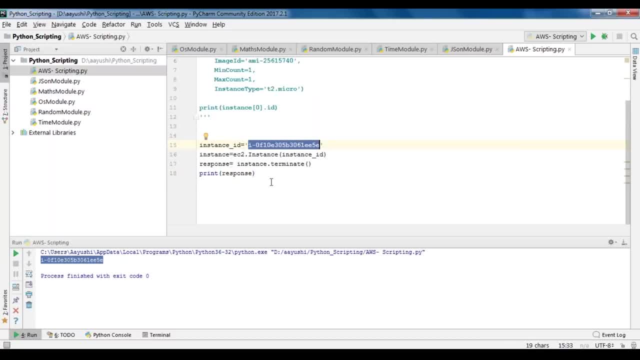 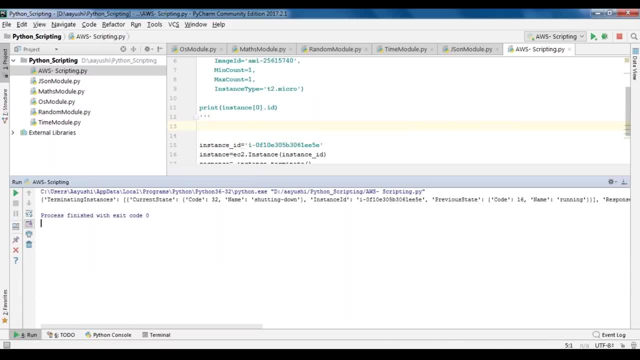 So here I have just specify the instance ID that they need to terminate and I've just print the response. So now let me just run this. So, as you can see here, it has been terminated. We have the current state, then we have the code. 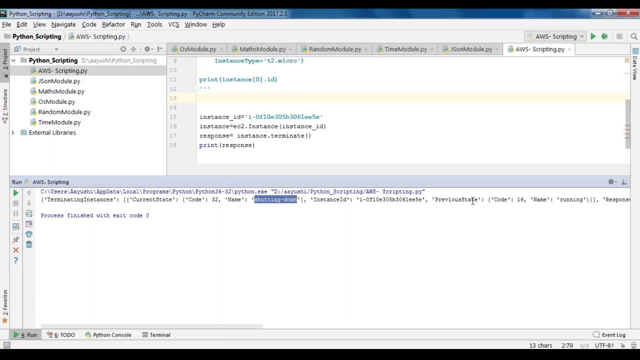 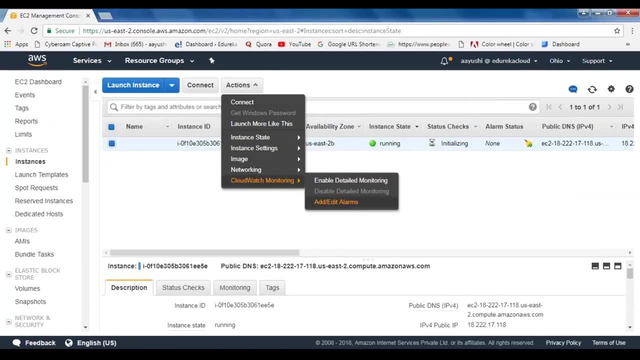 We have the name to shutting down and we have the instance ID. So here it is also telling me that the previous state was running and now it has been changed to shutting down. So let me just go to my console and let us see whether here we have changes or not. 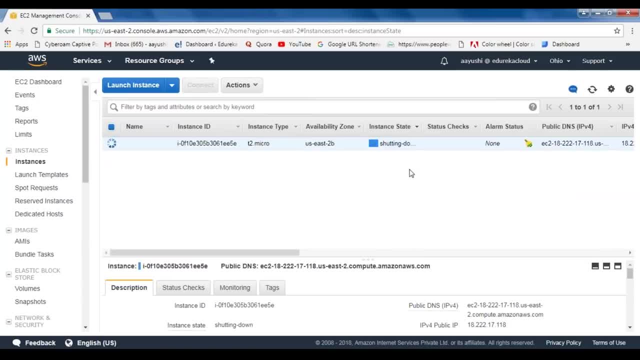 So let me just refresh it. So here, as you can see, it has been shutting down, So now just wait for a few seconds and it will be terminated. So, as you can see here, my instance has been terminated without manually going to the actions. 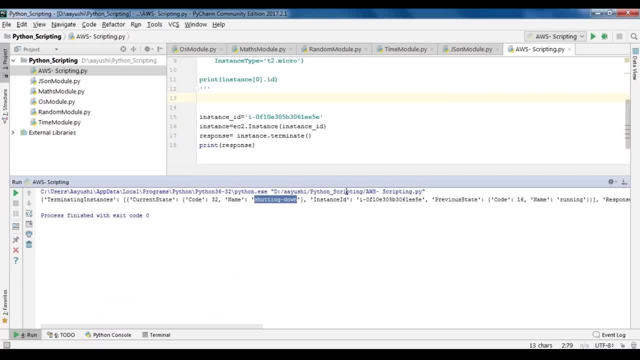 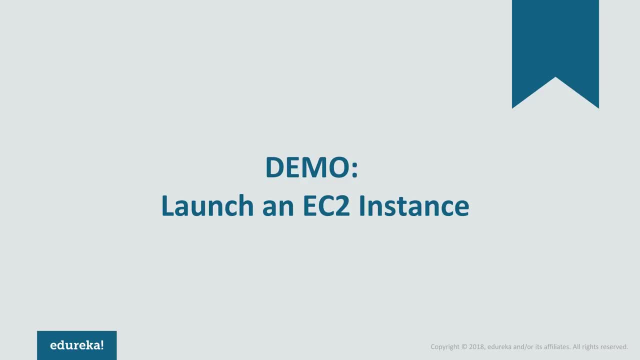 and then clicking it over here, So it can simply write the python codes And it will indeed do the same task for you. So isn't this easy, guys. now let me go back to my presentation and let's see what is my next task. 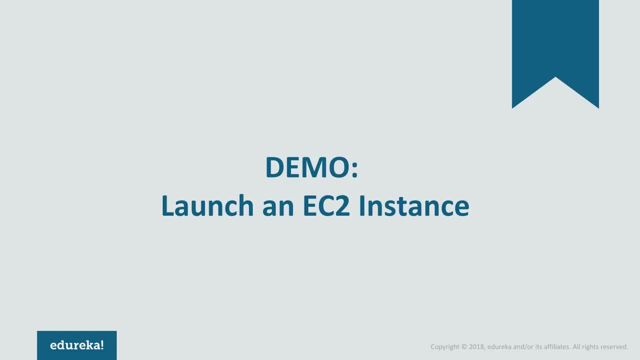 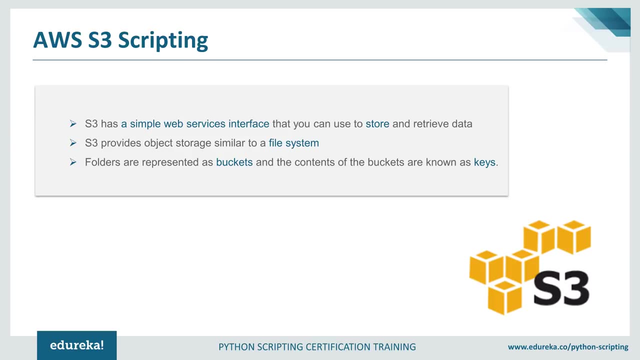 So here I have just launched an ec2 instance and then we have terminated the state as well. moving ahead, Let us understand AWS S3.. So AWS S3 is a simple storage which is offered by AWS, So it's basically a web service interface. 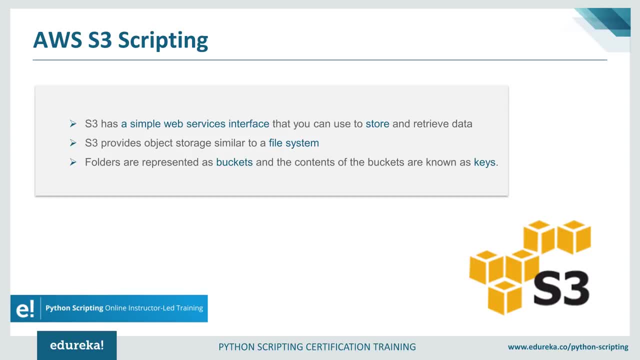 that can be used to store and retrieve the data. So S3 basically stands for your simple storage service, which is a storage for the internet. So S3 provides object storage, which is similar to your file system, wherein the folders are represented as buckets. 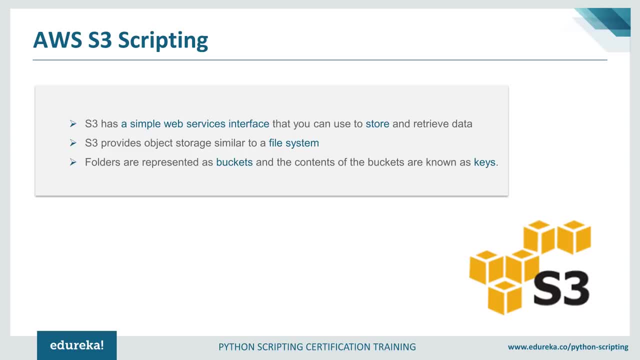 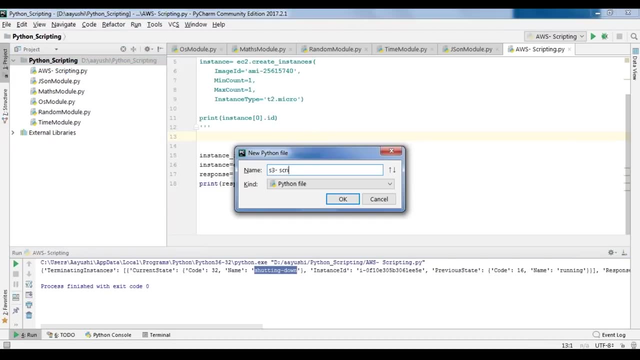 and the content of the buckets are known as the keys. So now let us move ahead and launch a S3 bucket as well. So now let me create a new file, Let's say S3 scripting. So first of all, I need to import my boto module. 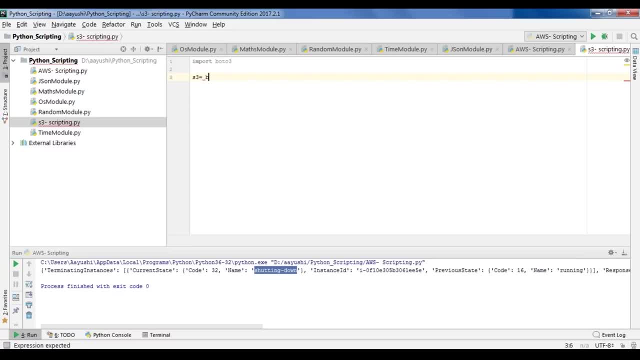 So now what I'll be doing. I'll be creating a S3 storage, So I'll be typing in S3, boto3.resource, the same thing that we have done for ec2.. So, inspired this, I'm just typing in S3.. Now let me go back to my AWS console. 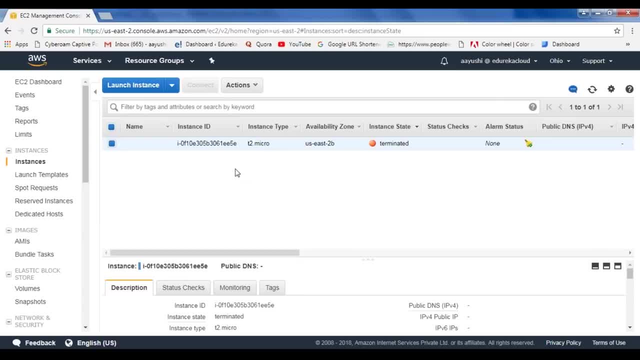 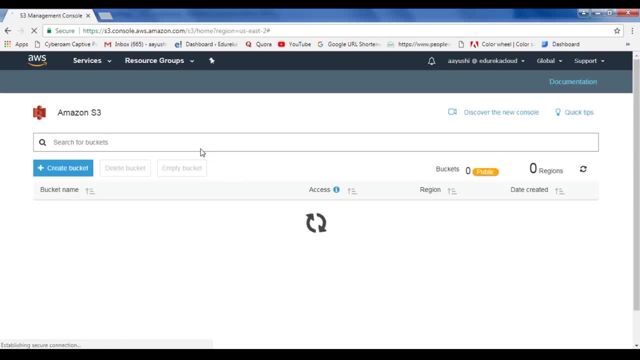 and let's see where this history is present and how can you manually create an S3 bucket. So I'll just go to my services and go in my storage S3.. So, as you can see here, I have a button over here which says create bucket. 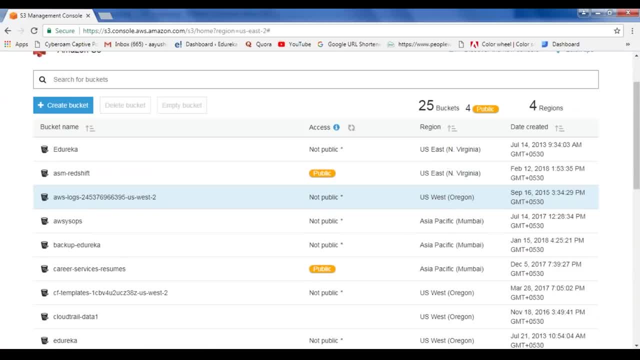 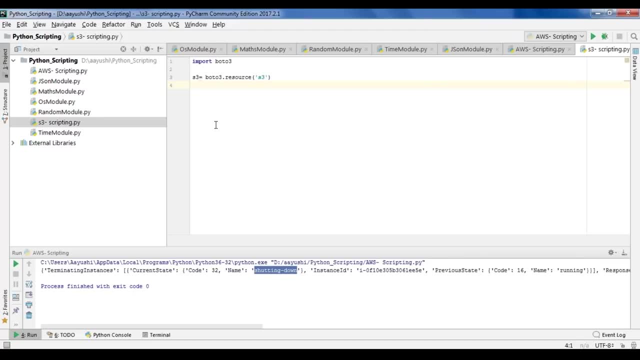 so you can manually go and create a bucket from here. And these are the buckets that have been stored in my account. Now what I'll be doing: I'll be writing a Python script So as to create a S3 bucket automatically for me. 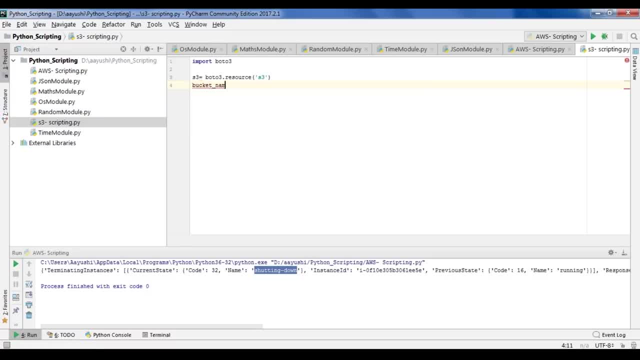 so I'll just type in, let's say, the name of the bucket. So I'll type in bucket name and I specify a name- Let's say bucket one- and I'll try some try-catch to it. So I'll say: response equals to S3, not create bucket. 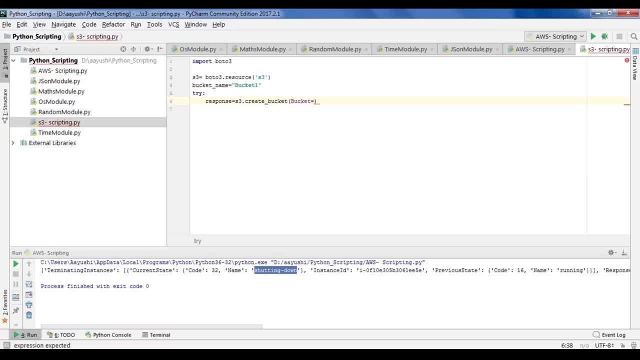 Wherein I'll pass on the bucket name. So I'll say bucket is equals to my bucket name, which is bucket one. Then I'll just pass the configuration, So I'll say create bucket configuration And I'll set some attributes to it. 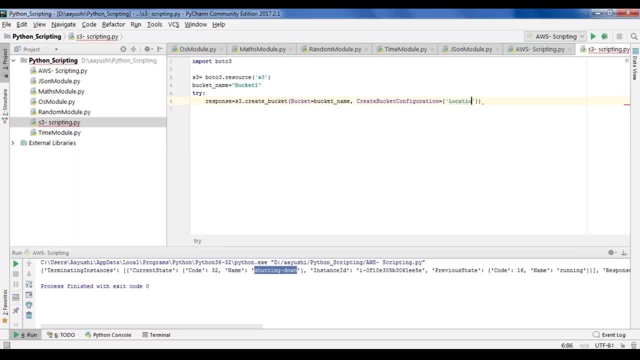 So I'll be giving in the first attribute, that is, location constraint, And I specify the location. So remember, guys, when you were configuring your AWS account, they gave you an option to fill in the access key. So there also, they ask you for the default location. 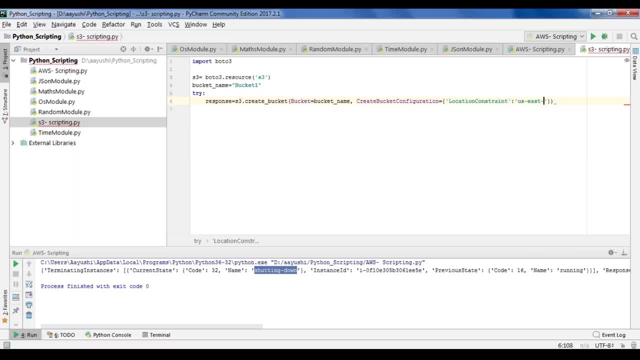 So there, I didn't change any. so I have the default location as US East 2 and here I'll just print my response. Then I'll be just typing in the except- that is the exception, except exception as error, and just print the error if any error comes. so now let me just run this code. 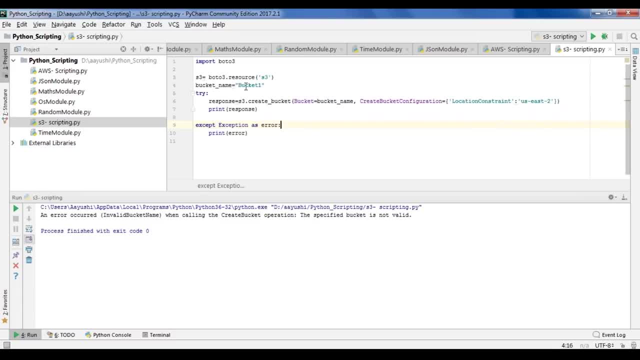 All right. so here it's giving me an error, that invalid bucket name, or it's why I'll just change This bucket name. Let's say, I use she bucket, So I'll just run this code now. So, as you can see here, 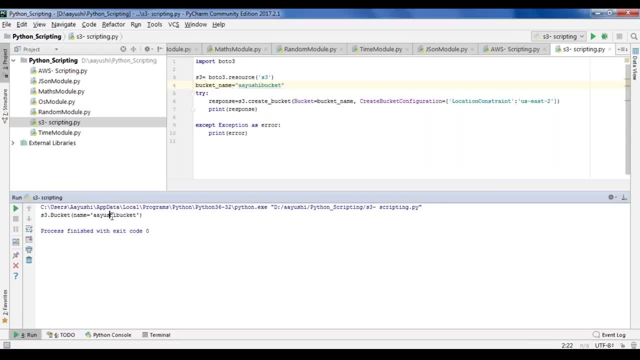 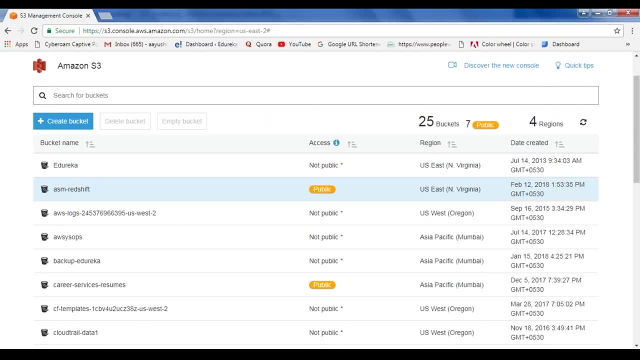 I have the response which says s3 bucket and with the name I use, she bucket. So now let me go back to my AWS console and let's see whether the bucket has been created here or not. So here, as you can see, I don't have any bucket with this name. 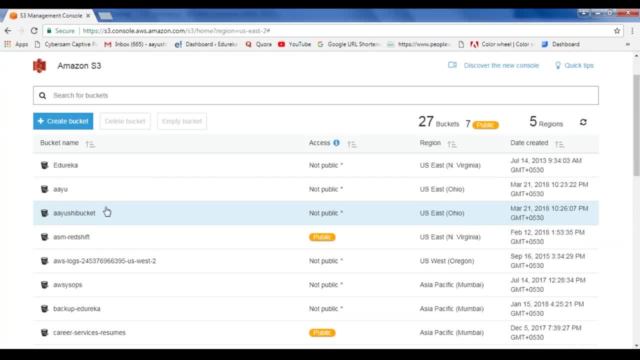 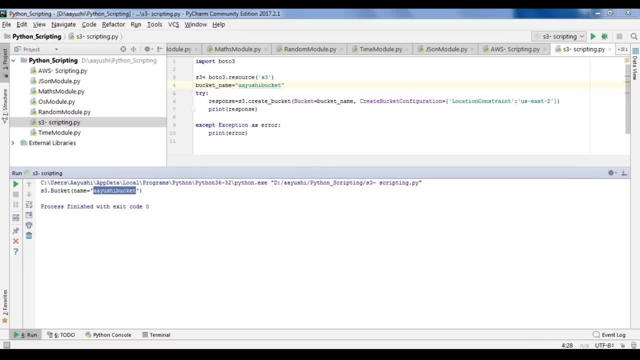 but now let me just refresh it. So now, as you can see, my S3 bucket has been created. So, guys, this is how we can write simple codes and implement a lot of things by using Python. So now let us go back to my presentation. 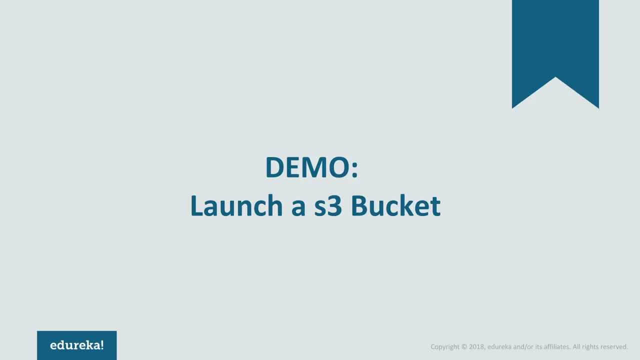 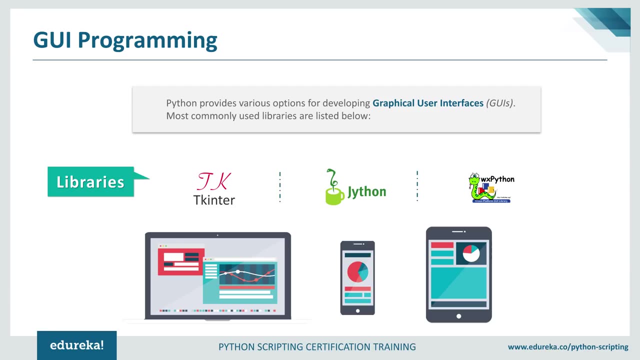 and let's see what is the next task. So here we have successfully launched an S3 bucket. next, Let us move on to a last topic, which is the GUI programming. Python provides a various options for developing your GUI's, which is nothing but your graphical user interfaces. 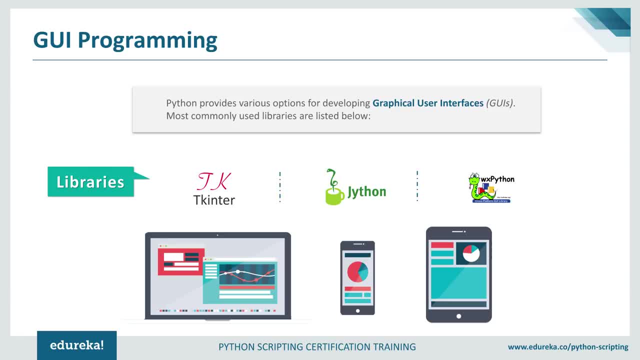 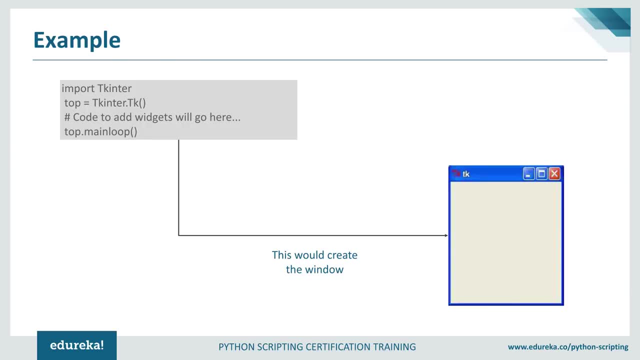 So many libraries which are being commonly used are Tkinter. then we have Jython, we have WXPython, So let us just create a GUI using Tkinter. So here this is my library, which is called as Tkinter, And this is a simple code. 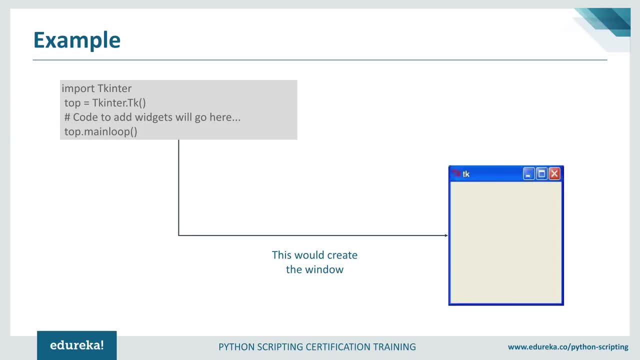 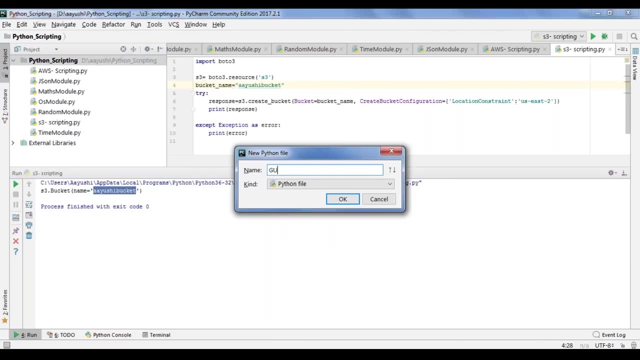 wherein you will just generate a window. So now let me go back to my PyCharm and let us see how Tkinter works. So here I'll be creating a new file, Let's say GUI programming, And over here I'll be first importing Tkinter. 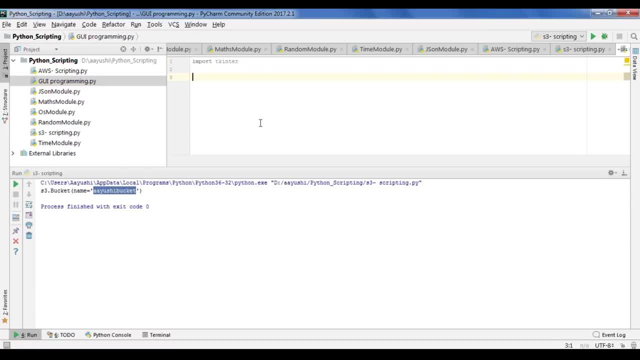 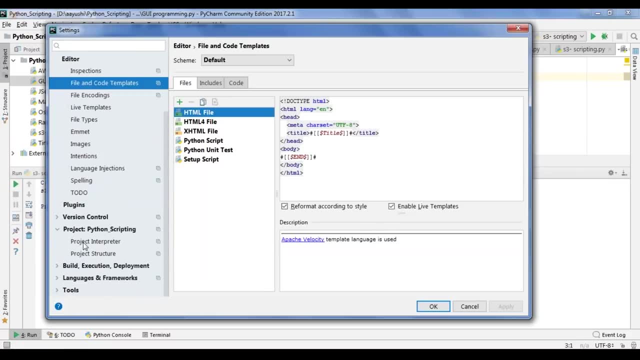 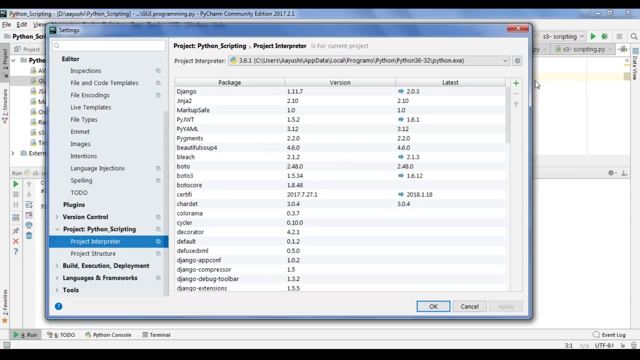 So I'll say import Tkinter. You can also import these libraries by going to file, just going to settings, And under the project, just go to the project interpreter And over here you can add the packages from here. So you just need to click on this plus icon. 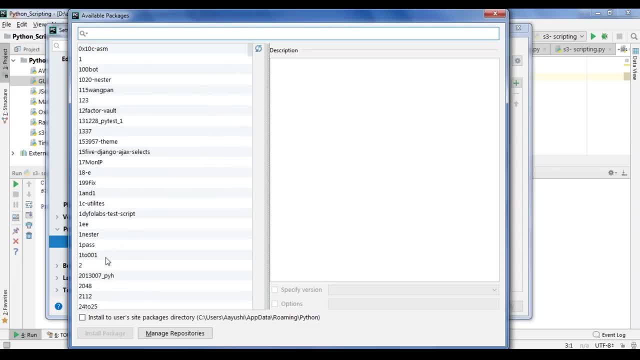 and the list of packages will be displayed to you. So from here you can import any package. So now we recently we have talked about Boto, So we can just type in Boto 3 and here Boto 3 is present. So we just click it on here and install the package. 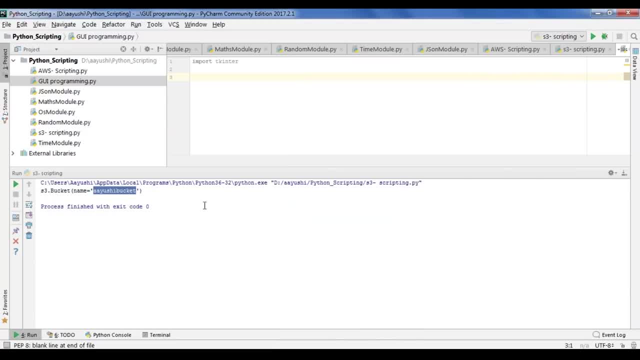 So, guys, if you have any issues or any problems regarding the code, comment below the video and I'll be happy to help you with the same. So now let us just come back to a program and let's implement Tkinter. so Tkinter is available for all the versions of Python. 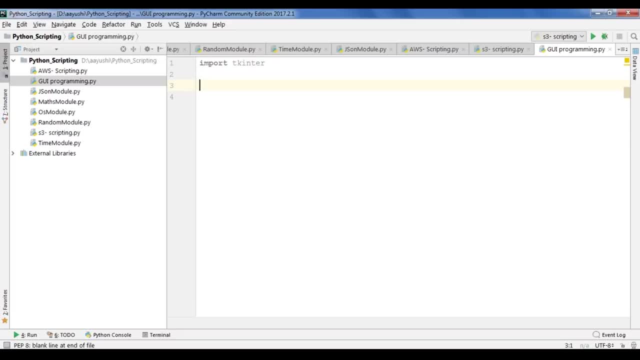 Now, first of all, let us check whether this Tkinter is working or not. So for that, let me just type in Tkinter dot underscore test and now just run this. So here, as you can see, I have this pop-up coming up, which gives me this window with two buttons. 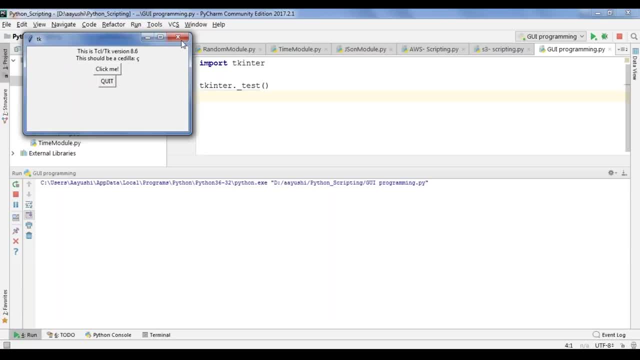 which is click me and quit. So this proves me that my Tkinter is successfully installed. Now what I'll do? and remove this line and I'll be creating a blank window wherein we have a close sign, minimize and all that stuff. So for that, what I need to do, 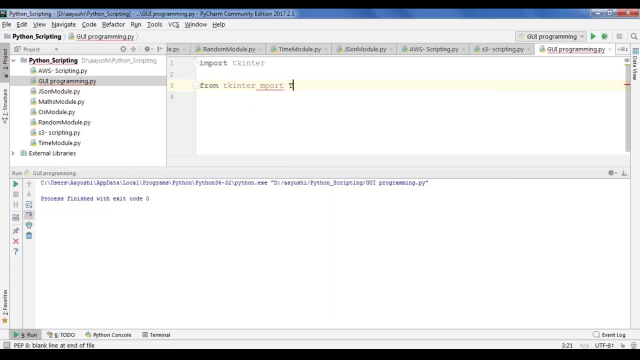 I need to type in: from Tkinter import TK. So now let us enter some dummy text to it for that. Let me just remove this. So here I have just import TK, So you can also import from Tkinter import TK. Or you can simply write in: from Tkinter import star. 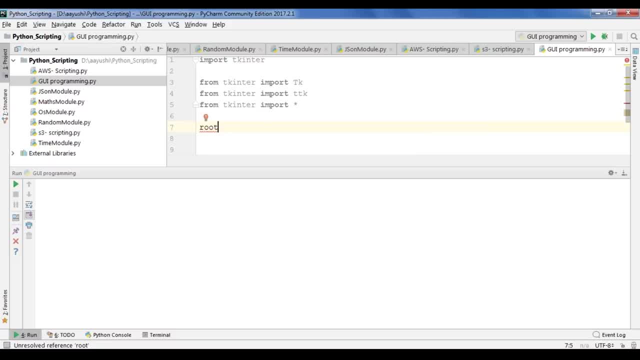 Now what I'll be doing. I'll be creating an object. or you can say: let's say it's named as root. So I'll say root is equals to TK. So here the root is basically a class, which is the main window that surrounds our interface. 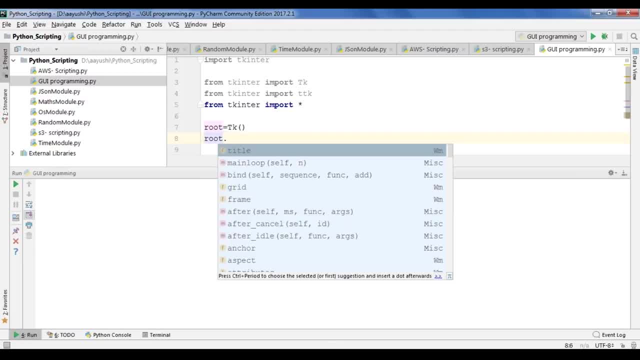 Then, once we have done that, we'll give a title to this. So we'll say root dot title and inside this I'll be writing some text. So let's say: first GUI using Python, Next I'll be adding some button as well. So for that I'll be just typing in TTK dot button. 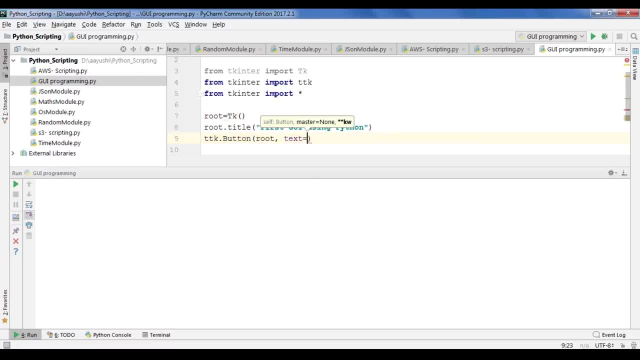 and I'll be passing in the root and a text to this button. So let's say I want the text as hello at Eureka and I set a grid to it. So grid is nothing but a simple layout manager which will help you to structure different components. 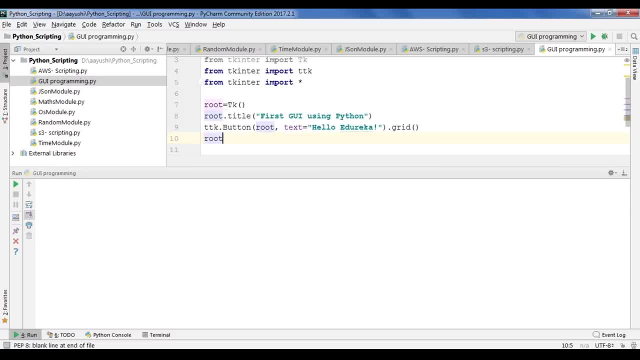 or the widgets inside the window. next, I'll just close this loop. So I'll just type in root dot main loop. So, as I've already explained you that this window will keep on turning until unless you decide to close it. So here I just run this code. 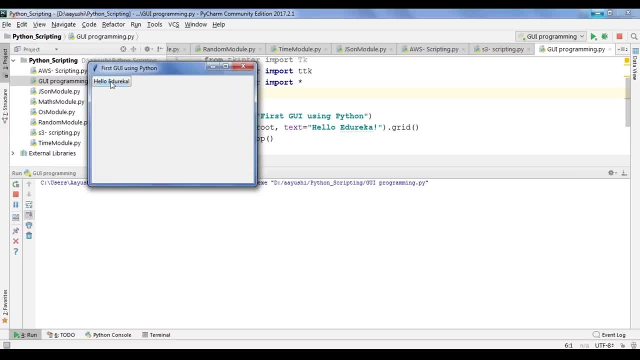 and, as you can see here, I have a title to this window as well as a button. So now let us see the different components which can be used in a GUI application. Let me go back to my presentation once. So I have discussed that- how you can create a window. next, 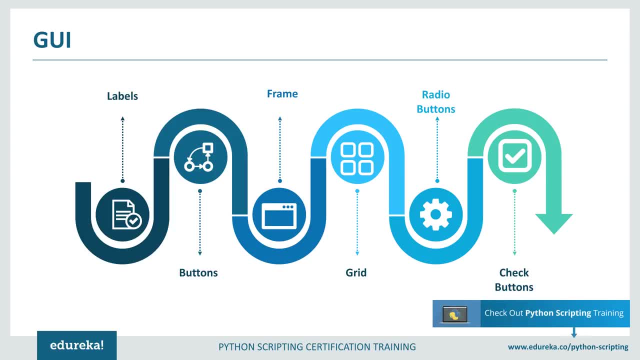 What are the different components in a GUI? So these are the basic components which are present in a GUI application. So first we'll start off with the labels- how we can add a label. then we'll see how you can create a button. So we have already seen how you can create a button. 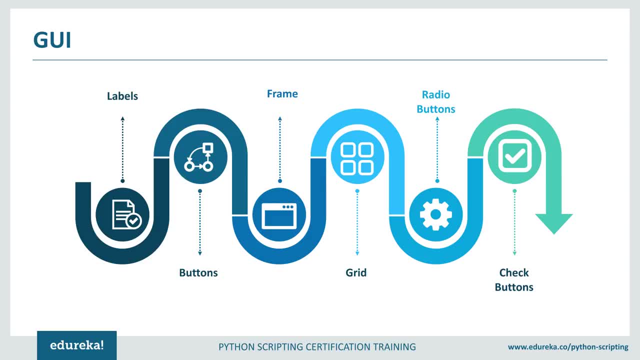 Then what we'll be doing will be creating a frame wherein we have the label as well as buttons. then we'll go into the details of grid, where is geometry manager, and tells how you can Define all the components within a window. then we'll be talking about the radio buttons. 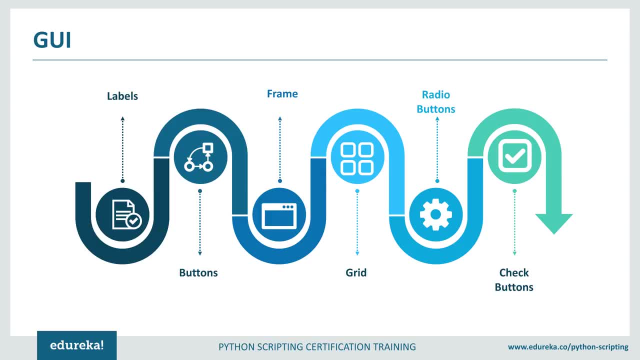 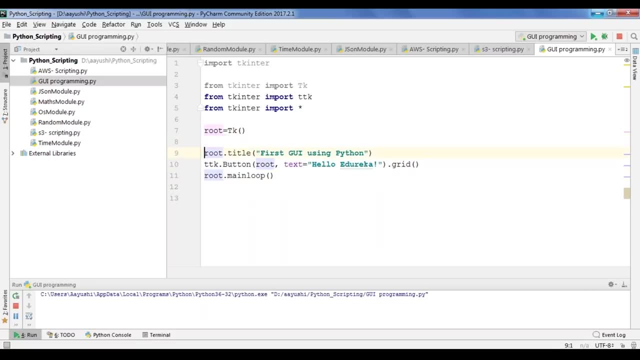 and check buttons as well. So let me go back to my pie charm, and it is implement these. so till now, we have just given a title and a button to it. Now let us create a frame. So for that, let me first comment this code. 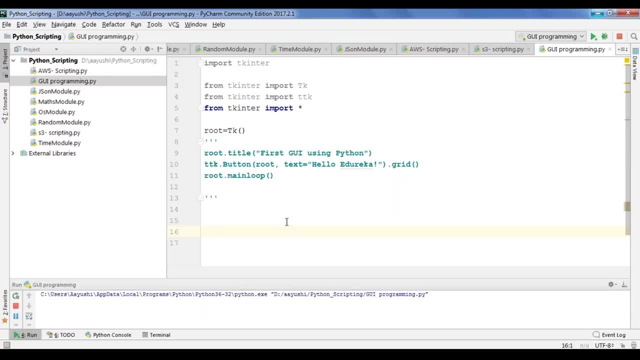 All right. So now let us create a frame. So frame is nothing but a widget which surrounds the other widgets. So I'll just type in frame and I'll say frame and pass in: the root is nothing which has DK, or you can say: peek into next. 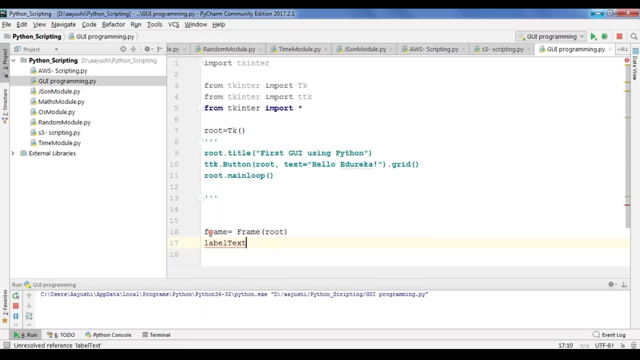 I'm creating a label text, So let's say label text and say string where. so over here I am just defining this, but we'll be changing the text for the label components. So now let's create a label and buttons with some attributes. 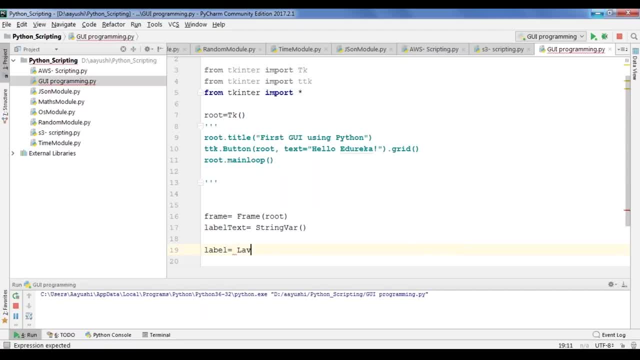 So first of all I'll create a label. So let's say label, It is equals to label and it should be inside a frame. So I'll just type in frame and then I have text variable equals to my label text. So here this label text will be changing this afterwards. 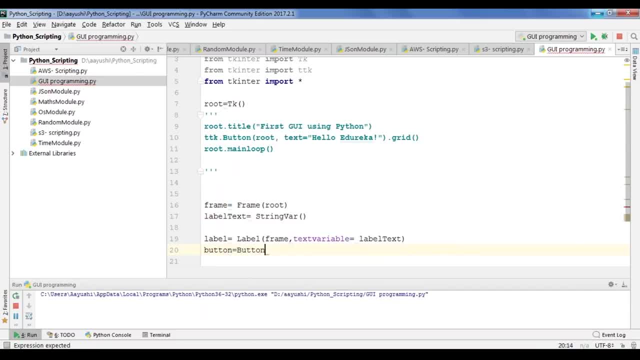 Now let's have a button, So I'll say button, which should be placed inside a frame, and we have a text. Let's say: hey, I am a button. Then let us just change the text inside the label component. So for that, what you can do, you can type in label text: 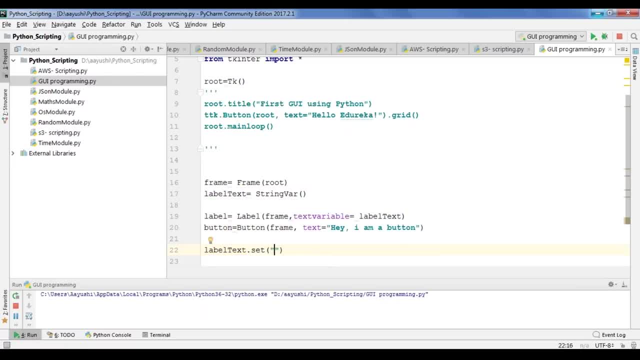 Dot set inside this. I can just change the text. Let's say I want type in: hey, what's up, And then what I'll be doing: IP just using a pack. so pack is nothing, but it's geometry manager which defines how all components are arranged inside the window. 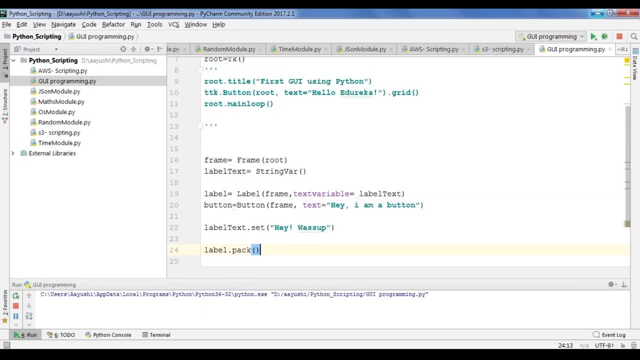 or you can say it's used to position the widgets inside a label, So I have just packed my label. then what I need to do, I need to pack my button as well. So I say button dot pack, I'll pack my frame as well. 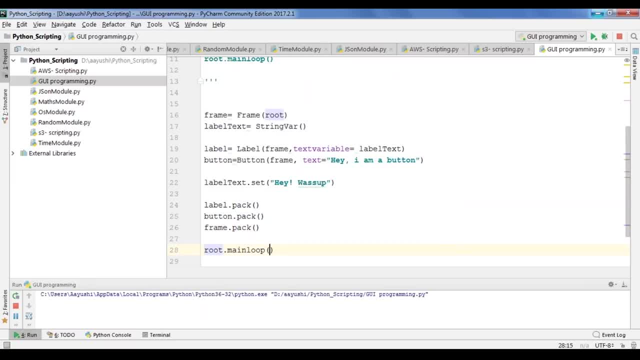 And finally, I'll be just closing the loop, So I'll say root dot main loop and I'll just run this. Let me just expand this a bit. So, as you can see here, I have a label and I have a button and, as you can see here, my label text has been changed as well. 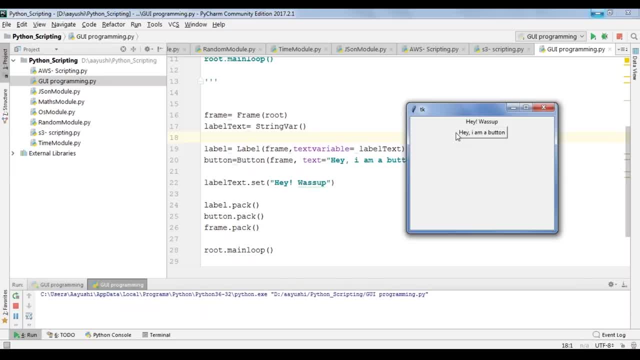 Now you can also have various attributes to this DOI application. You can also fill the directions to it. You can mention whether it should be stretched among the x-axis or y-axis, or it should be stretched from both of them, and there are a lot of things you can do it. 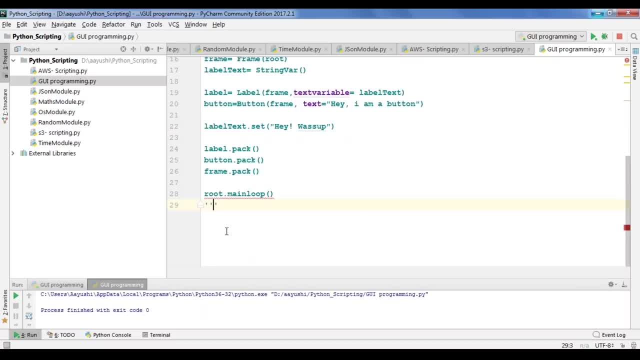 So here let me just implement some of the attributes to it. So I have just commented all the buff code and inside this I'll be having one label. So I'll say: label: it should be inside a frame. Then I have a text, Let's say say: and I just simply pack this next. 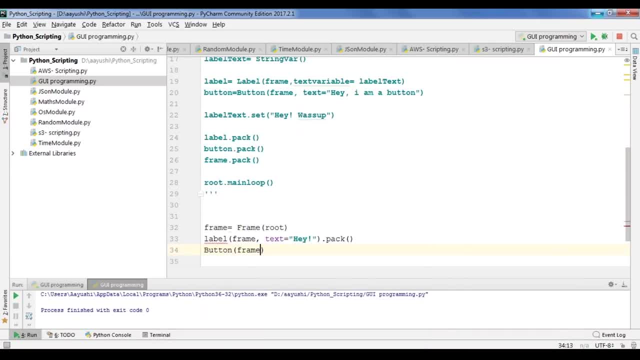 I have a button which is again inside a frame. I have a text to it. So let's say text is b1 and then I just pack this. now, when I pack this, I can mention the attributes, such as I'll say that it should be in the left-hand side, then specify the field. 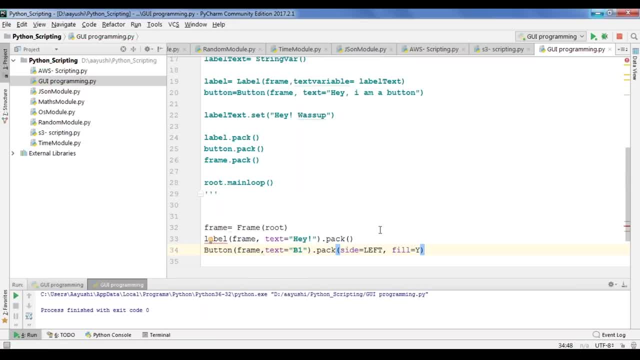 which should be filled in the y-direction. So this field direction is basically, it will tell you how they will be stretched. So it will be stretched along the x-axis or y-axis, or x, y-axis or both of them. Similarly, you can have many more buttons like that. 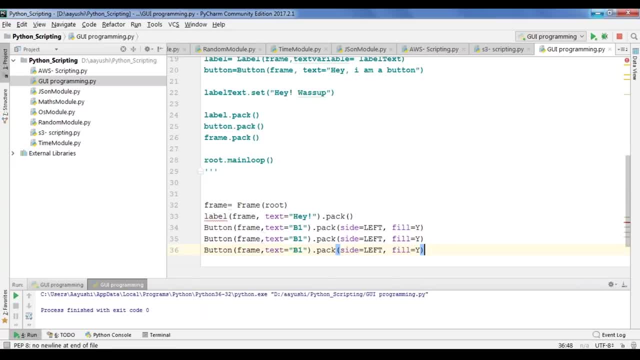 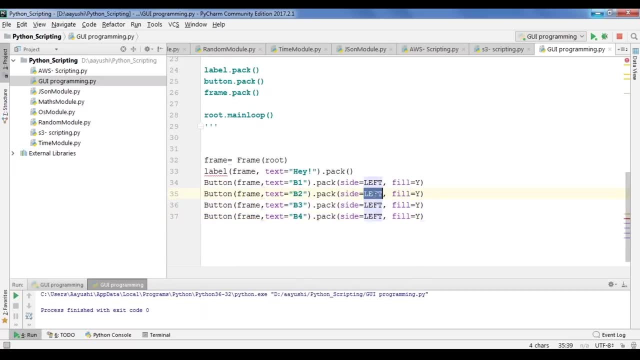 So I'll just copy this line and I'll just paste it over here, All right, and I just change the text to it, So I'll say b2, b3, b4, and then I just change the side as well, So you can distinguish between the different buttons. 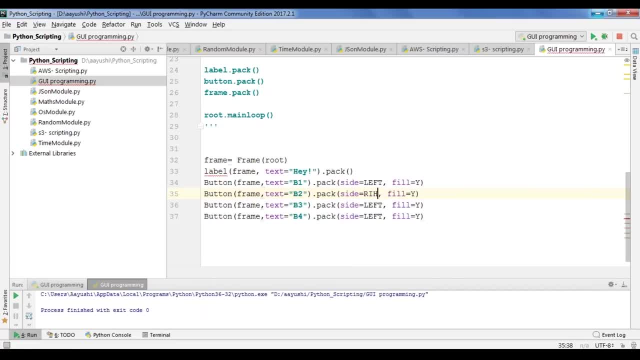 Let's say it's right now- Remember guys, it should be in uppercase. So I'll say right, then here I'll say it should be top, and let's say it be left only, and then I'll be changed, Changing the direction also. 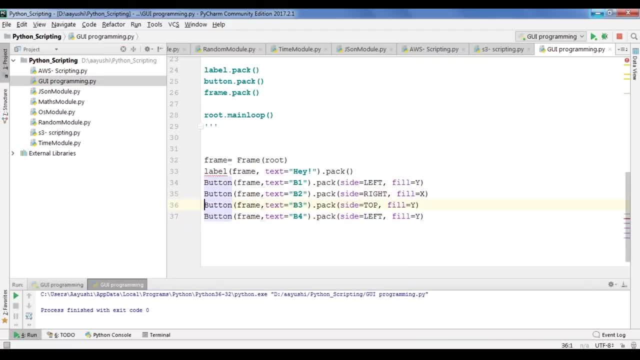 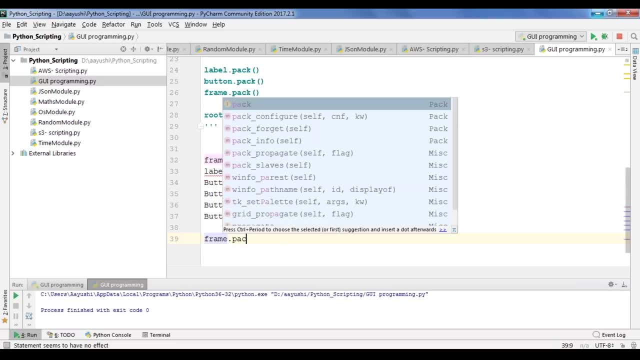 So I'll say it should be in x-direction or should be stretch among along the x-axis, and this should be Y again. So now what I'll be doing: I'll just pack the frame and I just close the loop. Now let me just run this. 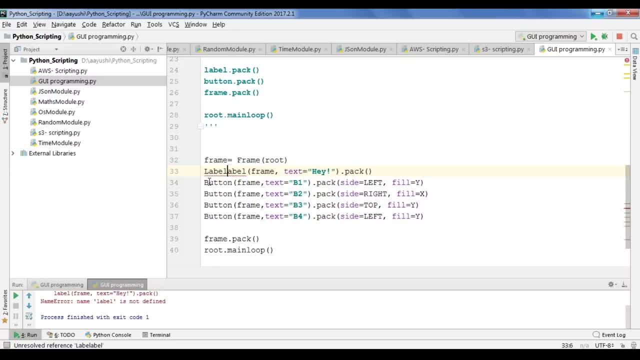 All right, So here my label should be capital. All right, Now let me just run this. So now, as you can see, my buttons has been arranged beautifully. So here my b1.. It has been set to left, So here it has been aligned left. 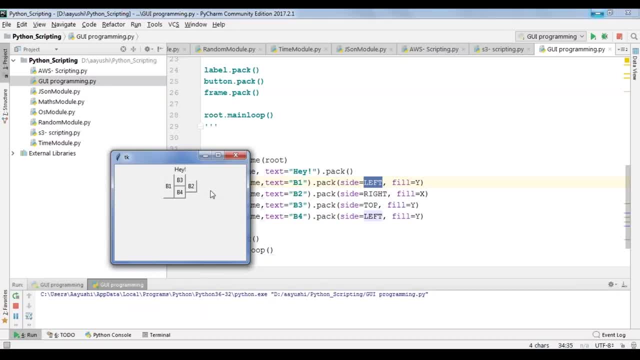 Then my b2 is been aligned right, So it's again in the right hand side and it's in the x-direction. Similarly, your b3 and b4 are aligned top and left, along with the directions. So that is how you can set various attributes. 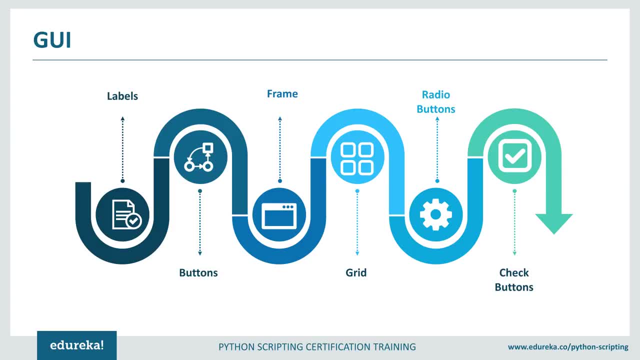 to your GIA application. Next, Let me go back to the presentation and let's see what all are left. So we have learned how to create labels, then buttons, then how to create a frame in which labels and buttons are packed. then Let us see how you can create a grid. 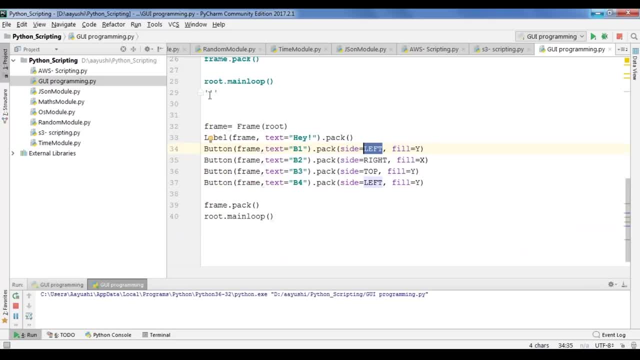 So now let me go back to my pie charm and let's implement grade as well. So again, I just comment the whole code for now. So now what I'll be doing. I'll be first having some labels, So let's say I'll specify a label inside a root. 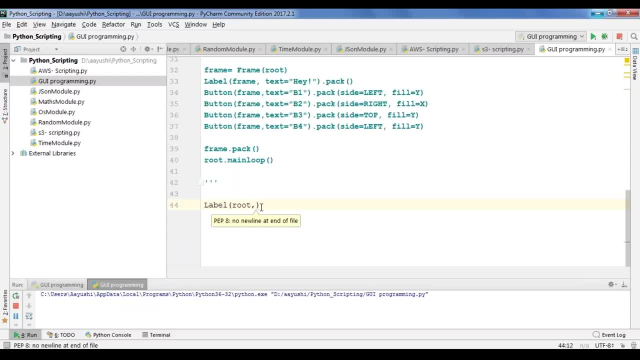 and I have already mentioned, root is equals to TK, So I'll be giving some text to it. So let's say I want text, Let's say name and I want the grid to it. So create is nothing but a geometry manager which will basically help you to structure different components. 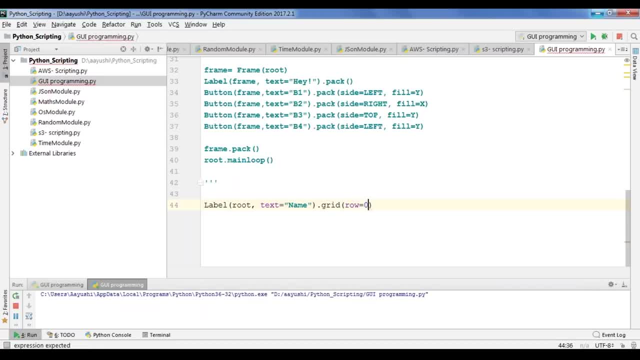 or the widgets inside the window. So here you can mention the row and remember, guys, your index will always start from 0. then you can mention the column. Let's say my column is also 0. then I have sticky and I can give some direction. 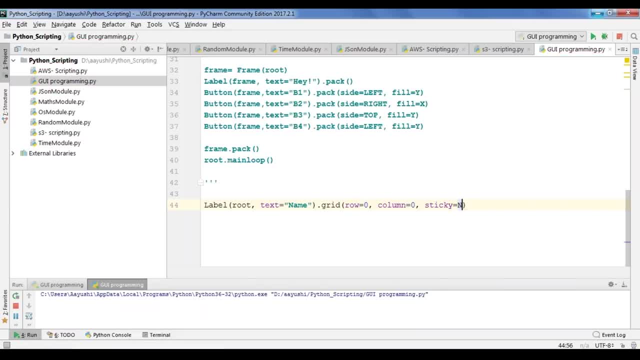 Let's say not so sticky is nothing but how your widget can expand and in which direction. so you have very directions such as North. you can type in East, you can type in W for West and you can specify according to your needs. So I've just created one label. now what I'll do, 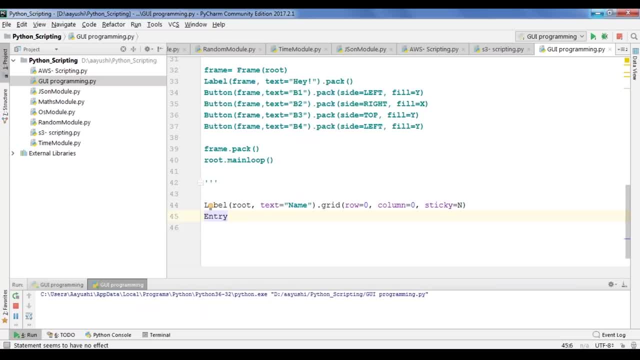 I'll create one entry box wherein the user can take input. So I'll type in entry and pass the root. then I can specify the width. Let's say it is 50 dot grid and I'll again mention the row to it. Let's say row is equals to 0 and let's say column is equals to 1. 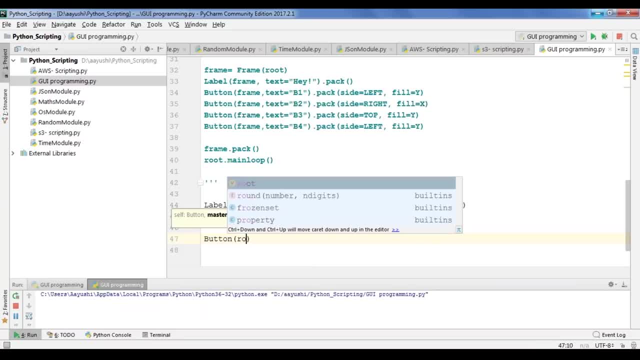 and I'll have one more button- Let's say button- and I'll say it's in root, And I'll have a text which says submit and I'll pass the grid functionality which is in the row 0 and column Let's say 5, and I'll just close this loop. 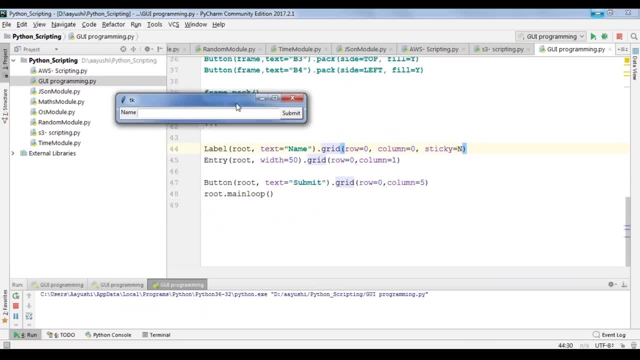 Now let me just run this code. So, as you can see, here I have one label which is named as name, then I have an entry box, So here you can type in any name. Let's say, I want to type in ABC and I have a submit button. 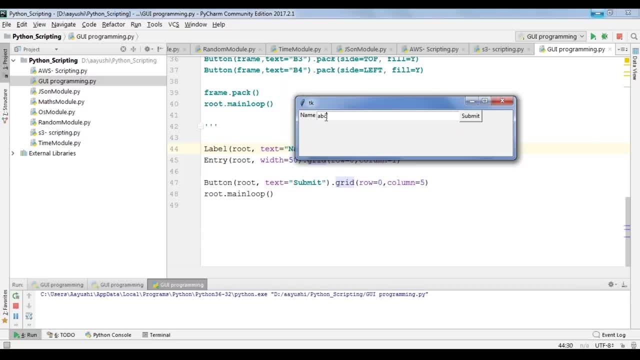 So here the submit button will not do anything, but you can actually save the entry box, So entries to a SQL database or anything you like. So we'll be discussing the SQL databases and all those stuff in our upcoming sessions, But in today's sessions let us focus on GOI. 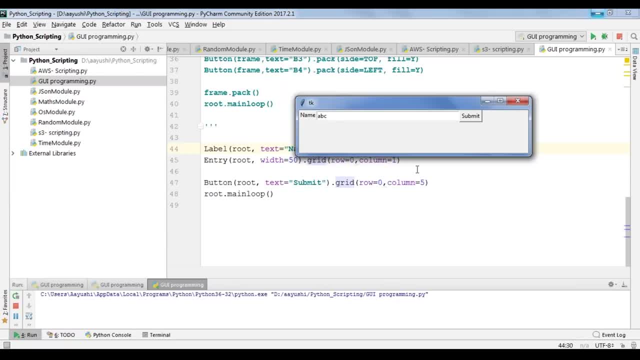 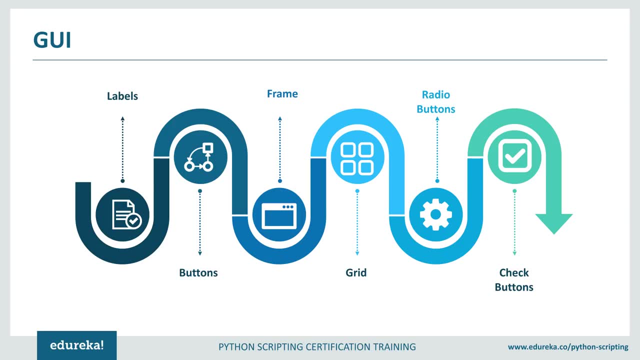 Also, if you have any doubts, you can just let me know in the comment section and we will be replying you as soon as possible. All right, so this is done. So now let me go back to my presentation and let's see what else is left. 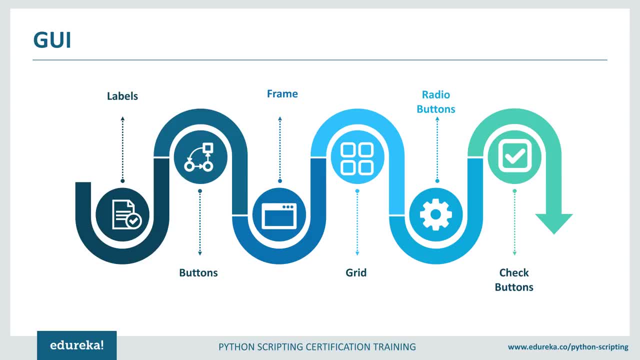 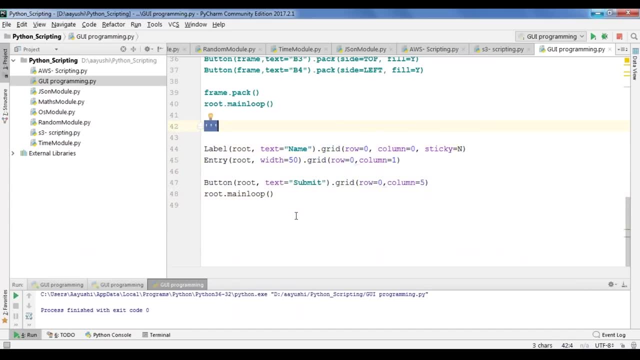 So we have covered the various attributes of grid. Now let us talk about the radio buttons and check button. So let me go back to a pie charm. Let's see How can you add a radio button and check buttons to your code. 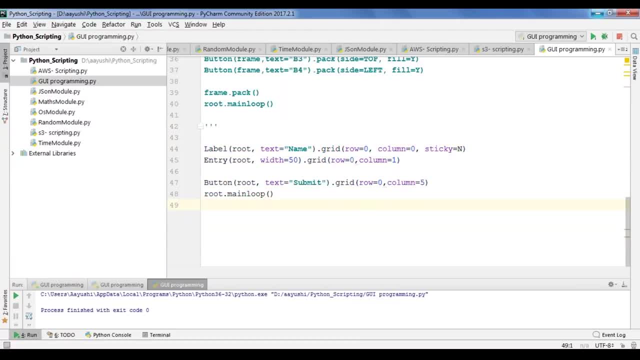 So now what I'll do. I have a label, I have an entry box and I have a button. So next what I'll be doing? I'll be creating one more label. Let's say I'll just try it over here. Let's say I have one more label inside a root. 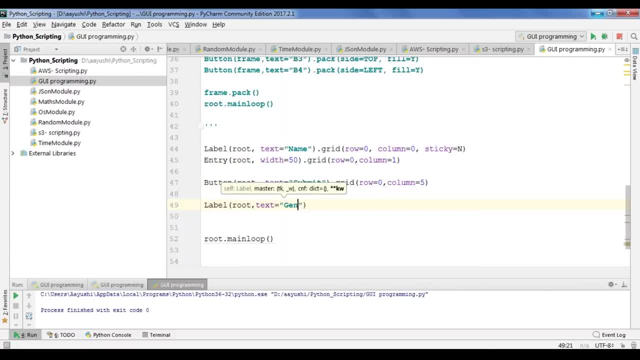 and I want text as gender. I specify the grid functionality to it. So I say Joe is equals to one, then column is equals to 0 and sticky to North. or you can say n. then what I'll be doing? I'll be creating a radio button. 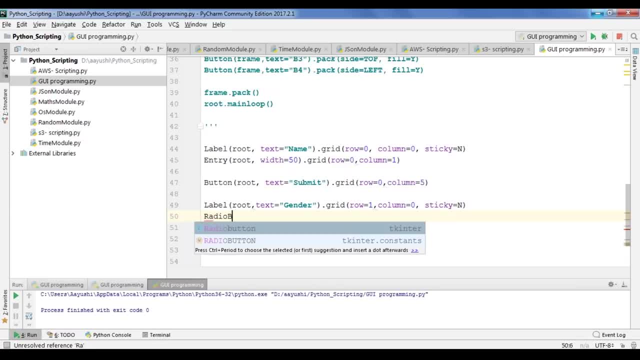 So for radio button, what you need to do? you just need to type in radio button inside a root which has the text: Let's say if that is for female, and I specify the value to it. Let's say one. so this will basically ensures. 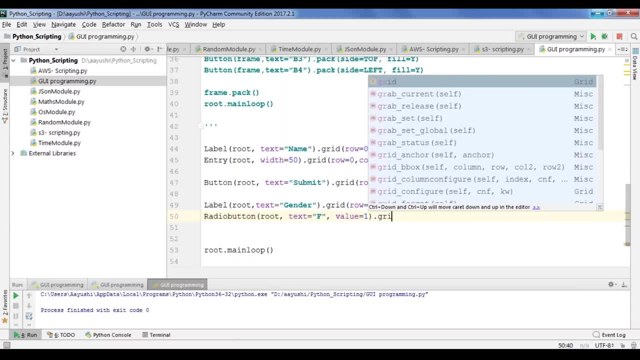 that which radio button is clicked on next. I'll be just giving the grid, so I'll just copy the same thing from here And I'll change the column value. Let's say it is one now- and I'll have one more radio button where I have the text as M, or you can say mail. 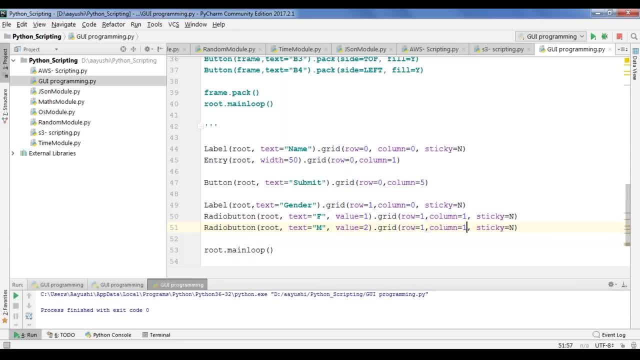 I have a different value to it. Let's say value to it should be in different columns. So I'll specify column 2 and sticky. So now let me just run this. All right. So as you can see, here I have my two radio buttons. 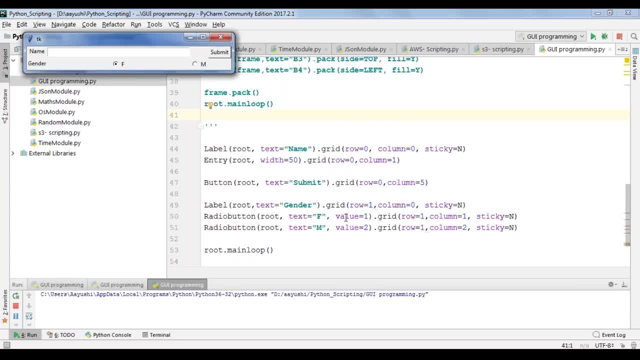 That is female and male, and once you click on this- the value over here that we have given- you can click on these radio buttons. Now let us see how you can implement the check buttons as well. So here I have implemented radio buttons, So check buttons are also very simple. 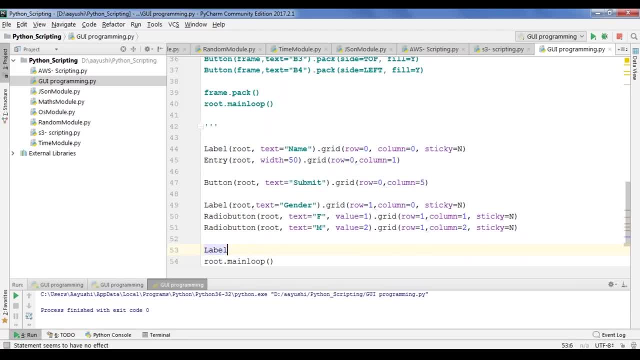 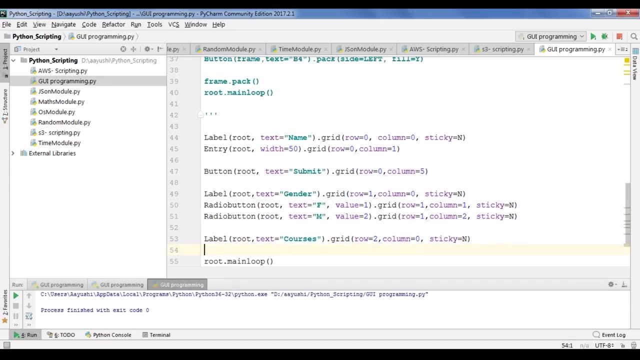 So again for check buttons, I'll first create a label. So I'll just copy this label line and paste it over here. I'll say the text as courses. It should be in my row too. Column should be 0 and should be sticky towards the north direction next. 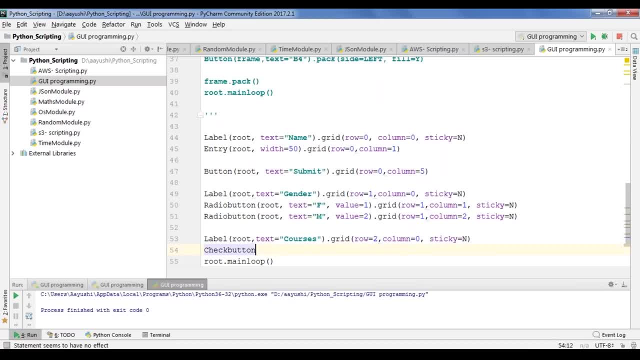 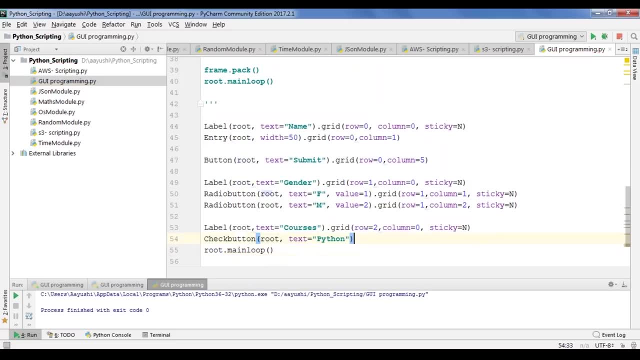 I need a check button. So I'll say check button, It should be inside root and specify a text to it. So let's say I want Python. then I'll mention the grid. Let's say it should be in the row 3, column should be one. 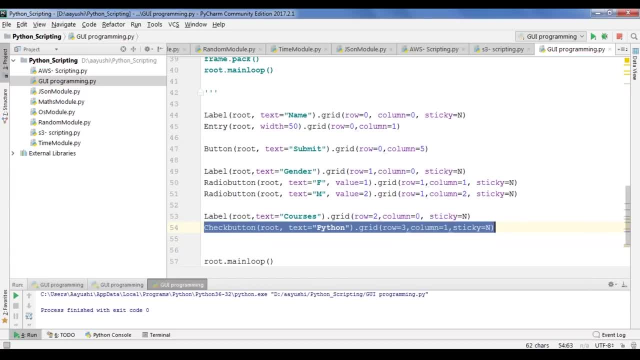 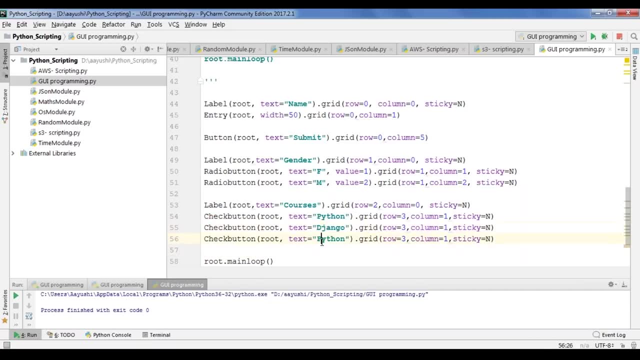 and sticky towards the north direction. Now I'll just copy this line and paste it over here. So now let me just change the course, His name, that say it's Django, then let's say it's, it's fast, which are nothing but the frameworks of python. 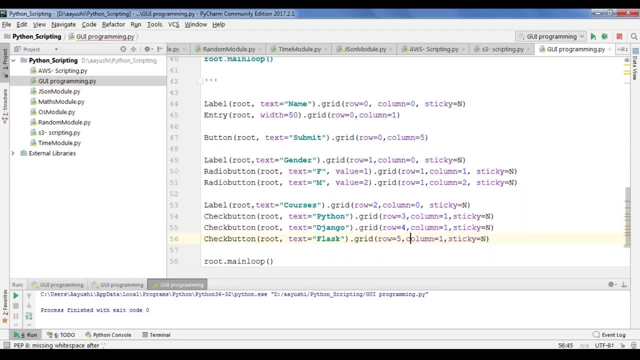 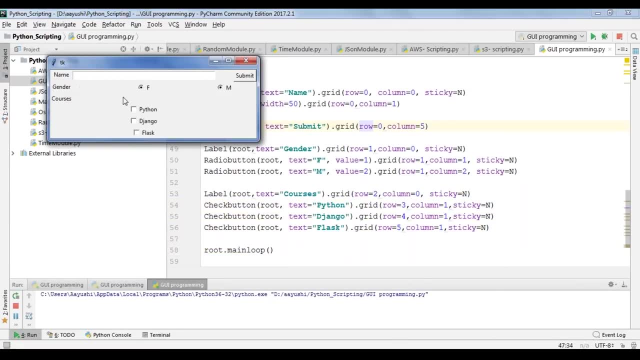 So now I'll just change the rows, that is, 4 and 5, and columns should remain the same only. So now let me just run this code. So, as you can see, here I have the radio buttons and I have the check buttons as well. 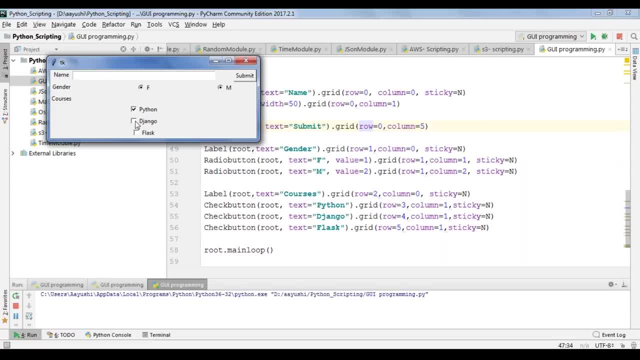 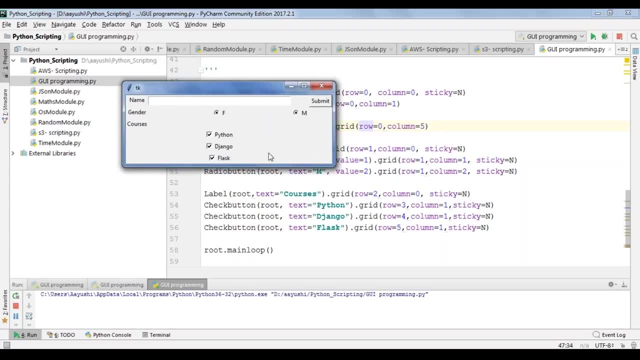 So if I click on python, a check has been displayed. similarly, you can do it for Django and plus, which are nothing but the python frameworks. So, as you can see, here I have created a short UI application which has a name, which has a gender. 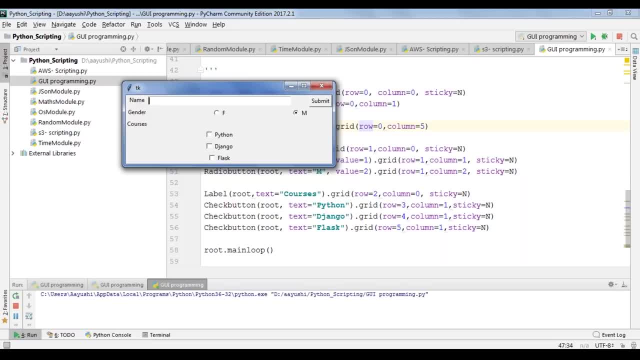 and then you have some courses, or you can say the check buttons and similarly you can create a entire form and just click on submit. So clicking on submit right now It doesn't do anything, but you can do a lot more when you go into details of it. 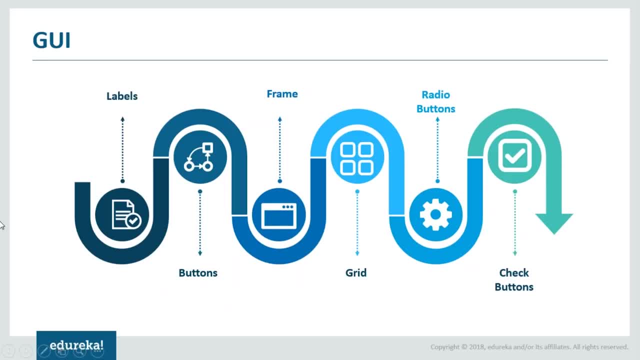 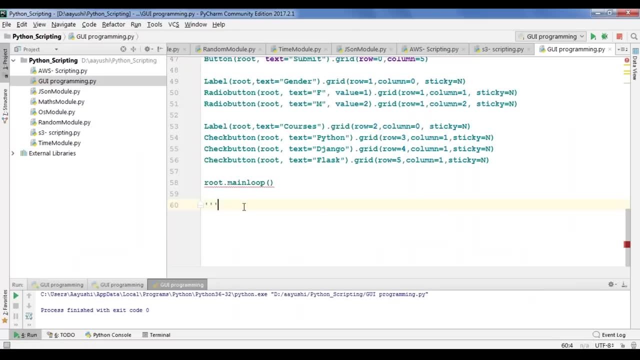 So let me just close it for now. So here I have discussed all these conference, So now let us implement a basic operation using all these. So now let me just comment the whole code and what I'll be doing. I'll be performing some arithmetic operations. 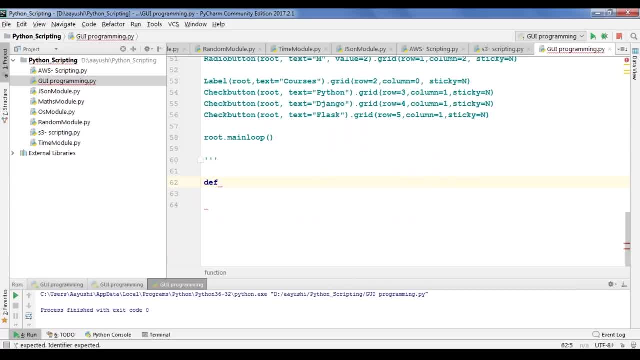 So now what I'll be doing, I'll be first creating a function. So let's say I'll be creating a function. Let's say square. This will basically give me the square of a number. So here I'll be writing an event. 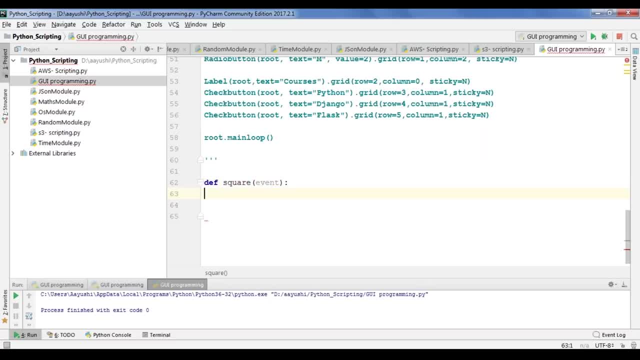 So there, I have just created a function which is square, and inside this I've given an event. now let us first create the interface, and then we'll come back to the logic. So here I'll say: root is equals to TK. Well, it's, I guess, over here. 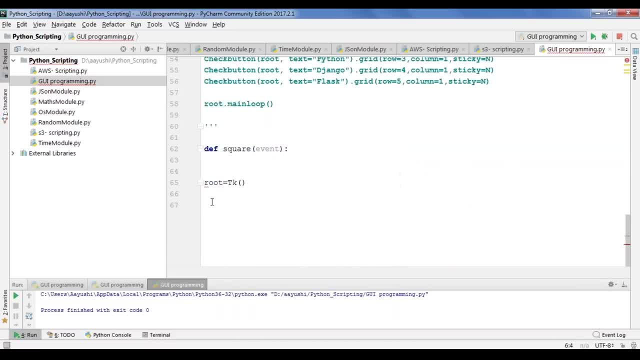 I haven't, So let me just comment from here. All right, so here I'll be. first creating a label, So let me just type in label, then it should be inside a root. I'll give some text to it. So let's say, I want to find the square of a number. 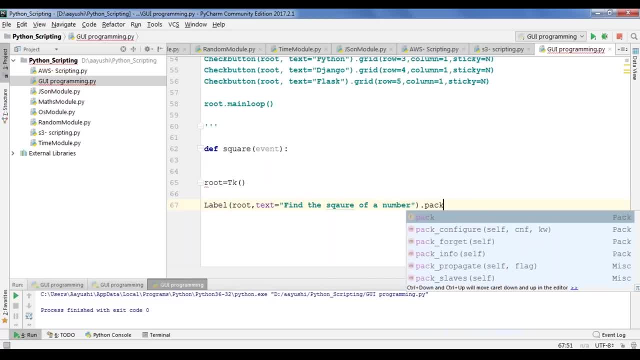 So I just type in that and I'll just pack it next What I'll be doing. I'll be taking an entry of a number, So I'll say number one. I can say number one is equals to entry and I'll pass in the root next. 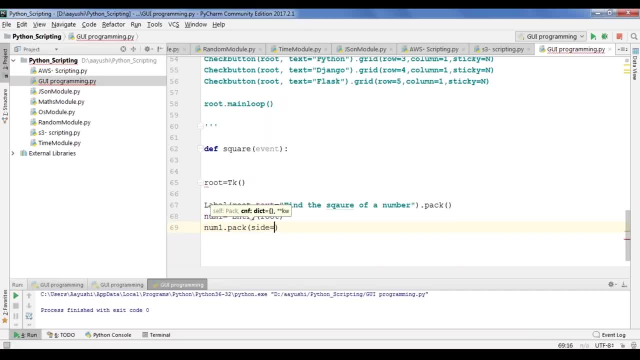 I'll just pack This root and I can give some attribute. Let's say I want to give. it should be aligned to left. next, What I'll be doing, I'll be creating one button, So this should be inside a root and it has a text. 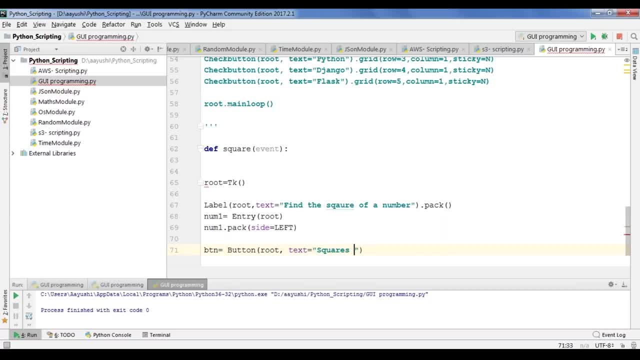 Let's say squares to, and I'll just bind my button. So I'll say button dot, bind, and I'll specify the button. Let's say it's button one, I'll pass on the function that is squared. So what I've done here. 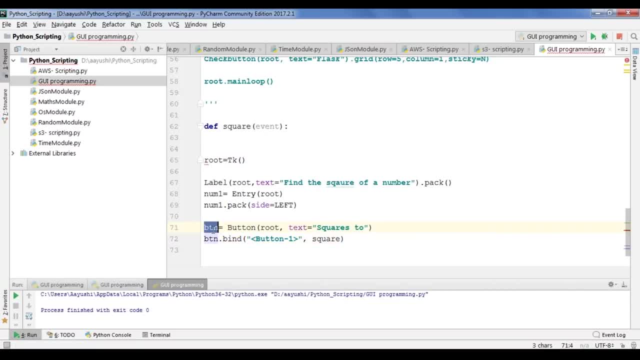 I've just find an event handler to a button which is nothing but BTN. So whenever person enters a number and clicks on button which is equals to squares to, it will just bind to an event listener. So now let me just pack this button as well. 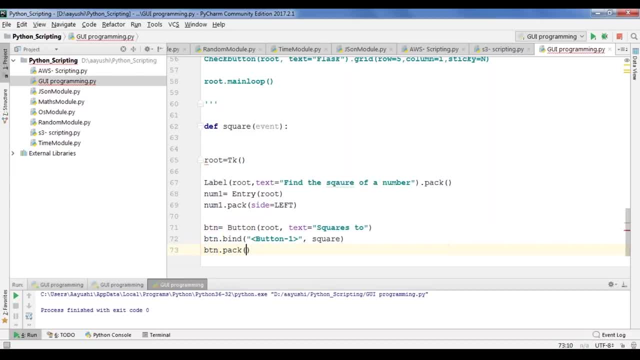 So I'll say button, or you can say BTN dot pack and I'll say side is equals to left. next I'll have one more entry box which gives me the results. I'll save results and I'll have a entry. I'll pass on the truth. 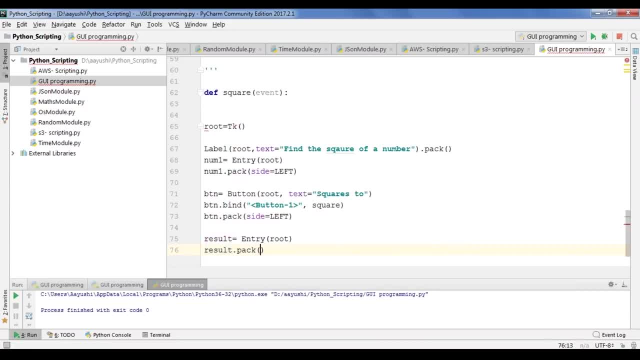 Then I'll be typing in result dot pack and I specify the side as left again And finally I'll be just closing my loop. So now my interface is ready. Now let's go to my method, wherein I will write the logic. 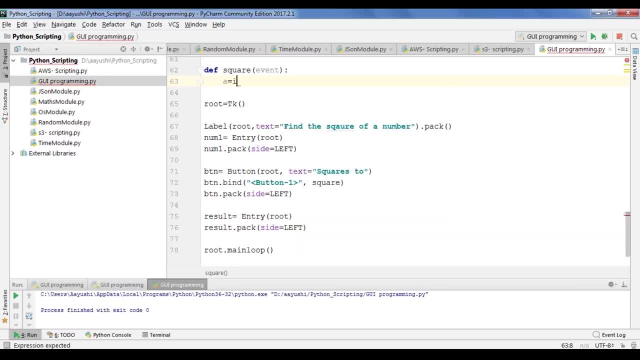 So here what I'll be doing, I'll be first needing the number. So what I'll do, I'll say a int and I'll say num1, dot, get. so this will basically get my number. So next, what I have to do, I have to calculate the square of that number. 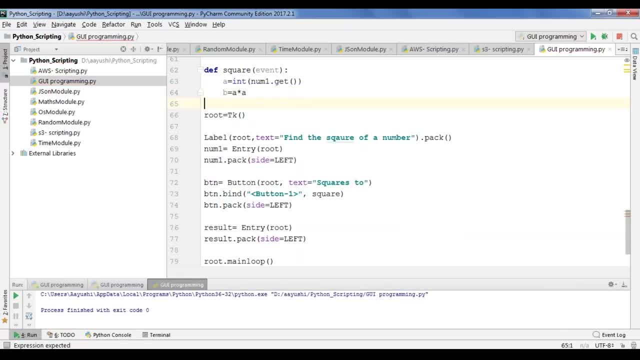 So I'll say a into a and stored in the B. then what I need? I want the result, which is a button over here. I want to display the result in this button, So I'll say result, dot insert, and I'll pass over 0 comma B. 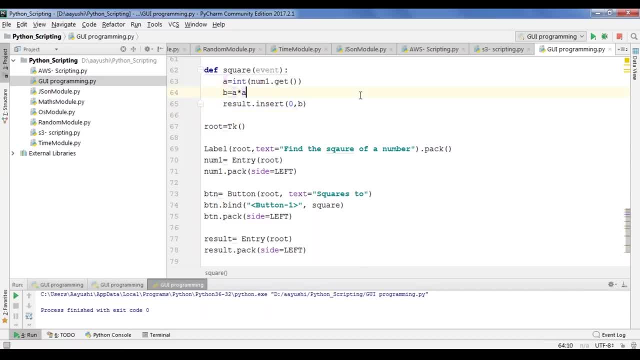 which is the square of the number. So now let me just run this and let's see whether this works or not. So now, as you can see, here I have the small GIA application, So now let me just enter the number, Let's say 2 squares to, so this gives me the result. as for similarly, 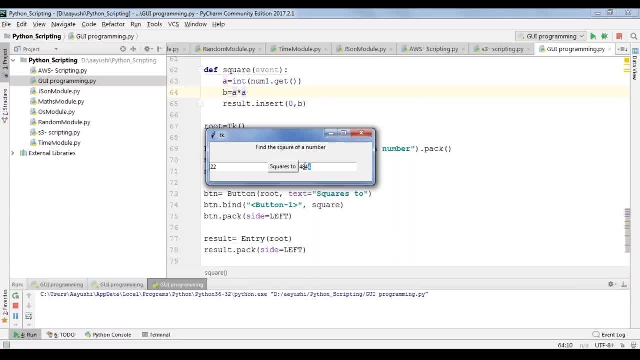 if I say 22 squares to, so it's just giving the output after that. So what I need to do, I'll just go over here. I'll just change a logic a bit. So I just need to delete the previous value. So I'd say result, dot, delete and say 0 and I'll say end. 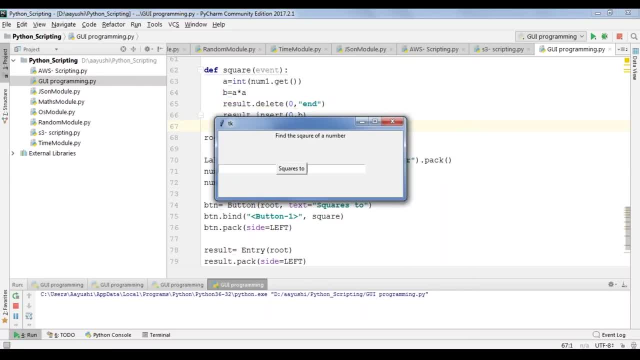 and now let me just run this. So now, if I say 2 squares to 2, then I say 22 squares to 484 and you can write similarly. you can write any number. So this is how we can perform various operations on this GIA application. 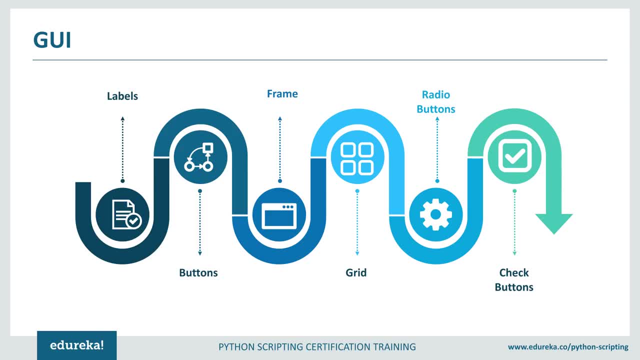 Well, now let me go back to my presentation. Let's see what else we're left with. So here we have implemented all these small components to create a basic GIA application. So let me summarize this session. So first of all, we have discussed how a scripting language 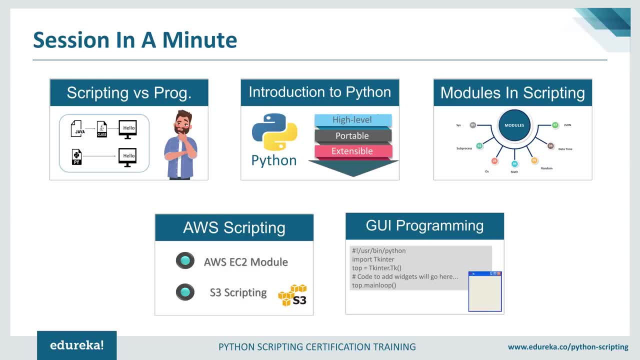 is different from a programming language. after that, I have introduced you to Python and various features. then we have covered the various modules in Python, which are sys, subprocess, OS, math, random date, time and JSON, and we have implemented some of them as well. Then they have talked about AWS scripting, wherein